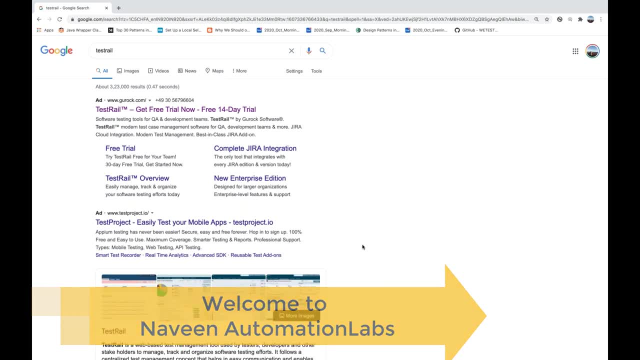 Hey guys, this is Naveen here. Welcome back to Naveen Automation Labs. Guys, today, in this particular video, we are going to talk about TestRail, which is a test management tool. You can do a lot of things over there, a lot of integration. You can integrate with your automation as well with Serenium. So in this particular video, we will be talking about how to set up TestRail, how to create your test cases, test cycle, text execution, a different type of integration and everything. We will be seeing that. So I'll be preparing only a couple of videos on that, But in most of the things we will be doing in the same video, only a lot of people will be seeing that. 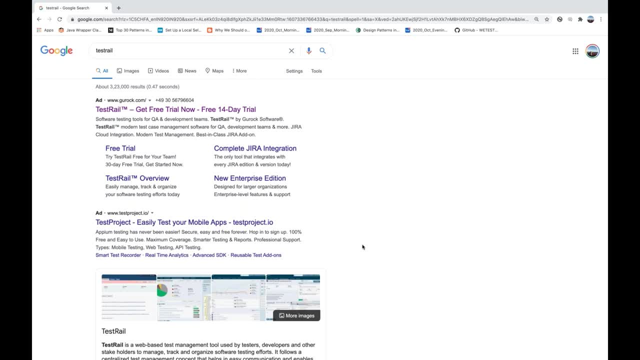 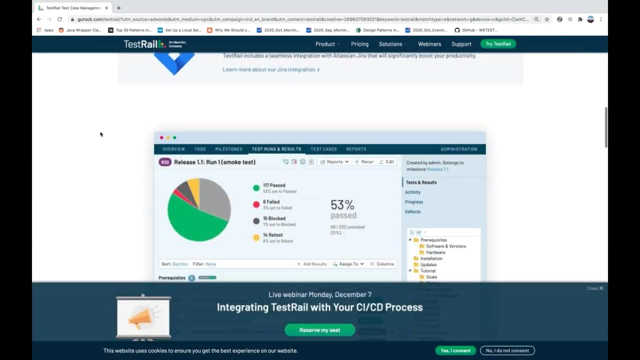 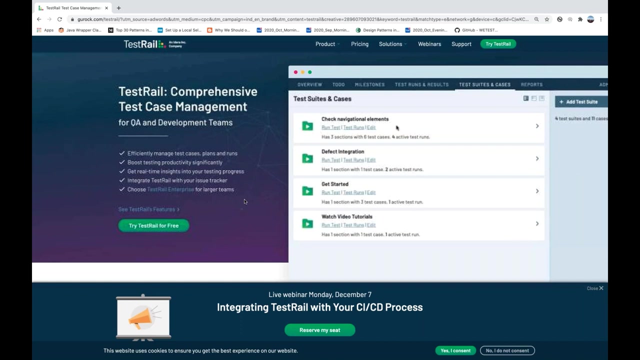 So if you are asking about Naveen, please prepare some video on TestRail. and then Zira tool is also available. we have for that. So TestRail is a pure test management tool, guys. So let's do one thing: that you simply go to this particular site, gurockcom, Here you can see this is the official website for the TestRail and it's clearly written that comprehensive test case management tool for QA and developing teams For 14 days. you will be getting the 14 days free. You can use that and you simply click on TestRail for free. 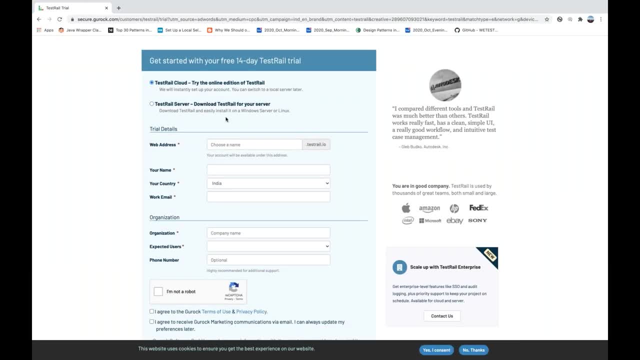 What do you just need to do? that You have to create an account initially, So you can download TestRail for your server as well as, let's say, you're maintaining one typical machine for that, a dedicated machine for that You can download, and then you can start the server and the entire team or your organization will be using this particular server. Or you can simply directly go to their cloud- TestRail cloud- and that is online edition for the TestRail. You can prefer this particular option also. I would advise you to go with this option and then here you 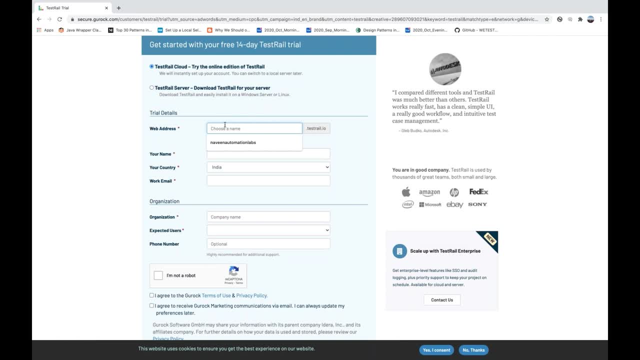 have to give your different details over here. So let's say, I'm writing some different details over here. I'm writing Naveen Automation Labs, whatever. Okay, let's see. tomorrow you're joining Amazon or Uber, So you will be writing. the URL will be created like this: Let's see: amazontestrailio. 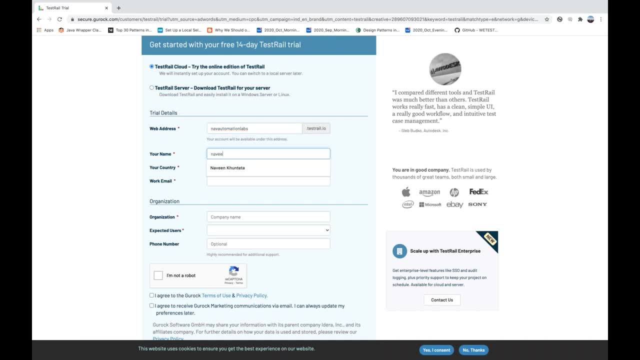 like that. Okay, and then I'm going to enter my name over here. Let's say I'm entering Naveen and country is India. I'm entering some email ID over here. Let's see this Naveen animation 20 at gmailcom. and then I'm 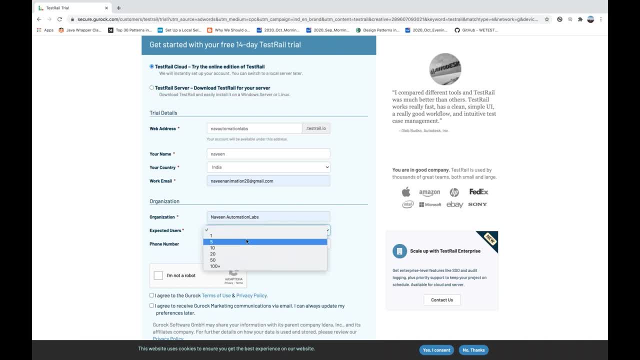 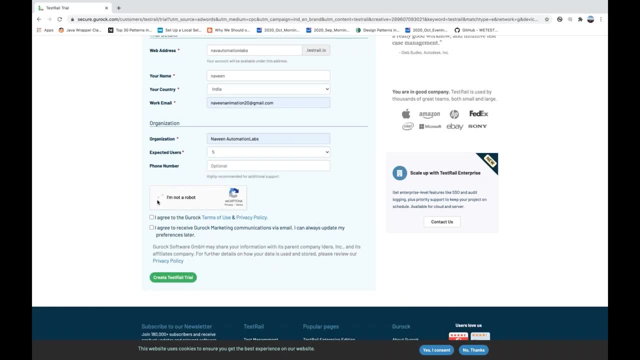 entering. Let's see. My company name is Naveen Automation Labs. How many users you expect? So let's see: I'm expecting around five users. Phone number is optional. You can ignore that I'm not a robot and click on this. Click on this Agree. accept the license agreement. 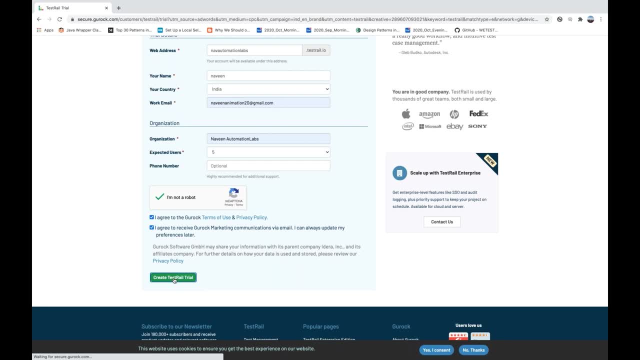 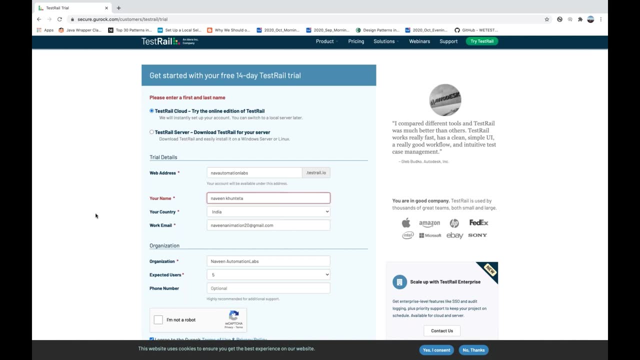 terms, conditions and everything and click on create test trial. When you see this that it's saying: please enter a first and last name. So let's enter a first name, last name over here and, I think, Selected once again- and then click on it. 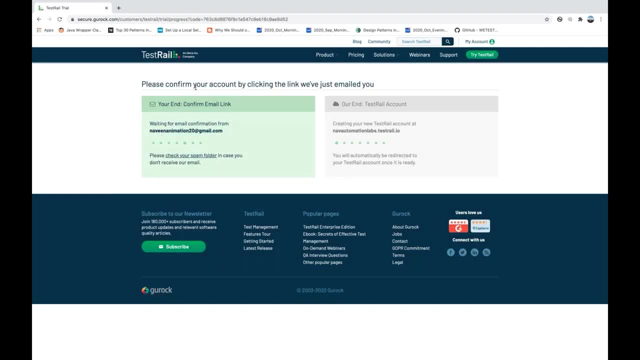 Ah, I see Okay, here I go. Ah, I see Okay, and then click on all your testers. OK, that's it. Yeah, so let's go ahead and read TEST RAIL. Let's see here. Her question is: is this correct? 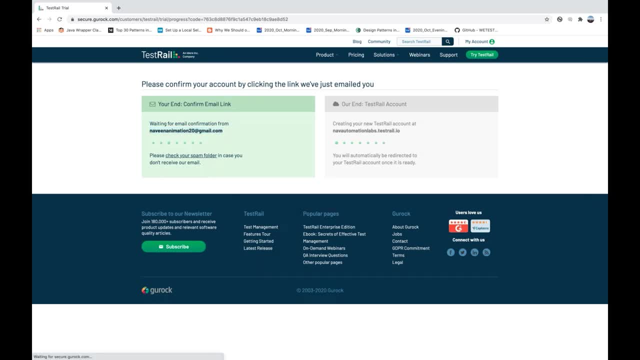 Yeah, So, yeah, So let's do another test against our website: test rail. Yeah, so you can see that. Okay, Yeah, so already one email has been sent to this particular email ID, and then you have to confirm the email ID. 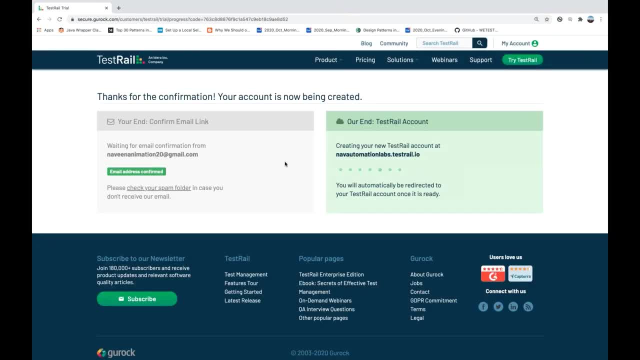 It will give you one confirmation link over there and then you have to confirm. So yeah, you see, that email address has been confirmed, You can see that and that's it. And after that it's saying that from there and test your account. it's creating a new. 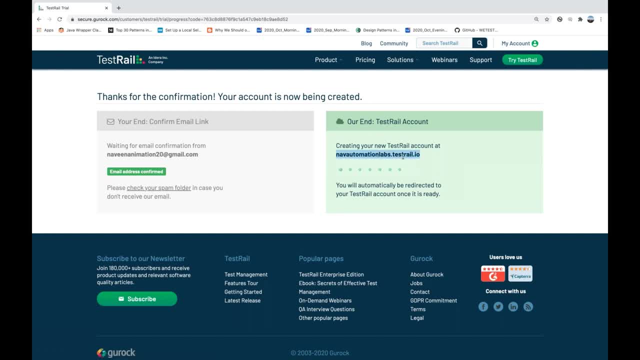 personal account for this particular laps test realio, and it will automatically be. they redirect you to test your account once it is ready. so let's wait for some time. it takes a couple of minutes to set up account and once it is done- yeah, so it is done- you can write your. 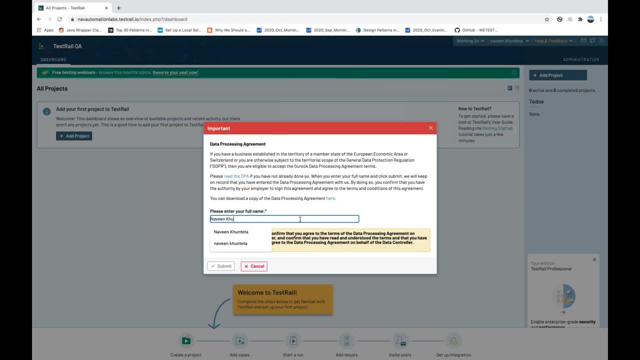 name over here, so that's my name, full name. i'm writing naveen kodita like this, and then select this particular checkbox to confirm the agree and license and terms and everything, and then click on submit. when you click on submit, you see that okay, yeah, data processing agreement successfully done. 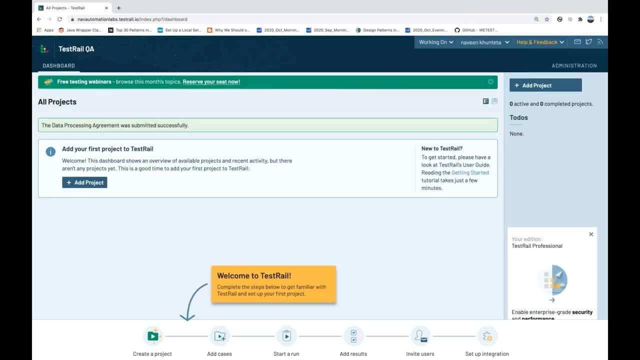 and that's it. and immediately after that, this is the welcome screen, or you can say this is the dashboard screen. you have to create multiple projects over here, guys, so first we need to understand that, especially this particular video for people who really wants to learn a test. 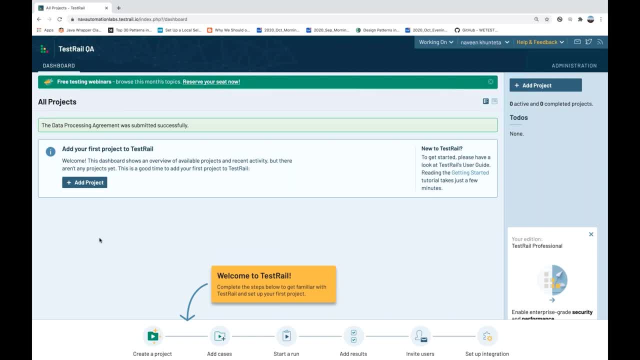 management tool. second thing is that if you have not any experience in test automation or in testing field or in manual testing, it will help you a lot, because this is what in real-time projects we do: that where exactly you want to write your test cases, how to create a test suite test plan, how to create a test cycle and what are the different. 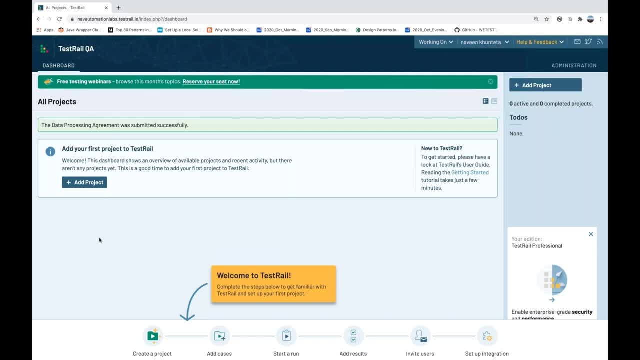 regression cycle, smoke sanity cycle or feature-based cycle. we can create that. so these things you will be learning in this particular video, so very beneficial- and similar kind of tools we have available in the form of zeta also. we have the fire plug-in over there, but this is. 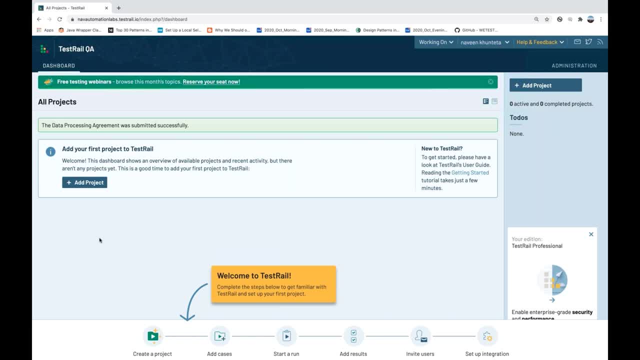 also one really good tool: test strain. it's not open source but you have to pay for it, but a lot of companies they started using this particular tool and for their test management activities. you can use it for a lot of different things. so immediately after that, when we land on this, 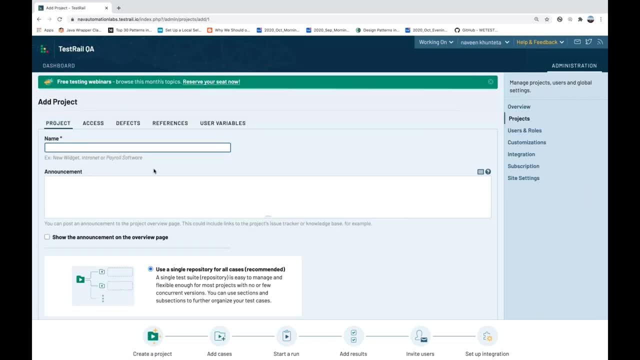 particular page, we have to click on project, we have to add a project over here and let's add one project over here. so, whatever the project name, let's say I'm simple writing. my project name is. let's say I'm writing for Amazon. okay, just take any example: if I'm writing for Amazon and Amazon. 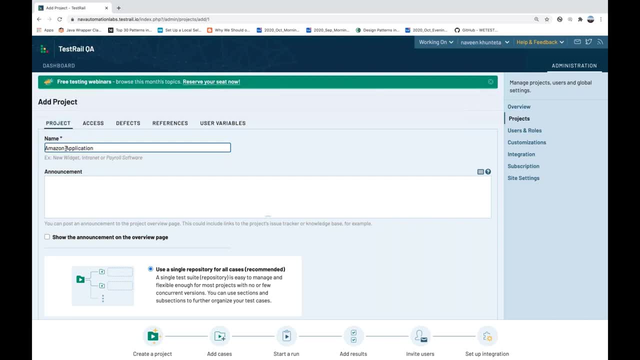 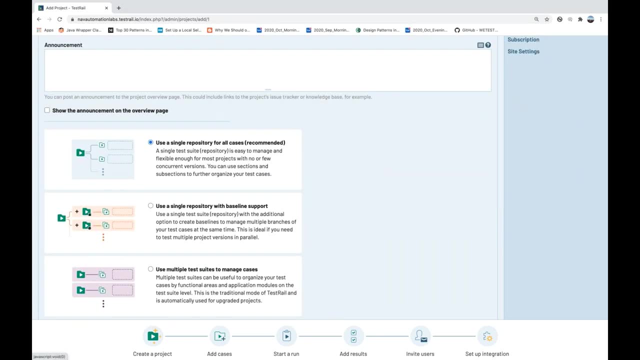 application. something like this: I'm writing it and you can write some announcement. if you want to do that, this is an optional thing. and then what exactly? they say that, okay, there are three types of project. you can create a project, use a single repository for all the test cases. 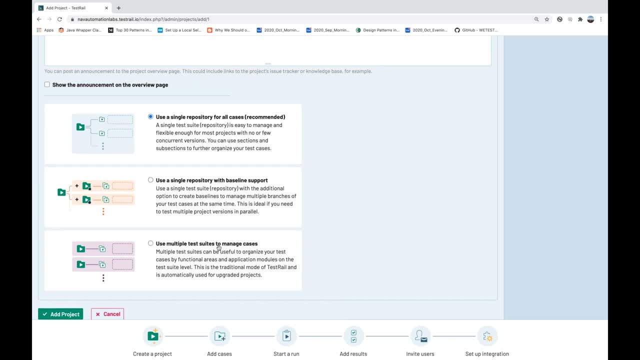 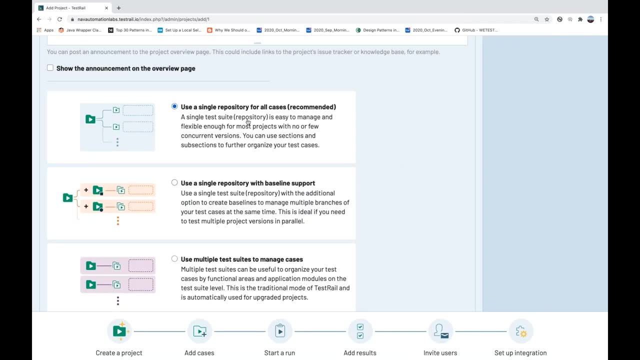 use a single repository with the baseline support and use multiple test suite to manage test cases. all three options are having the unique one, it's first option saying that, okay, a single test suite repository is easy to manage and flexible, so only one single repository test repository will be created for most of the projects, with no 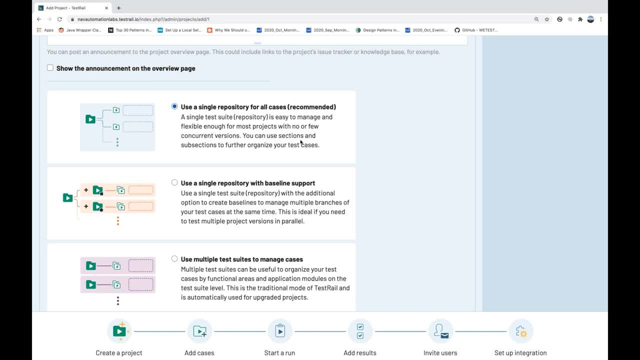 designer or few concurrent versions, you will be getting it. you can use sections and subsections to further organize your test cases. so this is a recommended one. you can use that from the single project you can create on the single repository you can create a single test suite over. 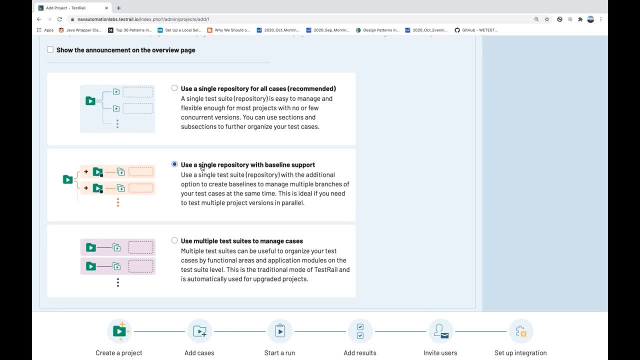 there and you can execute directly from there. second option is that use a single repository with baseline support, with additional option to create baseline to manage multiple branches of your test cases at the same time. this is the ideal if you need to test more of the project multiple project version in parallel. so let's see some companies. what happens that? uh, you have. 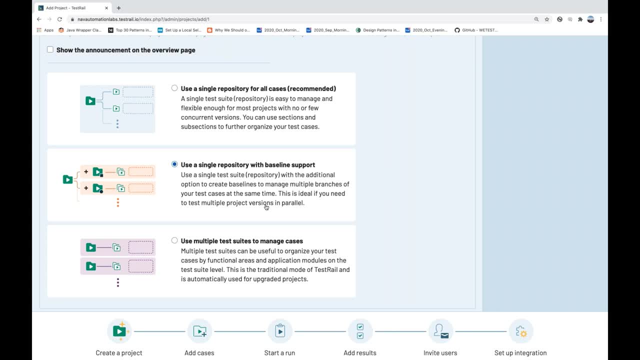 multiple projects and uh, or let's see one single project having multiple versions you want to execute. let's see something is running on some different uh platform and different versions. something is running on a different platform with the different versions. in that case, you can prefer this. i would advise you to use a third one. use multiple test suites to manage different test. 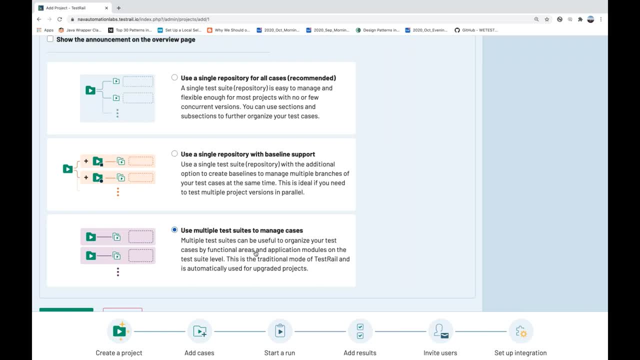 cases can be useful to organize your test cases by functional areas and application modules. let's say i want to execute only a user management test cases or order management test cases or log in related test cases. i would divide into that particular area and okay, on the basis of. 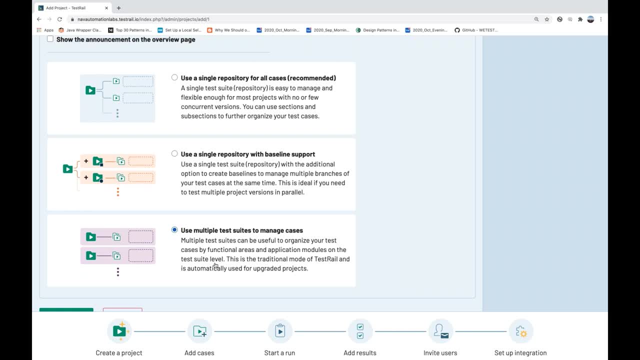 different modules at the test suite level and then i can execute and i can separate it differently. this is the traditional mode of test. rail is automatically used for upgraded projects, so let's use this particular option and then click on add project. when you click on add project, you 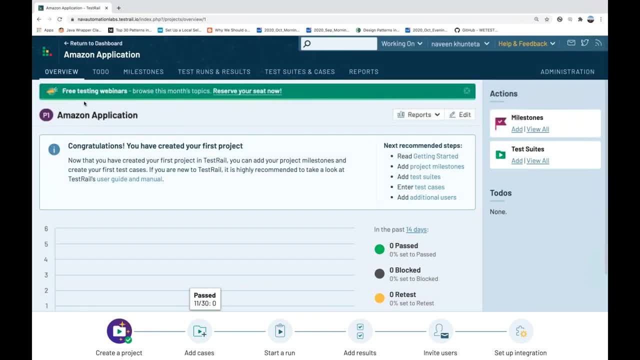 see that? okay, yeah, this amazon application got created over here. this is a. this is the project that i want to execute, and then i can execute and i can separate it differently. this is the project name and this is the first project that we have created over here. 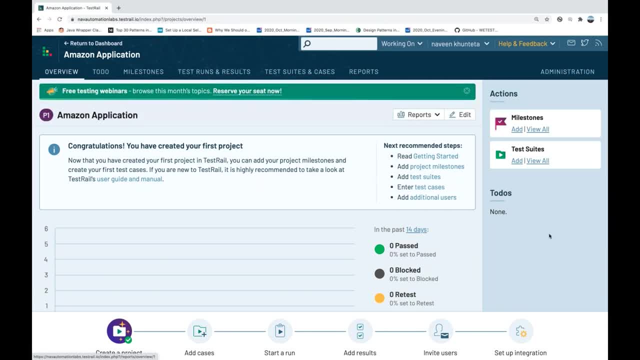 then what do we have to do that? after that you have to create the test suites over here. so i first go to a test suite over here. you can add it, but before that you can see that, yeah, this is a to-do. if you have any to-do notes or something like this, you can add that. you can add some milestone. 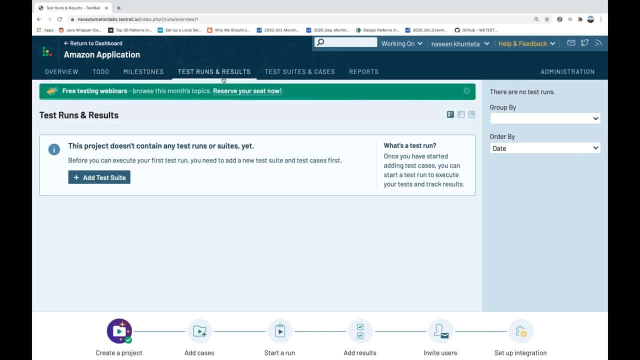 we will talk about milestone later. this is the most important section: test runs and test results and test suites and cases. you can check it over here. you can see the result over here. you can execute the result from this particular tab. i mean you can execute your test cases from this. 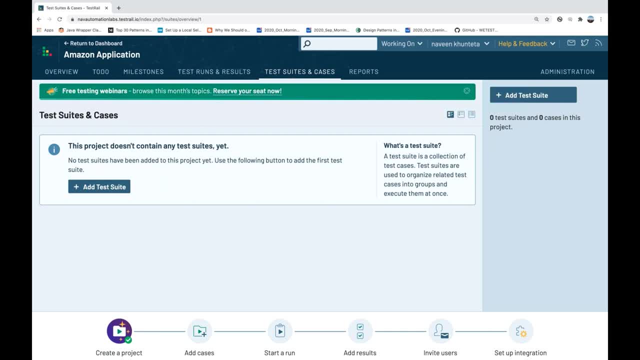 particular tab and then test suite and cases- you can see it over here- and then different types of report also. you can generate then what you can see that. okay, yeah, this is your account settings. you can check your settings over here: your email id, language preferences, time zone, different things. 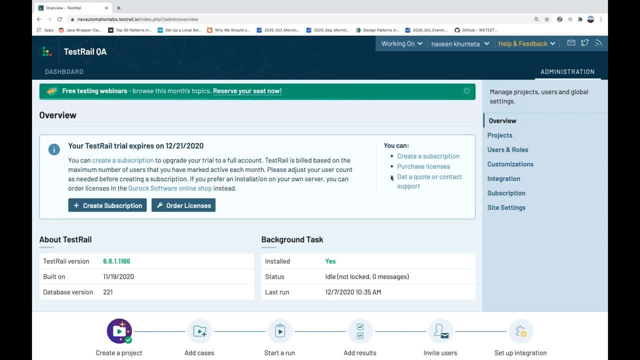 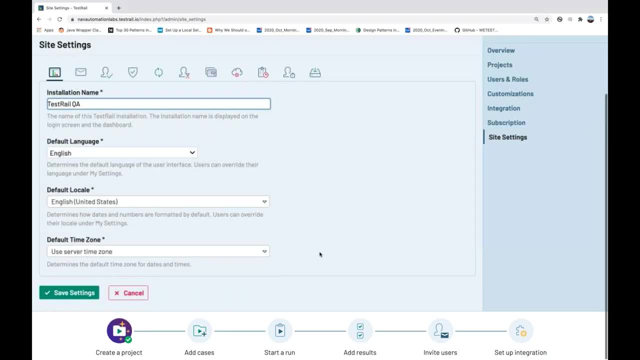 you can do that. and then we have administration sections also, where are different types of settings: site settings. let's see if you want to integrate with the uh with some other tool. let's see selenium or some any automation tool. they expose different apis and everything they do that. 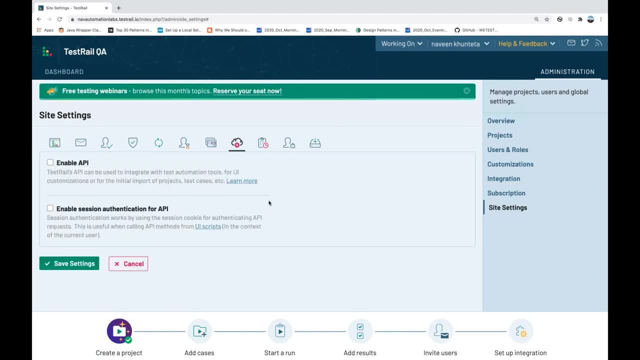 see you click on enable api. they will give you certain api. you can create their authentication api and and username password and the token you can create so that you can send whenever any test is getting failed from selenium, automatically it will be updated over here. so those things maybe we. 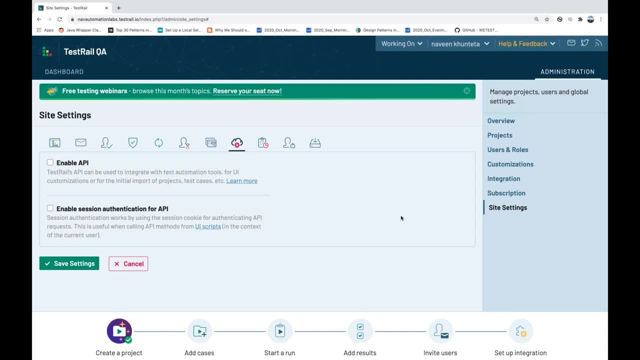 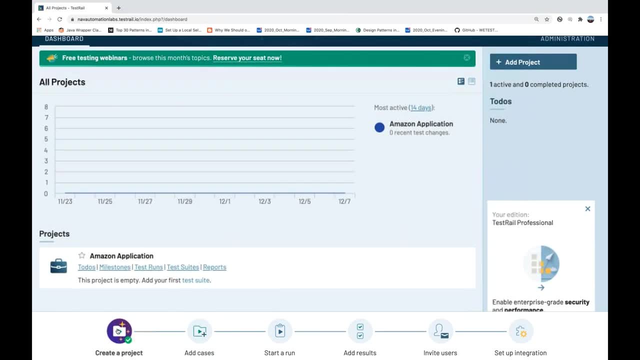 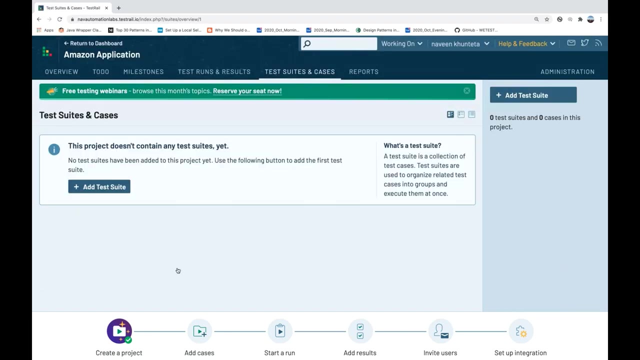 can do it later in some upcoming videos, but uh, quickly, let's see. i'll go to the dashboard once again. it's a very simple uh project guys, it's already added project. we have already created amazon application. now i am going to let's see on test suites over here. when you go to test suites, click on add a test suite over here and let's see. 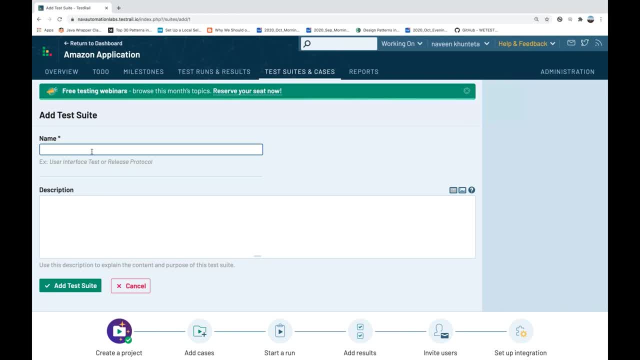 i'm giving a name, what is the name of the test suite. so let's see in amazon there is a application or there is a section. let's see login page. so i'm going to write some login page. i simply write login page or i would try: this is amazon login page. this is my suite name, right, and 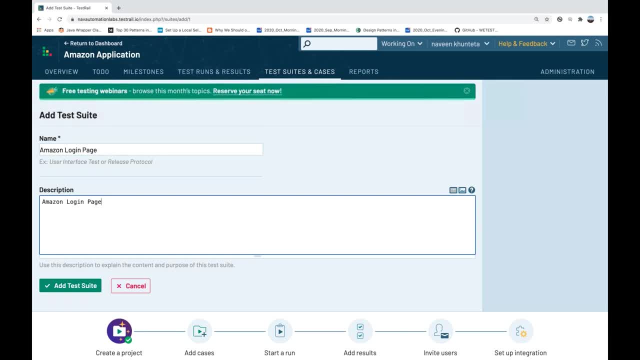 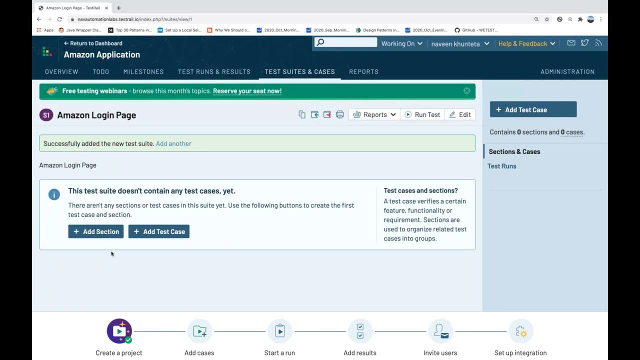 same thing. let's: in the description i'm writing it you can write some proper description. click on add a test suite over here. when you add the test suite, you can add multiple sections. also. let's see in the login page you have different sections. let's see: forgot password, reset password, a typical. 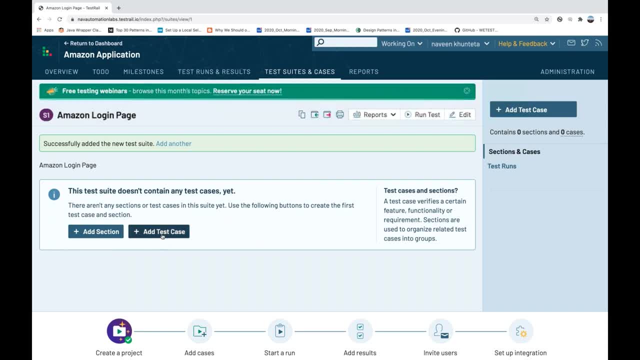 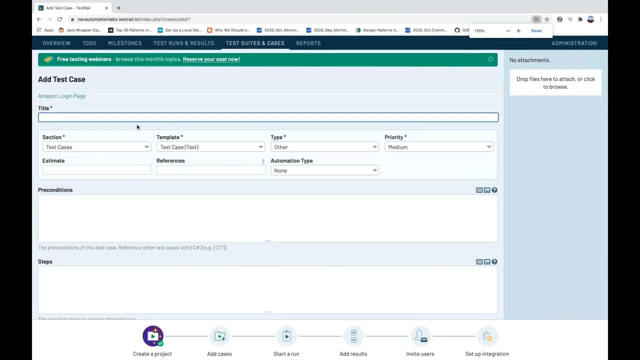 login such things also. you can do that, or you can directly start writing the test cases over here. so simple click on add test case over here and then, let's see, i'm going to write my first test here, my first test i'm going to write. let's see something i'm writing. uh, let's see. 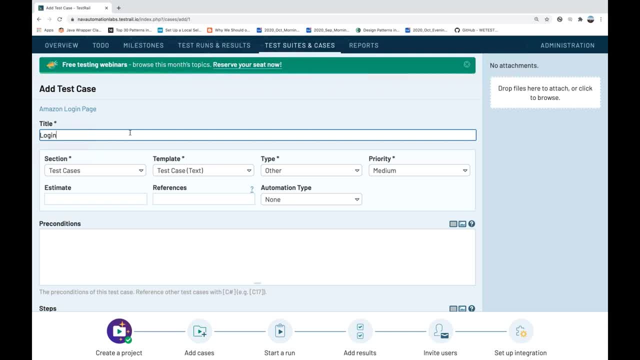 this is login, so i simply write: uh, my first test is that user is able to okay login into amazon application. this is a test case, yes, so yeah, you can see that. okay, yeah, this is my test case. and then they provide two different type of template sites, especially test cases, and 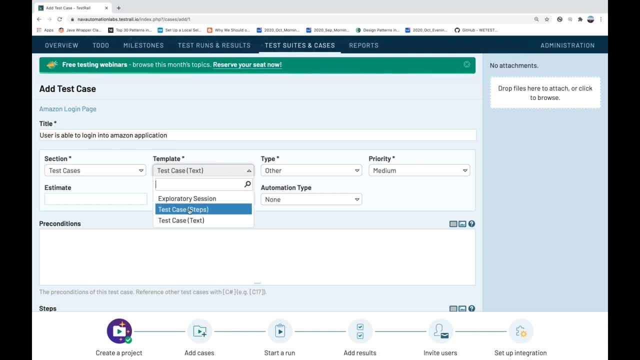 test cases in the form of text and one is test cases in the form of steps over here. so you must write your test cases in the form of test cases, in the form of test cases. okay, when we write the test cases in excel file, we have to write in the form of test cases with the help of text, and then 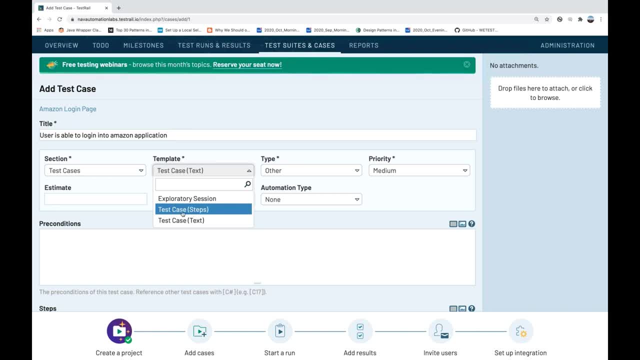 for every step also, you can write your expected result and the actual result and when you run your test cases, every step wise, also, you can execute that. so these are the generally two, a major, uh, a template we follow to write your test cases. so let's see, i'm picking the test cases, step over. 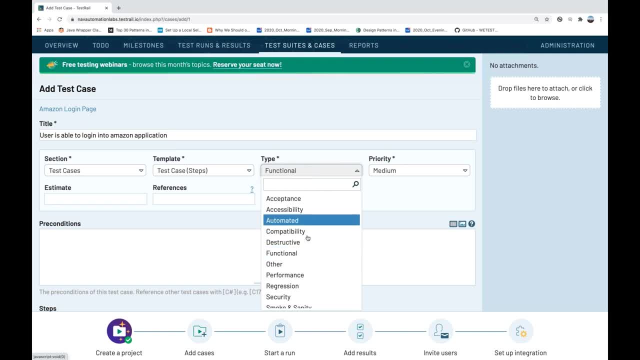 here, right, and what is? it's a functional type test. i'm writing and there are different options. are there performance, regression, security, like that? so let's see, this is my functional test case. what is the priority? priority is high over here. and then what is the pre-condition? so i simply say that user. 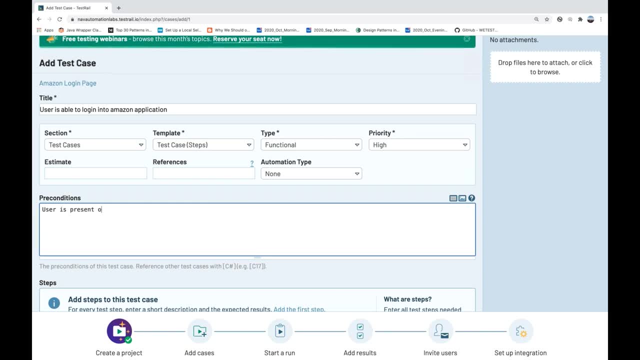 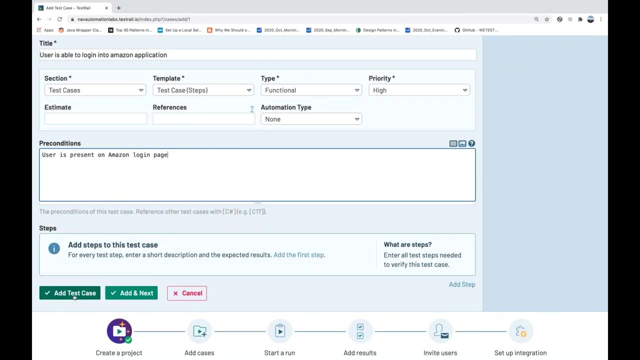 is okay. user is present on amazon login page. this is the pre-condition that we have written. and let's see simple: we have to add your test cases over here. so it says that: add your first step. you can write the step and what exactly you are expecting. so this is my first step, that okay. 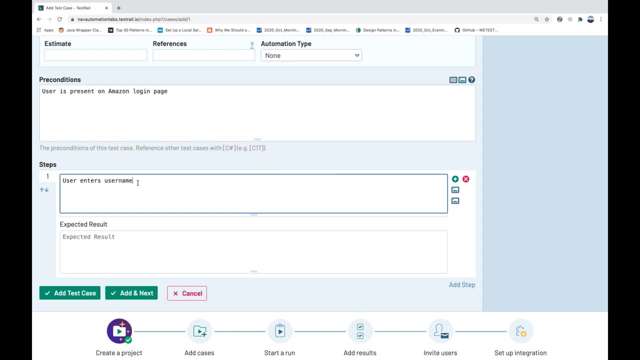 let's see: user enters username and what exactly you are expecting. so i simply write: user should be able to enter username, simple. so let's see. this is where the simplest step that we have written. so simply click on add, step over here and then the next step you can write. let's see. i simply write. 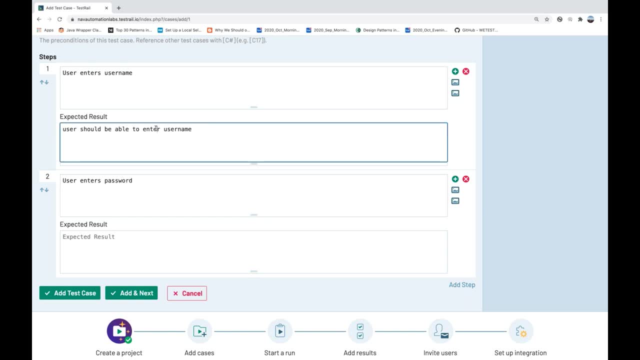 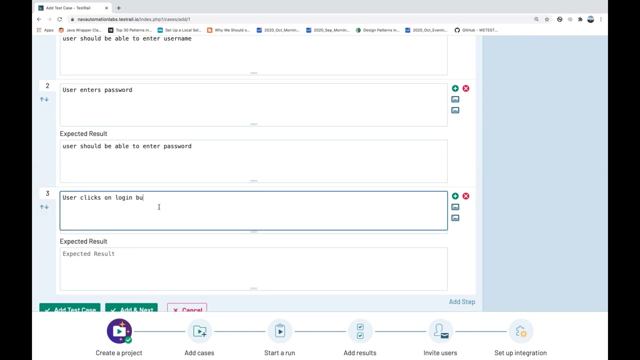 write it over here. user enters password. so each and every step you can write it like this and I simply say that, okay, user should be able to enter a password over here. and then I simply say that, okay, last step is that user clicks on let's see login button and I simple say that user should. 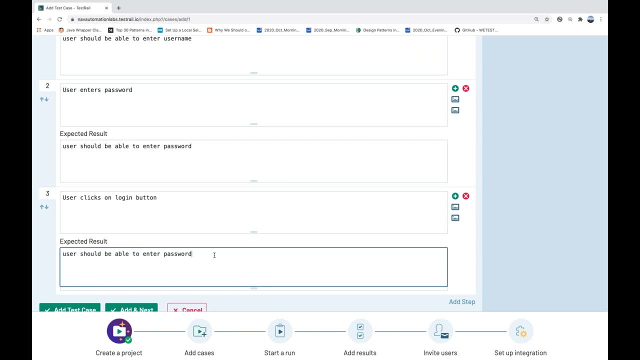 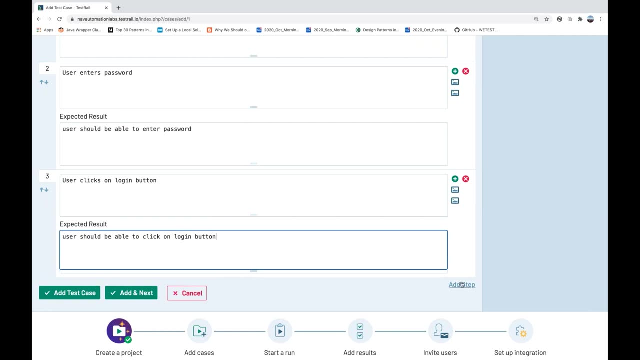 be able to click on login button. so should be able to. I'll write it over here: login button. and let's see- this is the test case that we have written. and let's see- I'm adding one more step over here- that when we click on login button and then the 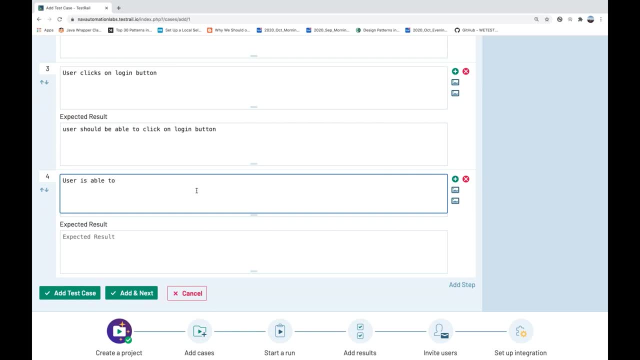 last step is that user is able to log into the application. an expected result is that user should be able to log in. I'll write some more expected result over here: that user should be able to see the home page and let's see, user should be able to. 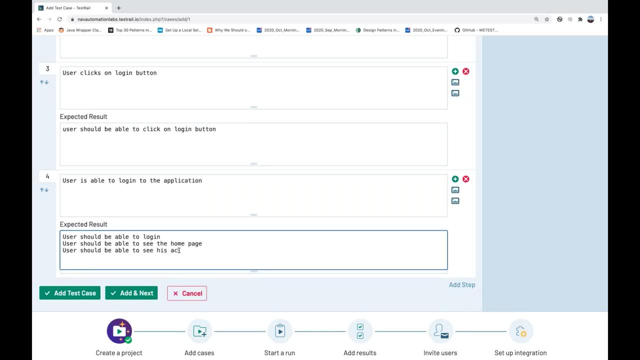 see right his account. uh, details like that. oh, let's see. user should be able to see a message over here. what is the message? the message is that a welcome username, whatever the username that you are passing, right, okay, so likewise you can do that. another thing is that guys. 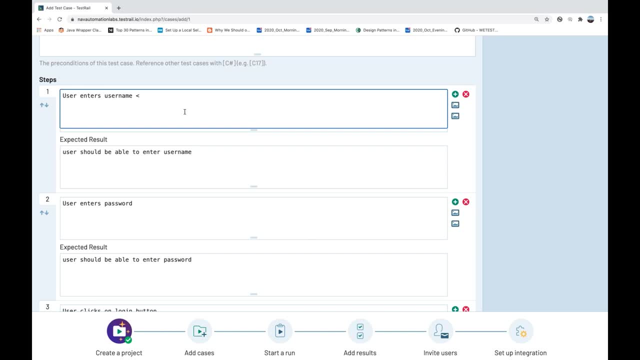 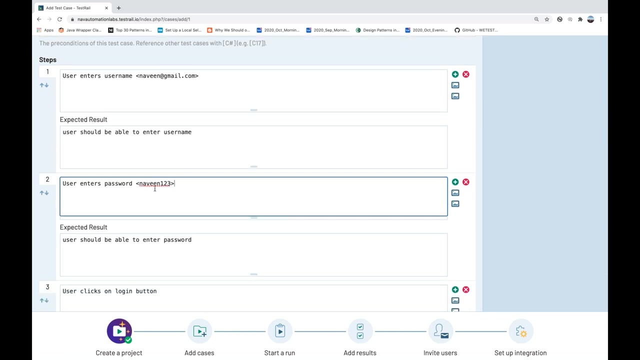 if you really want to enter a step along with the data, what is the username you want to write? so let's say Naveen at the rate gmailcom. I can write my username and then I can write my password over here. that let's see. my password is Naveen123. there's my password. so in anchor brackets within: 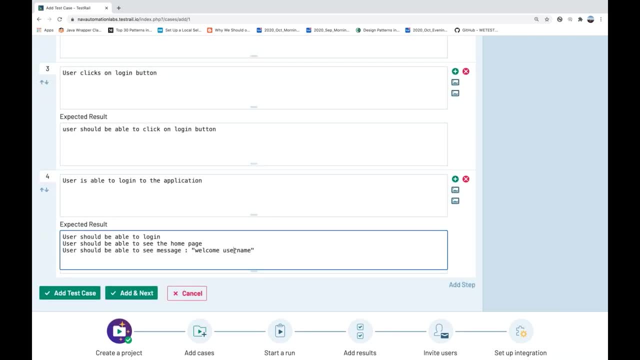 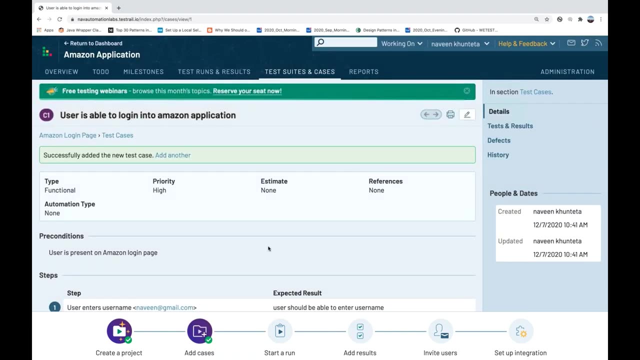 these two brackets. you can write it and then user should be able to do that and the I simple write welcome Naveen over here and simple add this entire test. so what do you see? this, this entire test. you can see over here that user is able to log it into Amazon application. this is the title of the page. 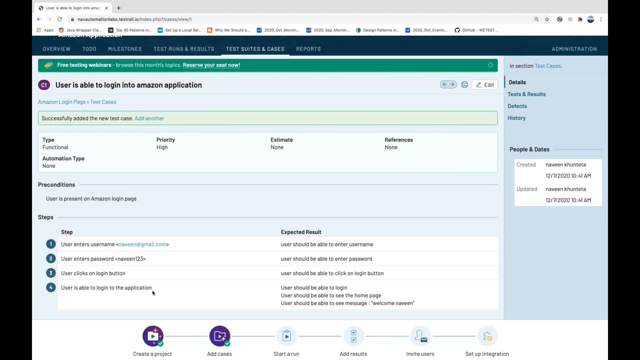 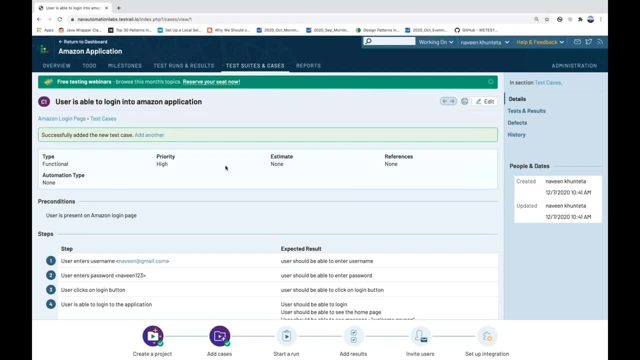 title of the test case and having these four steps are available and these are the different attributes and the metadata over here. so let's add some one more test case over here. so how will you add another test so you can do one thing? what again you can do simple test, suite and cases. you 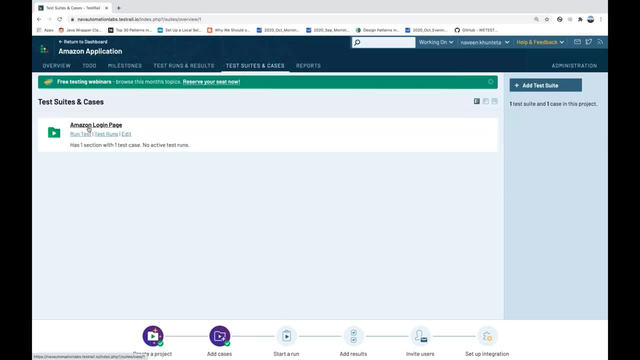 can see that Amazon login page and you just click on it. you will see that c1. c1 means this is the case ID. this is my test case ID got created over here and this is the title that you're going to use. we have already created and, let's say, i want to add some more test cases for the amazon login page. 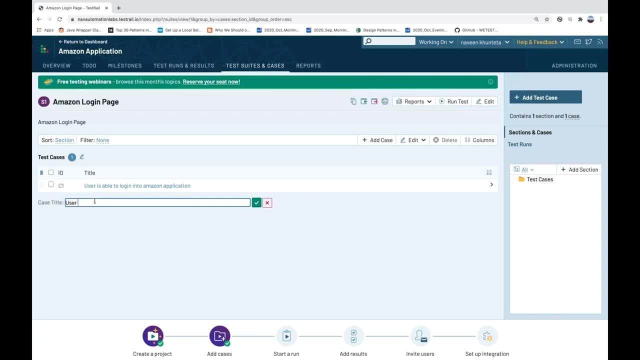 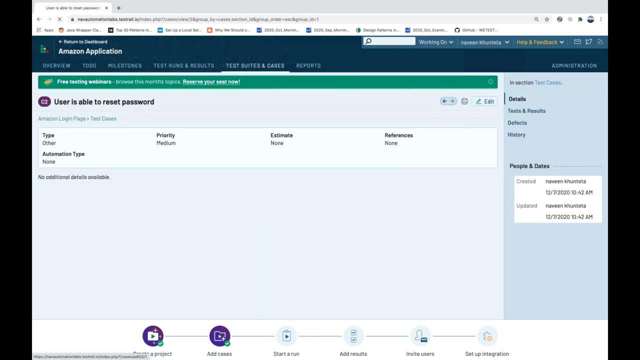 i simply click on this and the case title is: i simply say that quickly. i'm writing: let's see, user is able to reset password, right? so this is the second test i have written. you click on this particular second test and then you click on add it over here. when you click on: 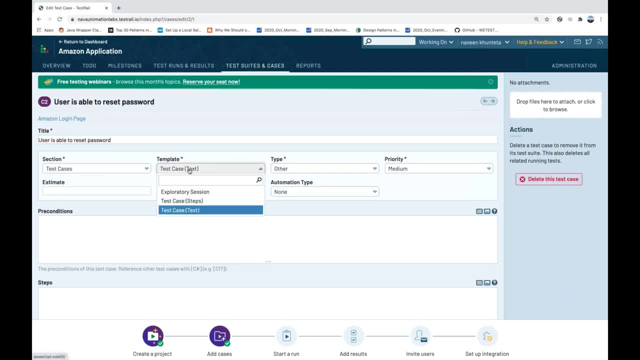 added again. the section is test case. now this time let's see in my previous section what we have done in the previous test case. we have written test case stepwise. let's write test case with text wise. i don't want to follow each and every step over there. let's see. i want to. 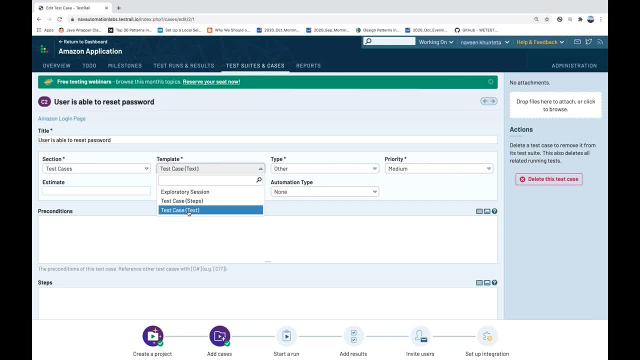 follow. i want to write all the steps in the simple text over here, not in the form of different steps, so click on this. what type of test case it is. this is functional test case and the reset password is also high and let's see- or maybe i would say, critical user should be able to reset the password. 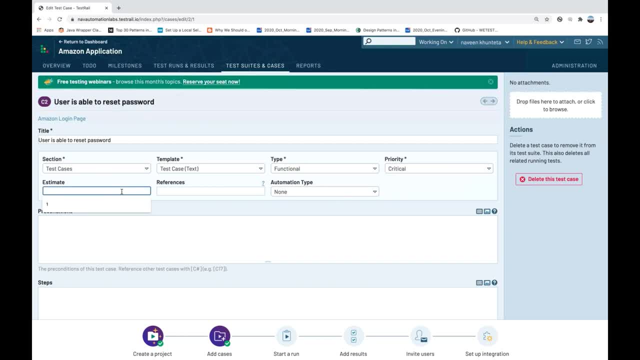 like that and estimate you want to give. let's say i want to give that okay. yeah, let's see something and i'm giving over here. you can say that, okay, maybe it could be 10 minutes or whatever. how much time it took. so let's say it's taking around two minutes of time to execute that. 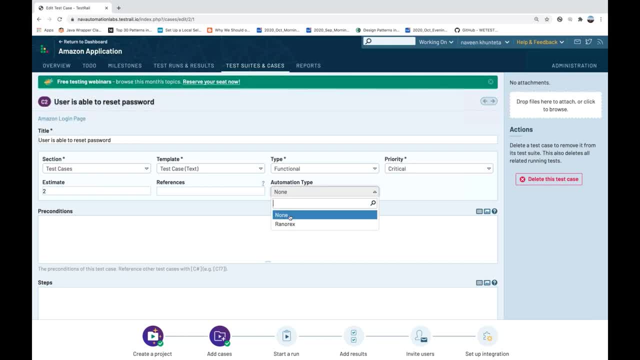 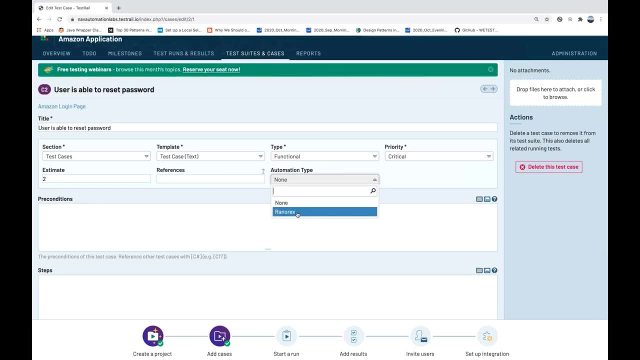 and or to write this particular test case automation type: right now it's none. later on we can configure when we integrate with some other folks, so you will see more options over here. that, yeah, automation type with a runner: x, selenium or whatever. so let it be none over here. 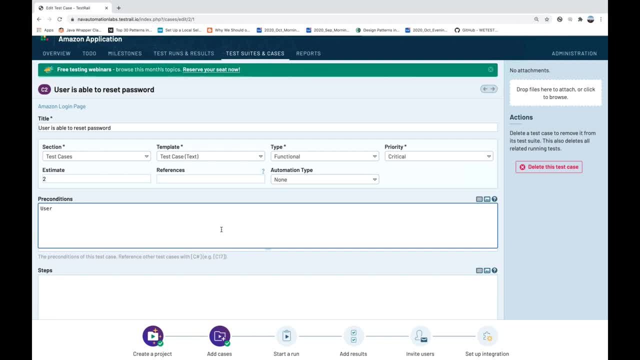 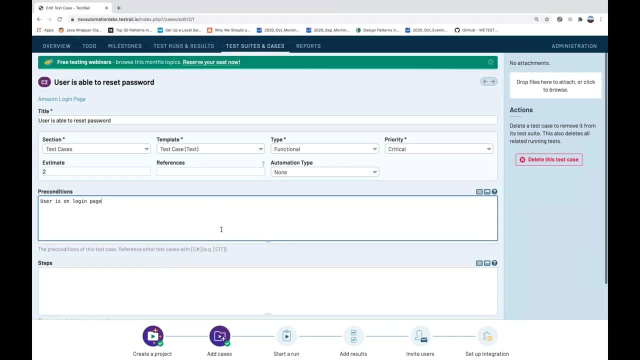 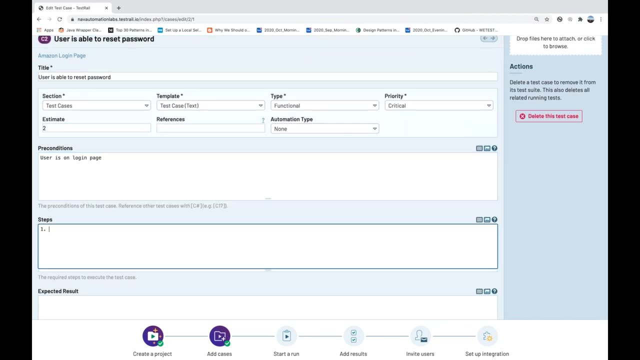 now what are the pretty conditions? so pre-condition is that user right is on a login page. this is a pre-condition user in the login page and then we have to reset the password. so what are the different steps? you want to write my first step. i can write it over here like this: 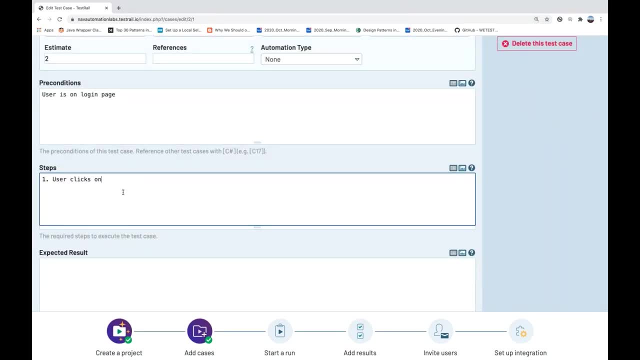 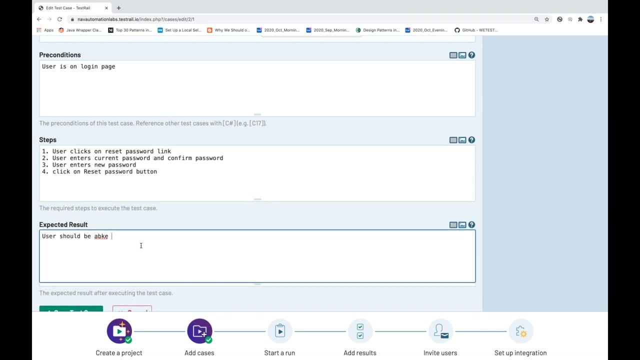 my first step is that user clicks on: let's see a reset password link. second thing is that user enters something. let's see: uh, i want to change my password, right, current password affecting. so my expectation is that user should be able to and i simply write a user should be. 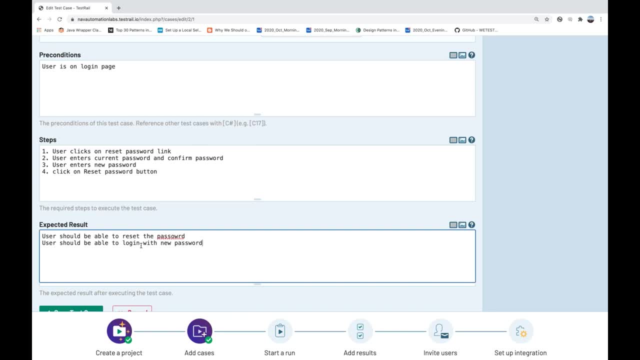 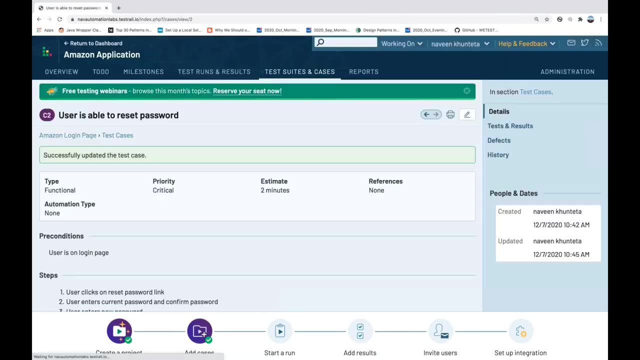 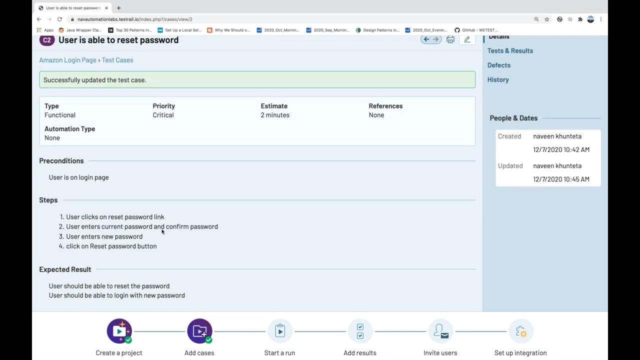 able to log in with new password, whatever the password that we have changed, right password- and then click on save test case. so yeah, so this is the second test having all these steps. so these are typical, if you remember excel sheet format that generally we use, that this is my pre-condition. these are: 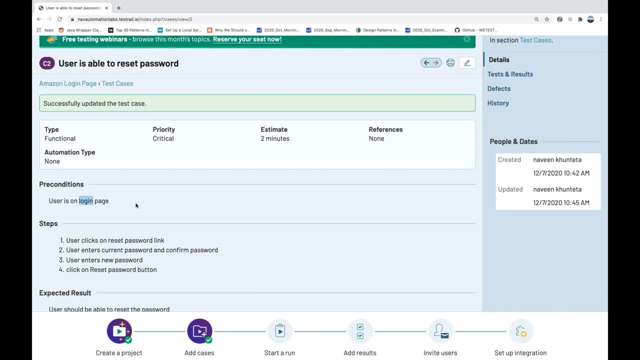 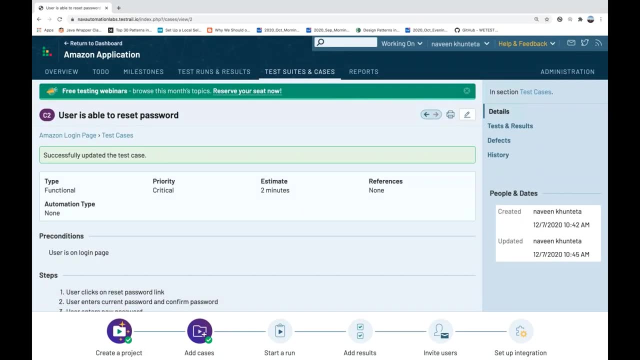 the attributes and this is my test case. i uh title over here and then these are my expected result and this is the steps to reproduce. you can check it over here. created by. updated by navin time and date. everything is coming over here like that. i'll go to my test tweet in cases. 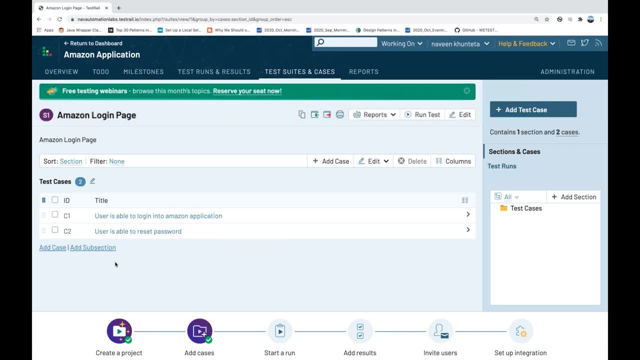 once again. this is the amazon login page. here you will see two test cases got created. this test case got created on the basis of their steps. second test is created on the basis of the simple text over there in the form of a step to reproduce. okay, now let's see. i want to execute my test cases, so i simply go to test run section over here. 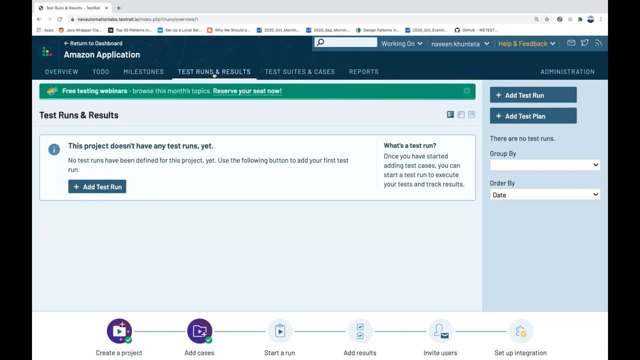 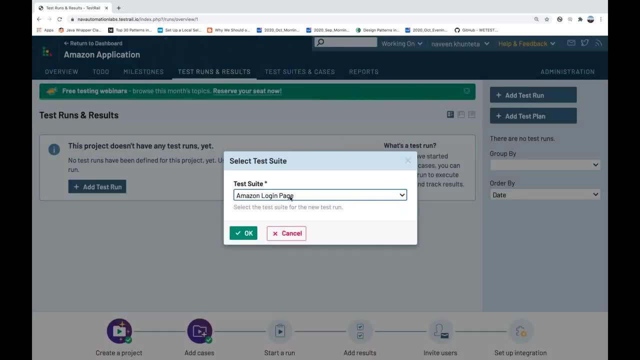 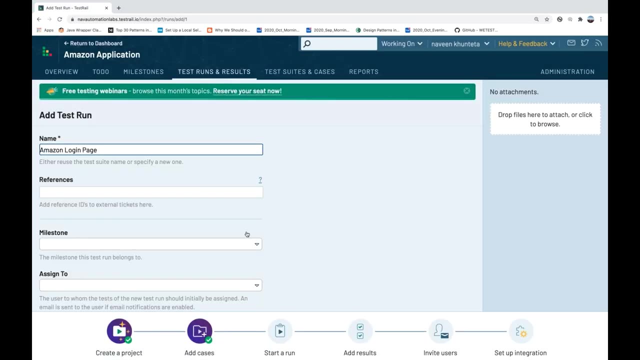 does test runs and results. so simply go over here and, uh, click on add your test run. so i just simply click on add test run over here. and what is the test suite name? so i can select the test suite name is amazon login page that we have created and click on: ok, similar kind of stuff. we do it in. 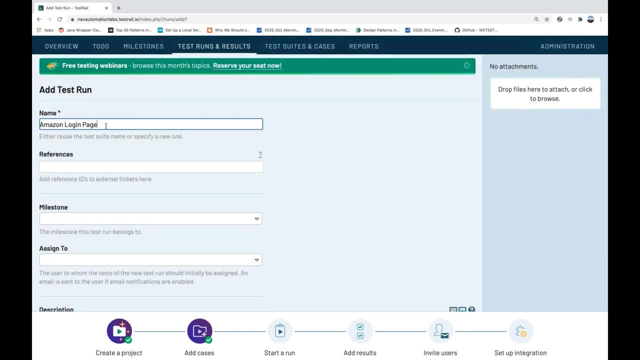 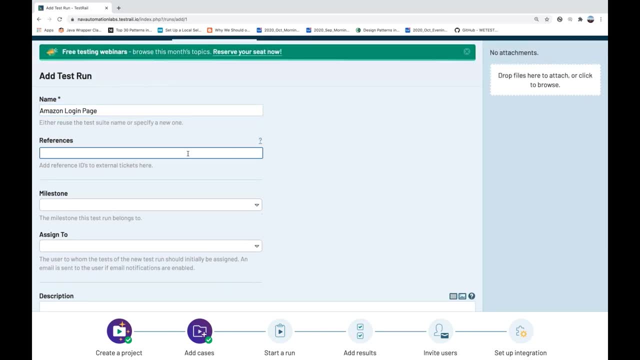 zira also, and this is the name of the test run. you can again edit it. if you really want to give a specific name, uh, references, any- let's see some zeta reference or any user story reference you want to give, you can give that. right now we don't have any milestone. we will talk about milestone. 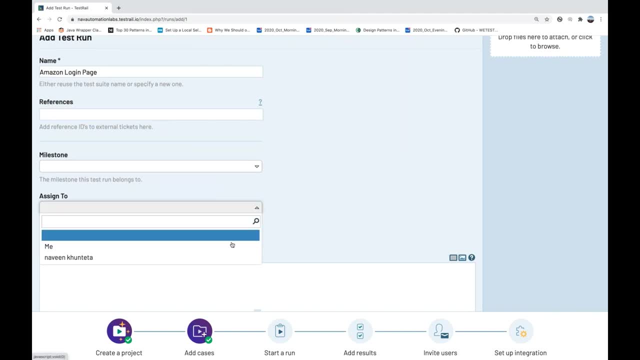 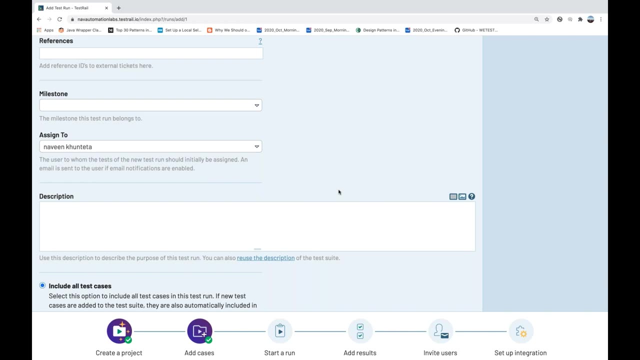 later. if you really want to assign that, okay, let's see, i'm the manager. i want to assign to naveen. so naveen will be getting a notification to execute, uh, these test cases. and let's see, you want to distribute your test cases to different people or different qa members in your team? that? 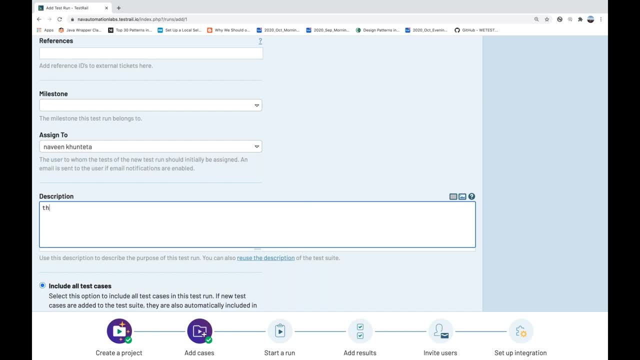 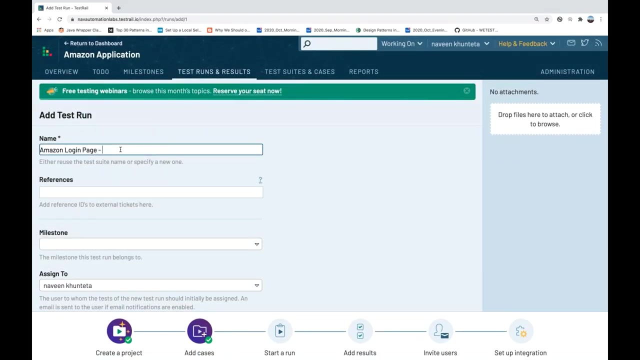 also you can do that. what is the description for that? so let's say simple: write this a test, run a cycle for a regression for, let's see, build number. we got the build number 1.0 and similarly i'll be writing amazon login page: this is my regression cycle because at the time 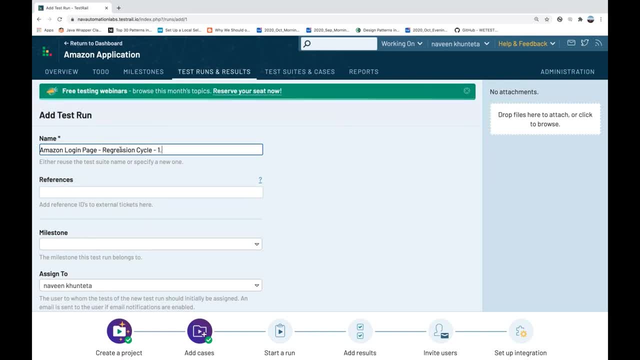 of. let's see the regression. i'm running this particular test case and my regression cycle is 1.0. later on let's see after 15 days again. you want to do a regression 2.0, 3.0, like that. you can bump up the version. 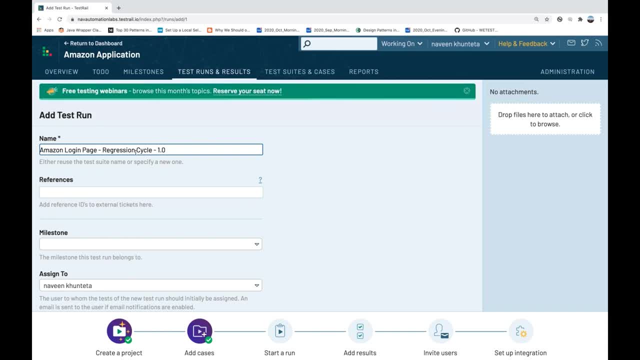 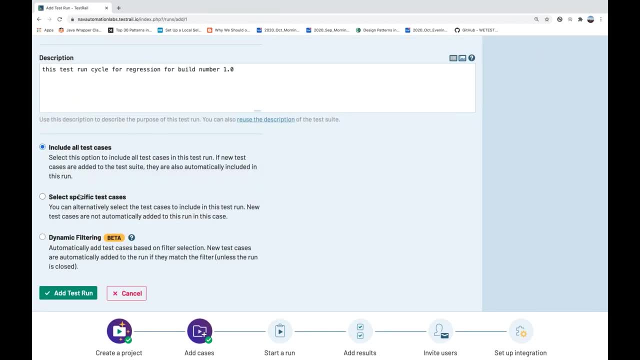 and you can create your own cycle over here. so i would say regression cycle or you can say regression test cycle. whatever the name you want to give, you can give that and include all the test cases, specific test cases or dynamic filtering we can talk about. you can check it later. 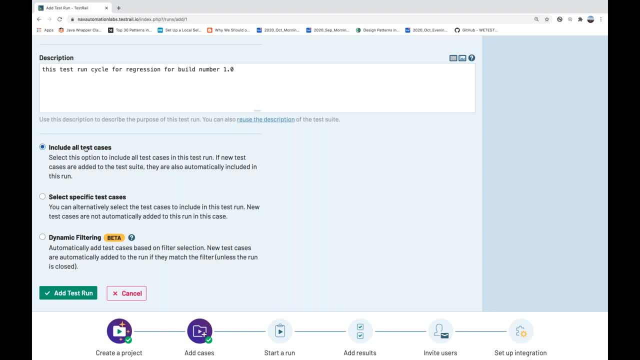 but let's say i want to include whatever test cases that we have written. i want to import all the test cases in this particular cycle because i want to execute all the test cases and then click on add test run. can you see that? okay, yeah, successfully, uh, added the test run. 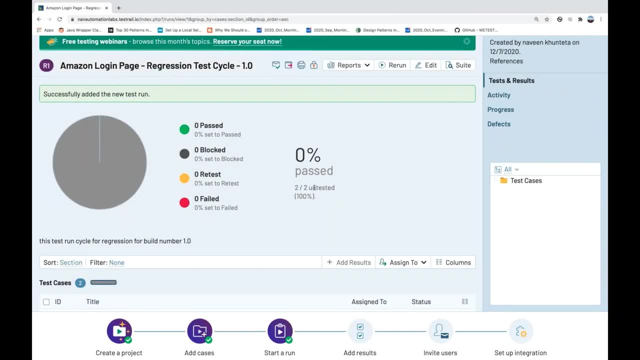 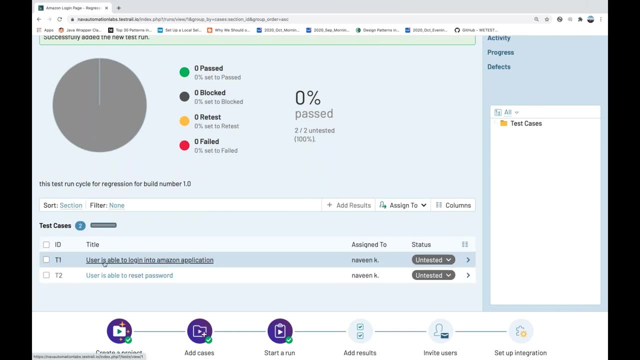 right now we have zero percent result because we haven't executed. it's saying untested, over here. now i want to execute my test cases. so what i'm going to do, that let's see. i want to execute my first test, so click on this particular link over here, the title of the page, so title of the case. you come over here and you see that, okay. 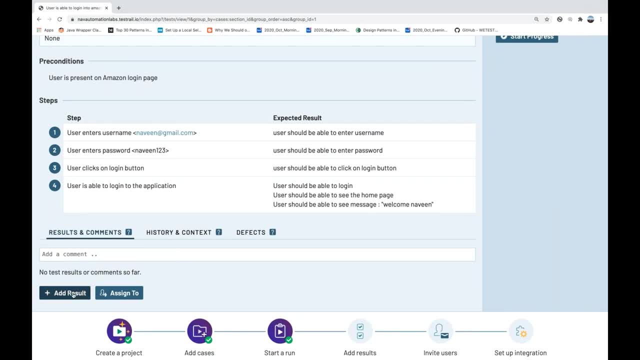 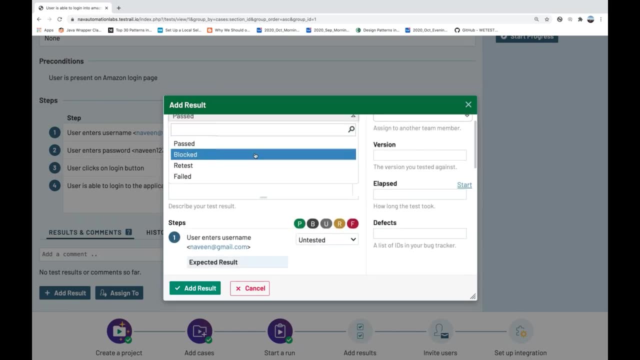 you can see the result over here and just simple click on add the test result. when you add a test result over here, you can see that. okay, you can select the specific status- pass, block, retest, fail and everything- and then for every step, this is the advantage you will be getting in the first. 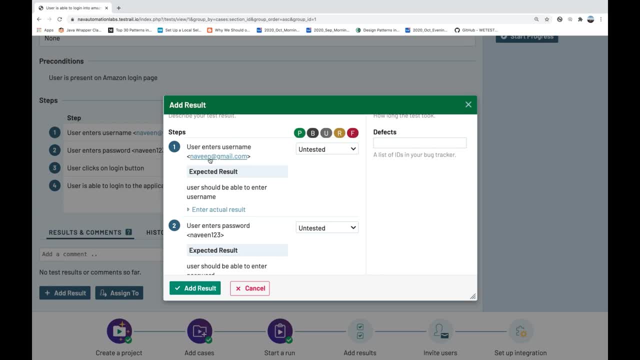 template: the stepwise template. user enters username. this is my username. an expected result is that user should be able to enter the username. so let's say, i'll open the application, i'm doing my password here and i see that. okay, yeah, this is absolutely working. fine, i make it pass over here. 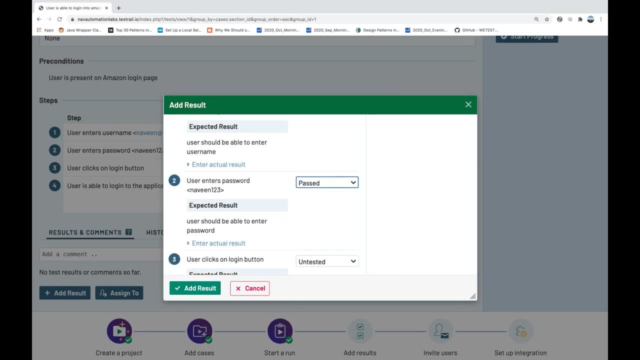 second, user enters a password. yeah, this is also working fine. so for every step you will see what exactly you want to do and what exactly you are expecting and the respective status you can change from here. and then user clicks on login button. so let's click on. passed over here then. 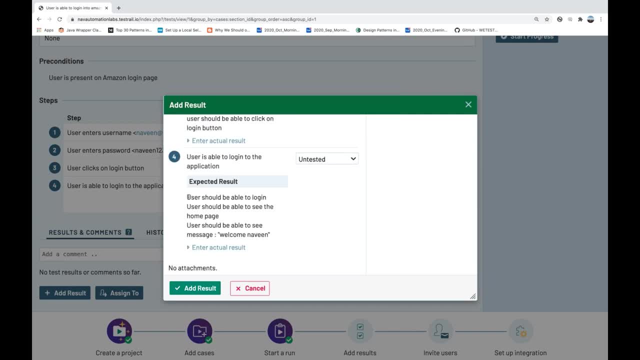 user is able to log into the application, of course. yeah, user should be able to log in. you should be able to see the home page and user should be able to see the message that: welcome naveen. and this is also got a passed over here. so all the test cases got passed and i put a common comment over here. 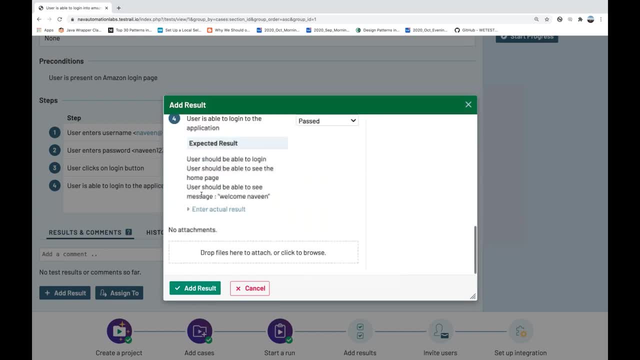 that this is as per x right like this and simple click on the result over here. or if you really want to put any screenshot or something like this or video, you can put it over here by browsing and something like this: click on add result and you see that. okay, yeah, all the test cases are coming. 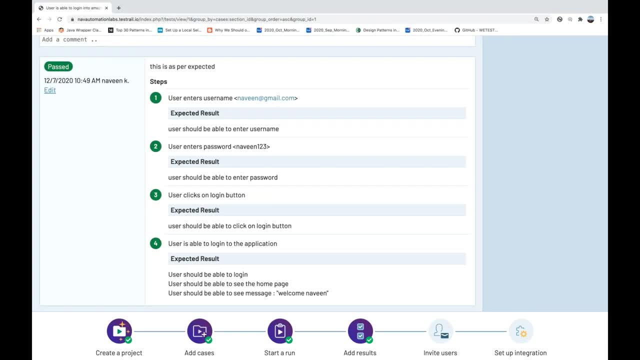 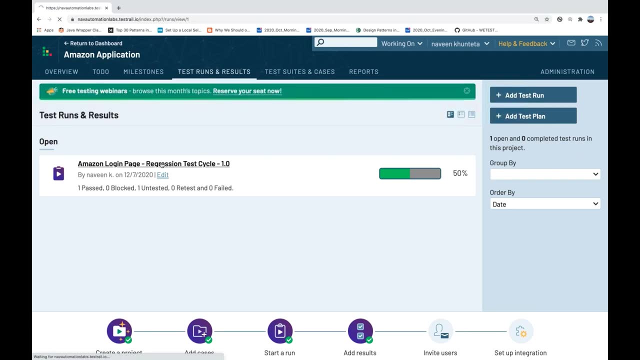 in green color, it means everything is running a fine right. perfect. then i'll go to test run result once again and i click on my first cycle once again and you see that okay. yeah, we have executed 50 test cases and someone is asking that. okay, hey, tell me the status of your test. 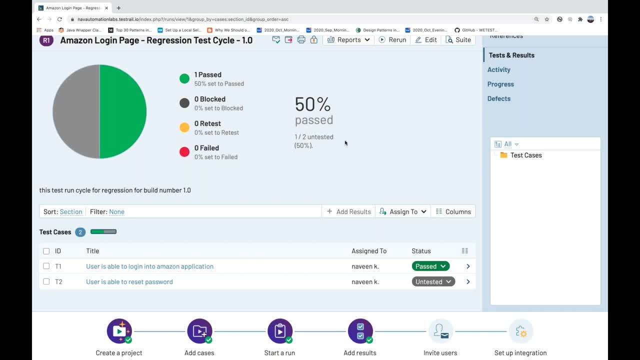 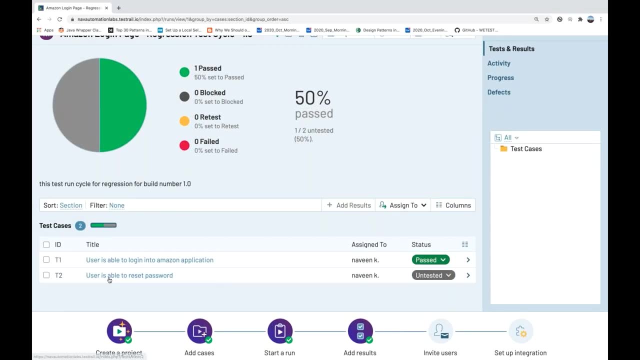 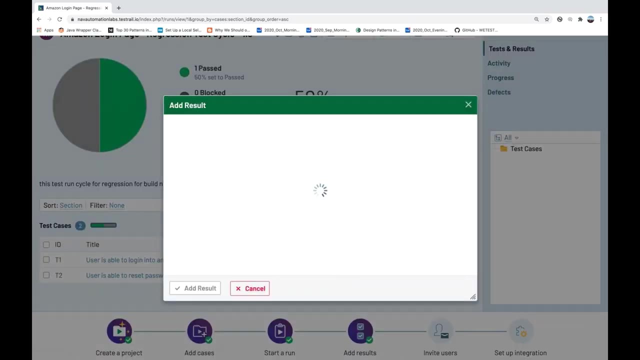 execution. i simply say yes, 50 test cases got executed and the 50 pass test cases are available like that. then i'm going to execute my second test so user is able to reset the password. so you can directly change the status over here. let's say i'm making it pass once again and then you can. 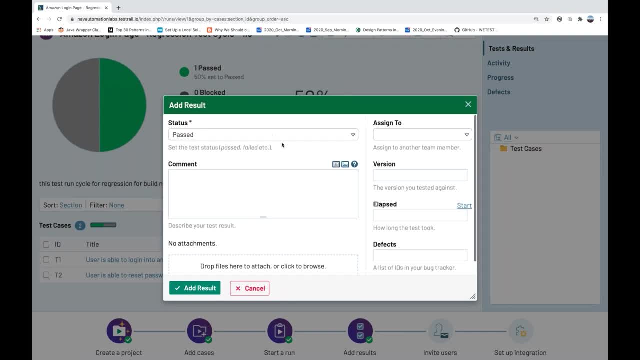 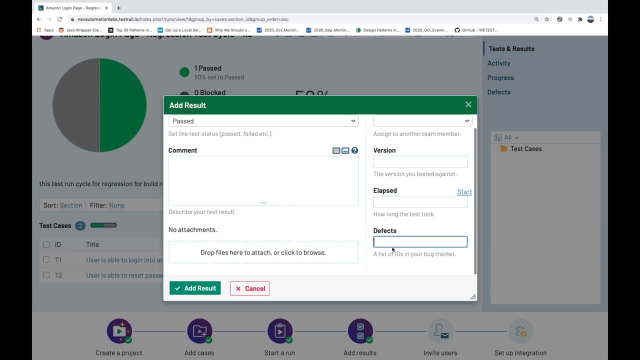 open this particular box over here and then you can simple change the status over here as well and then you can assign the test to someone and then if you have any defect, if the particular test is getting failed, you can defect id. also you can mention over here from your bug tracker. 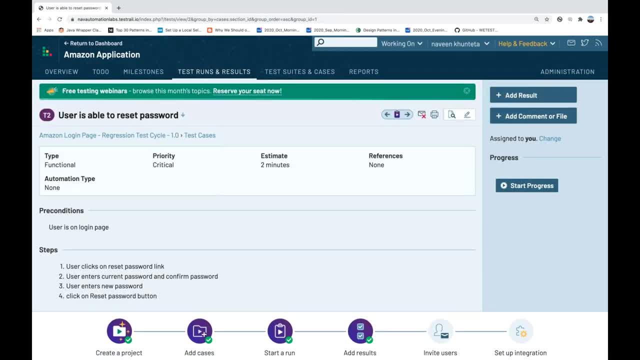 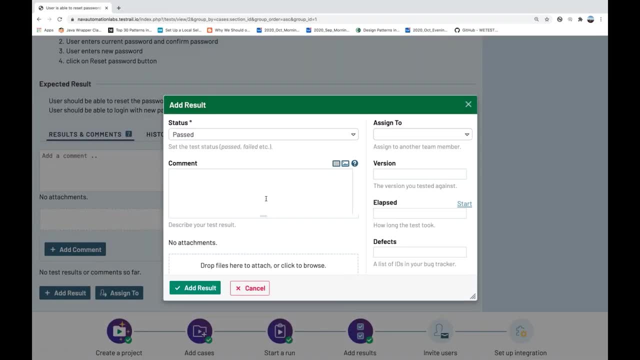 so let's see, i'll do one thing: i click on this particular link and then i simply say that, yeah, if you have any comment, you can add it. or if you have any result, you simply click on add result and then i simply say that, yeah, just, uh, what is the status? status is passed. i still say that, okay, yeah, this is s per. 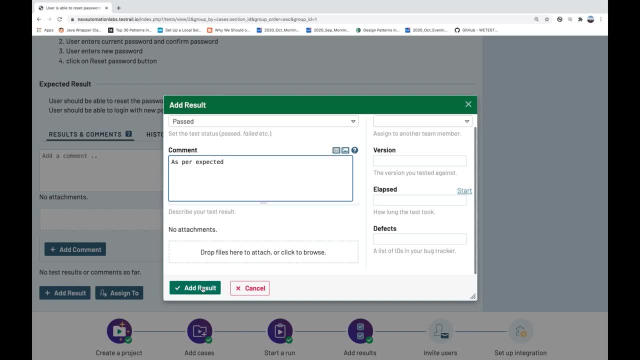 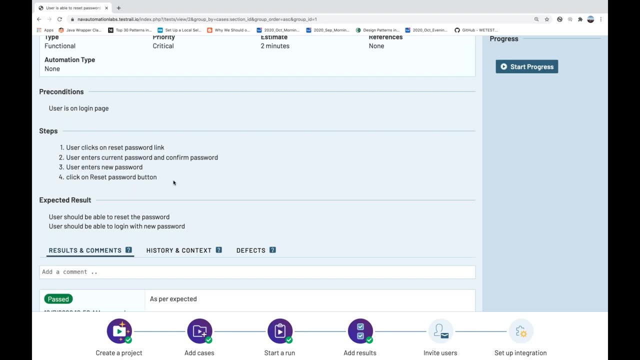 expected like this and then click on add result: perfect. so this is also test case got passed. so i'll read this information from here. but this template is outdated template guys generally, i it's again. it's up to you. if you're comfortable for writing this particular template, you can do. 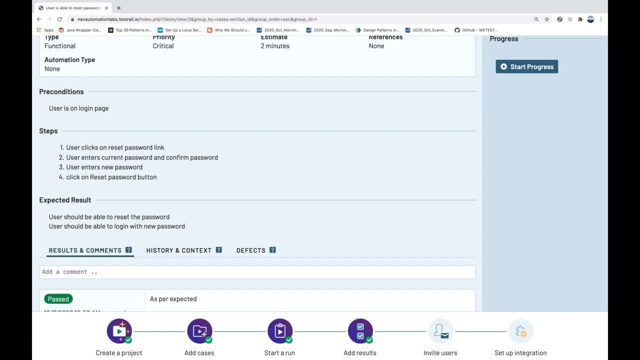 that, or if you're comfortable writing a template in the form of a multiple steps. for each and every step you can put what exactly pass, fail and actual result is coming against each and every step. that also you can do that, and some people they prefer this, so it's up to you which. 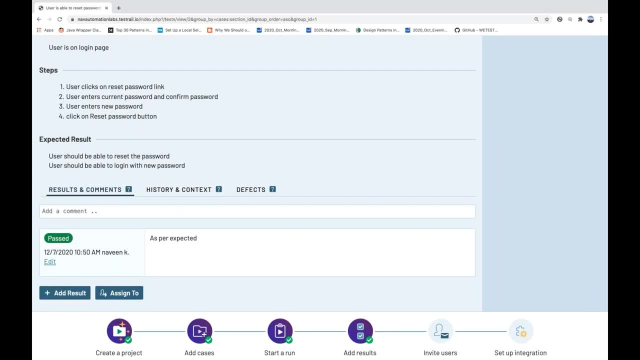 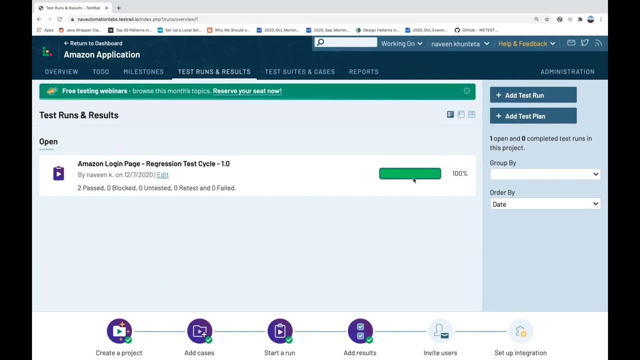 template you really want to prefer for writing a disk case, and then this is also done over here and then again you go to your result. run go to this particular cycle, but before that you can see that 100 green bar means everything is fine in this particular cycle. if someone is seeing that, okay. 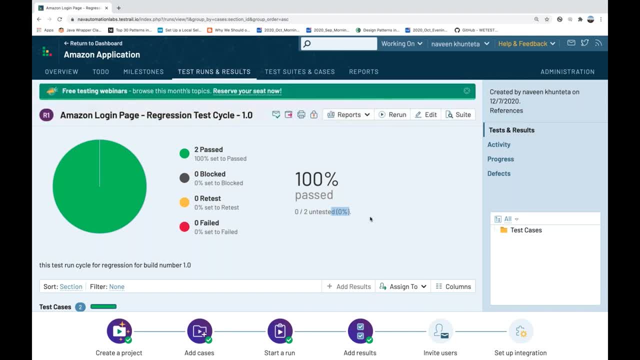 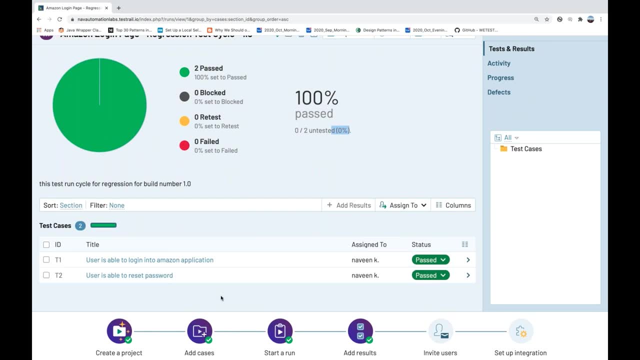 yeah, hundred percent test cases and we have zero percent of the test cases and we have zero percent untested. everything is getting passed over here, let's see. but again you are checking the application and then let's see: reset password is not working now, so i can make it a fail also. 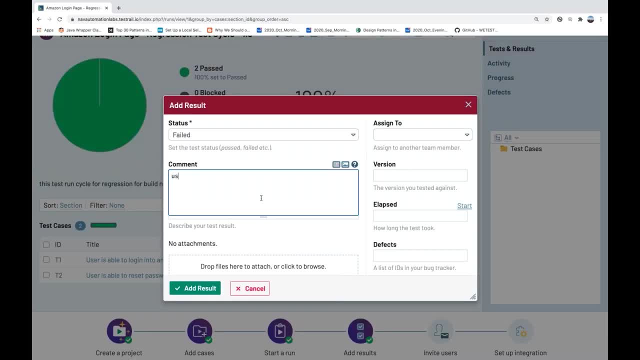 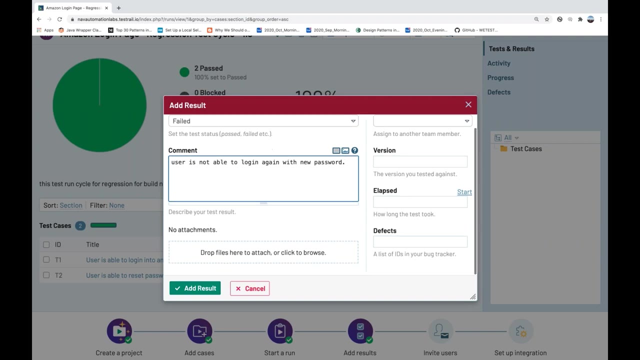 let's see this time and then saying that, okay, yeah, uh, i simply say a reason over here why it got failed. i simply say that, okay, yeah, user is not able to log in again with new password. whatever the password that we have reset, user is not able to log in again. let's see, this is the. 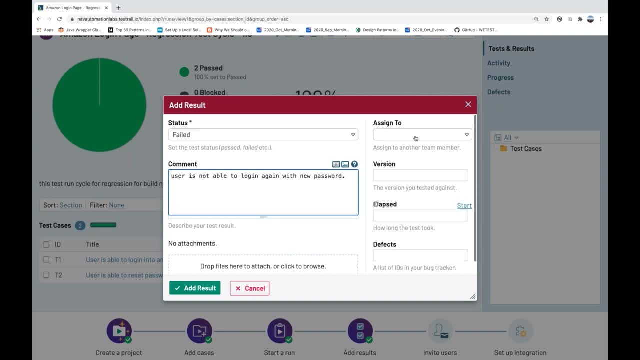 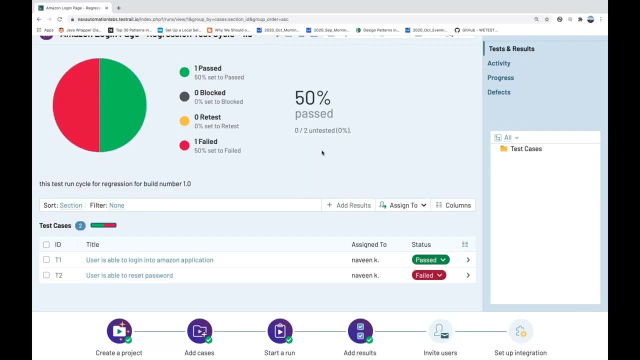 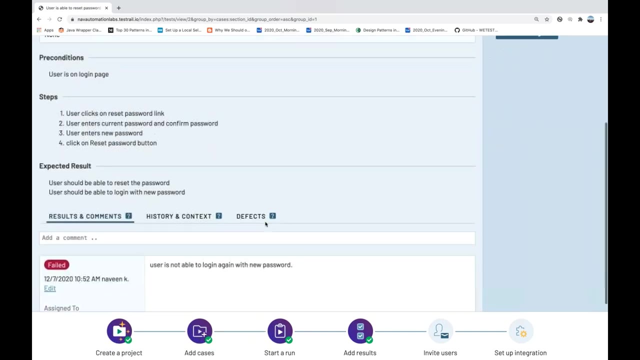 actual result, that i'm getting it and let's see: assign to naveen once again and click on add a result. you can put a screenshot and immediately your status will be changed in this particular cycle, right like this, and then you can come over here and you can check that. okay, yeah, what? 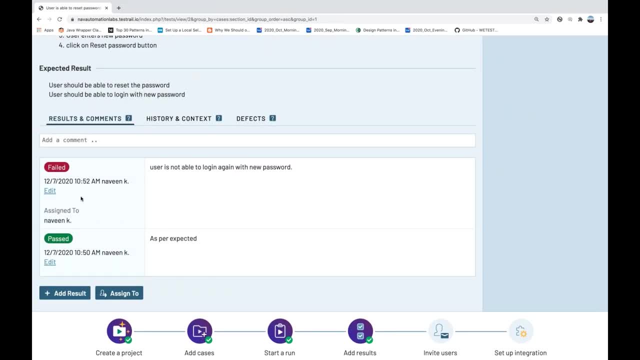 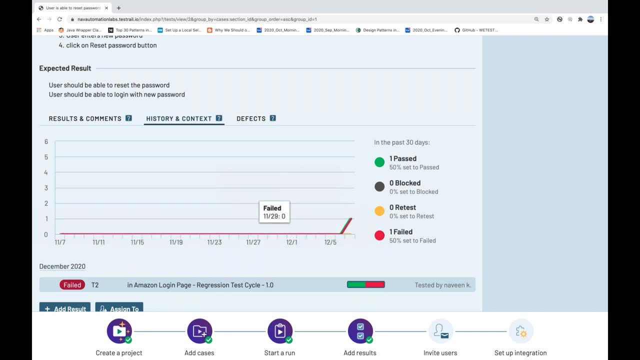 happened earlier, it was getting passed, now it is getting filled. you can check the history. you can see that, okay, the graph like that, and then, uh, you can check that and again, whatever different elements you can edit i will include here. you can add a new function, like i said, if this one. 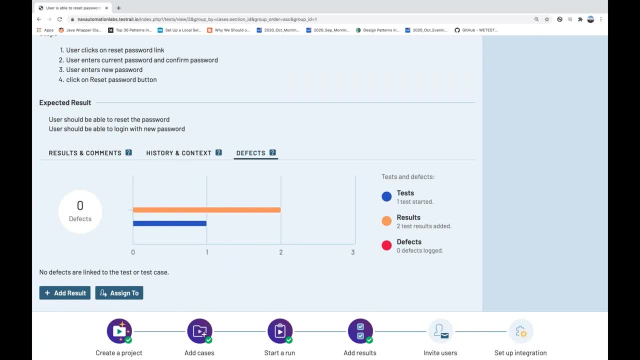 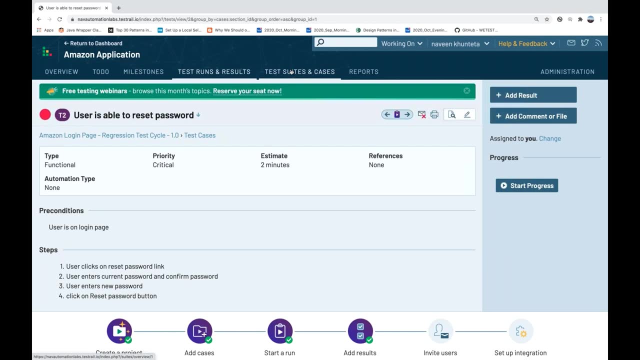 i'm not adding anymore. in case you need a different one, i will add a different one. so let me just build a new one for you. and then also, what i'm going to do is for this one you can put a default default ID, because if you can't see it well, let's say default. default is out of this. 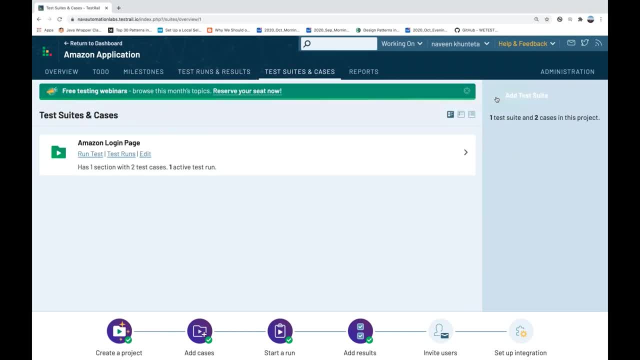 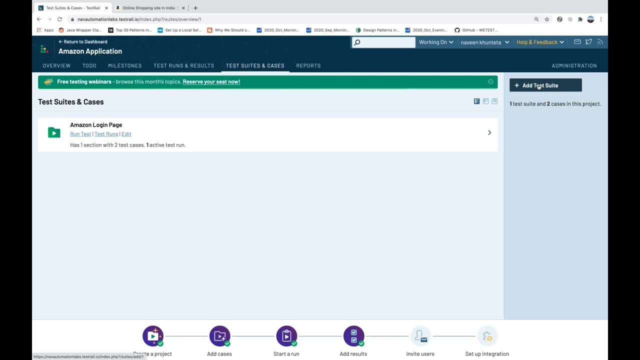 one. so let me get that default default ID and i will add another default default ID. and we want to add other default defaults. for example, let's say we want to add a test case, so let me add a number of test cases over here and then again you can add more test cases like that. so right, 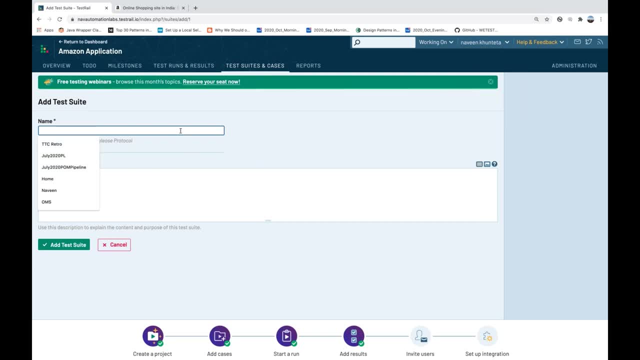 here here, right, this time I'm giving a different suite name. let's see I'm giving that is Amazon search feature suite, something like this I'm giving right, and you can write up some description about what exactly you are gonna test it over here and what type of test cases you are going to write. 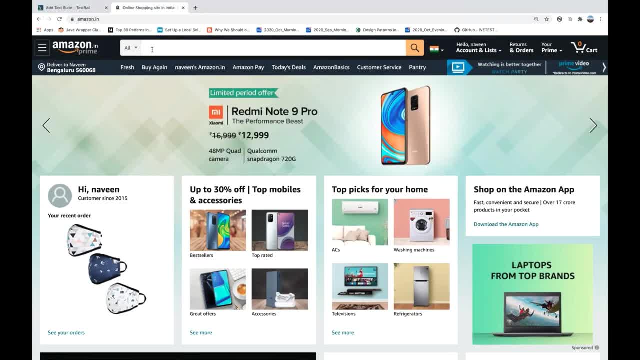 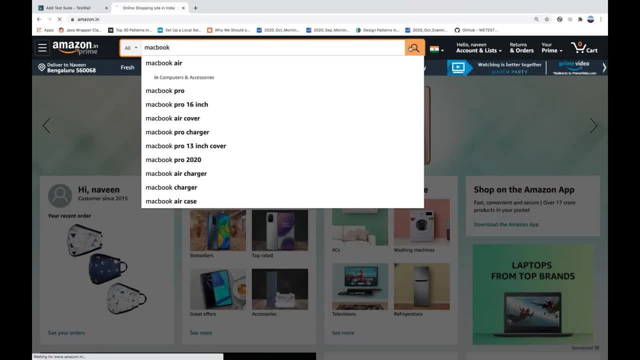 so you see that, okay, this is Amazon application that I've already opened and you can write something, you can search something. let's see, I'm writing a MacBook over here that I'm searching and from the search field, and then I'm checking filters, I'm taking different results over here. 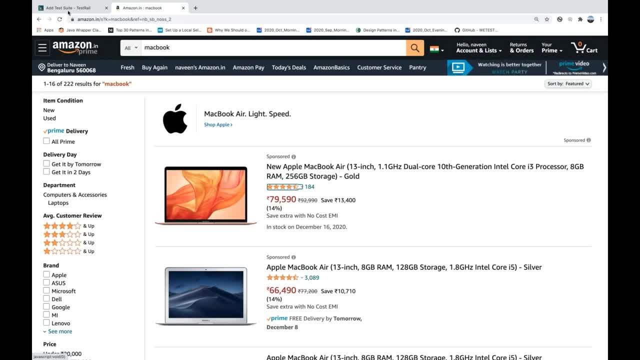 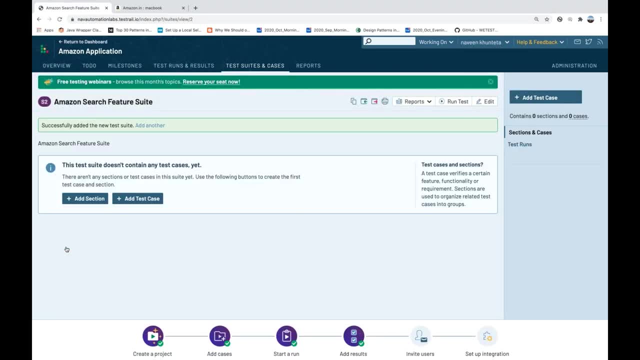 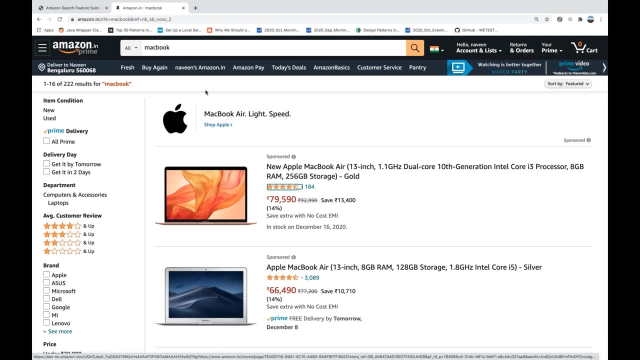 complete flow that we really want to write. so let's write up some basic flow over here. so click on add test suite and if you really want to, that, okay. in search, like: see, I want to do that, search a with this particular search field and then a filter search also I can do that. so I'm going. 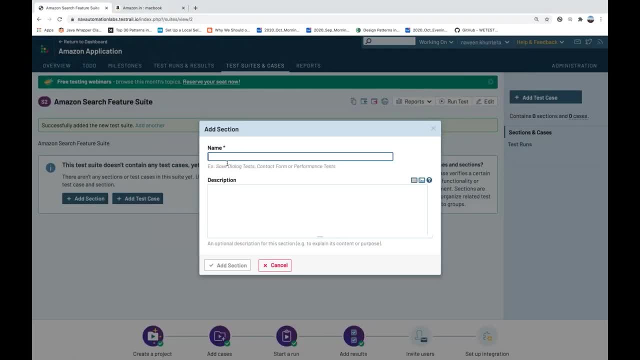 to create two section over here. I'm going to create one simple basic search, basic search and I simple right, this is test cases for basic search. I'll be writing 60 test cases for a basic search, okay, and then click on add section over here, and what I'm going to do? I'm going to add. 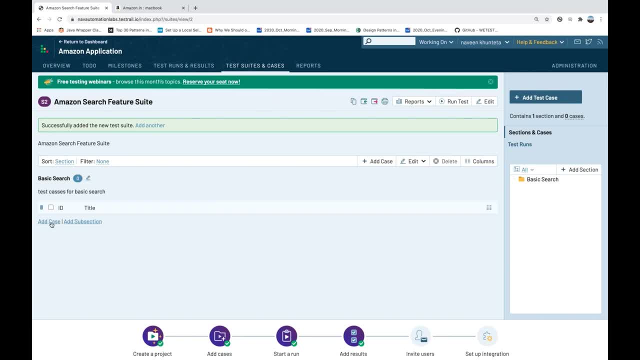 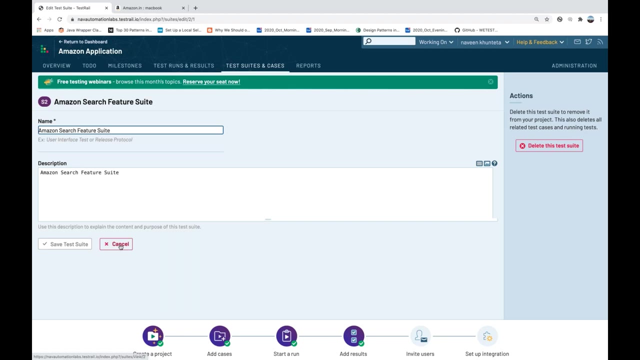 a some test is over here, so let's create a test case over here. let's see, click on add case, or you can directly add the case over here as well. if you really want to add it, you can add it also, and let's, if you really want to add it. i think we have to add search feature suite. this is fine. 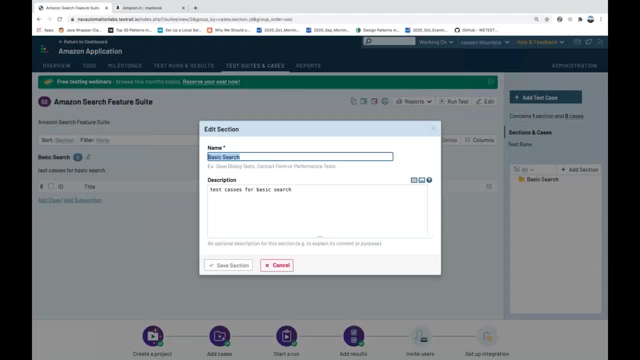 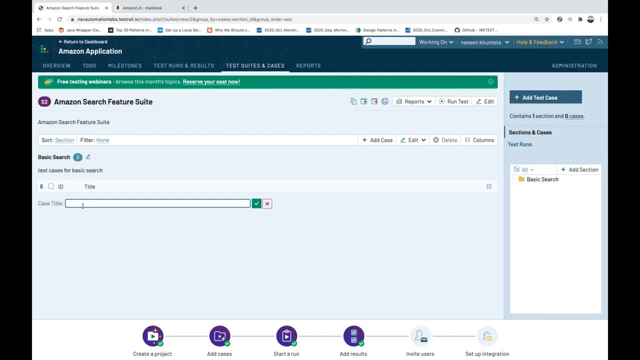 and the section got added: the basic search. if you really want to add that particular section, that also you can do that. so let me save the section once again. click on add and the case title is what i simply write. let's see, this is my a basic amazon search. okay, this is a title with. 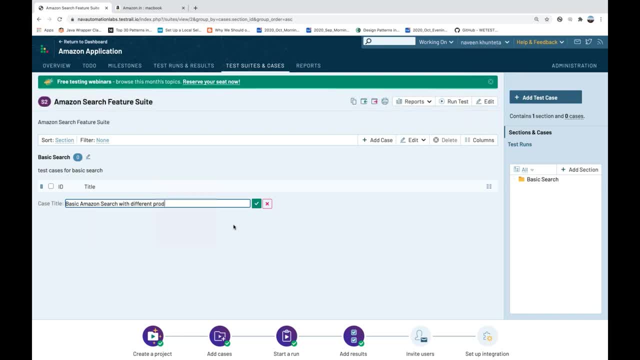 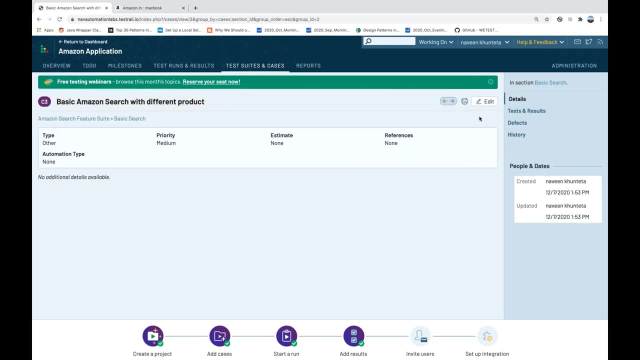 i would say with a different product. okay, so i'm just writing some basic test over here. this is the case got created, case number c3 and then you can click on edit and basic search is i'm going to select which template. i want to select the test. 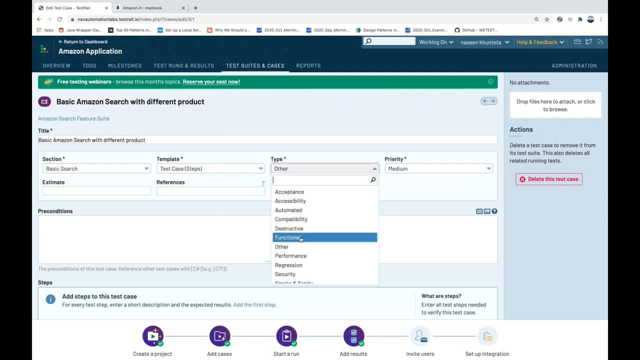 case with that steps template. i want to select what type of it is. it is the functional test. what is the priority? the priority is, let's see, critical because user has to search over there. and then, what is the precondition? the precondition: i'm going to write that, okay, user. 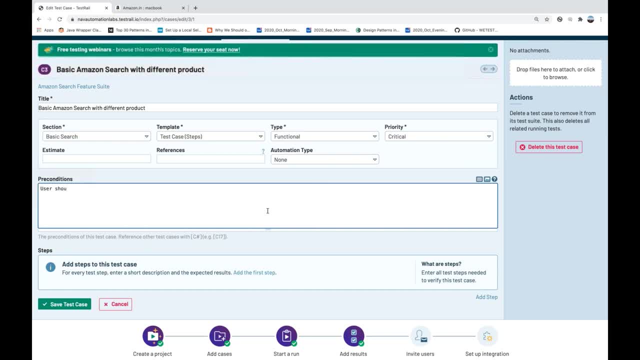 and should be able to. or i would say, user has already logged in. okay to application. and i would say that user is already logged in. uh, add a step, add on. just want to put a step over here, this step over here. this is a pre-condition and uh, simple click on: add a step over here. so this is the edit step. 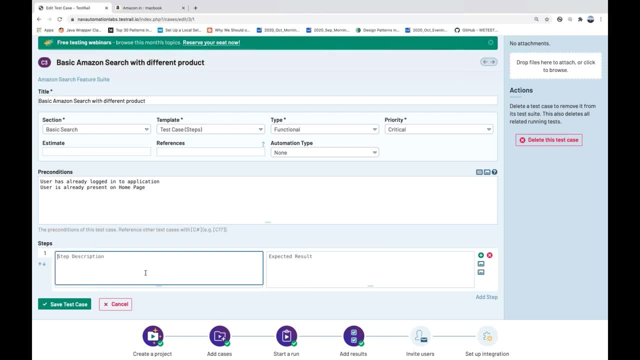 and right step over here. so my first step i'm gonna write. you don't need to write one dot because one is already written. so what is the description? let's say i want to enter, click on search and then enter some field over there. so enter some product named over here. so i simple write, Click on. 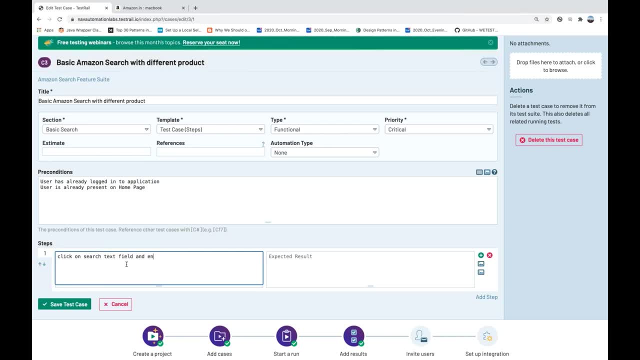 search text field and enter some product name. so let's see my product name. see, guys, follow this particular pattern whenever you are using your test data. so or you can use a double codes also, or you can use this particular pattern. i always follow: whenever there is a variable part in your test case or kind of test data that you are using, it i always 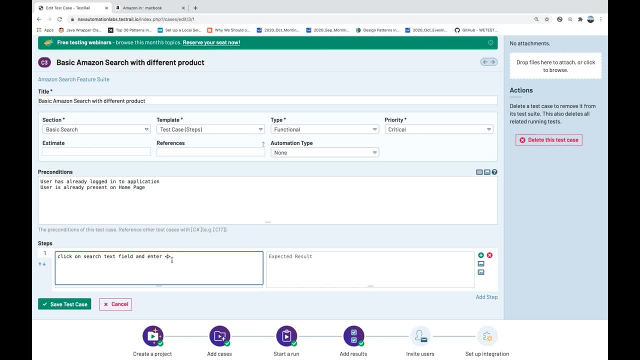 prefer within these two brackets or diamond bracket. i can use that. so let's see, i want to search for macbook air, i want to select a macbook pro, i want to select, and when you search, click on search text field and enter this and then click on a search button like 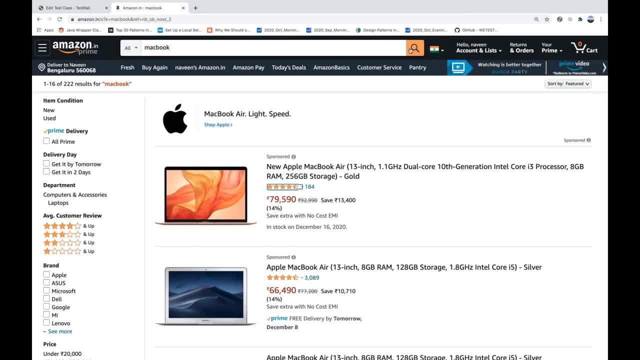 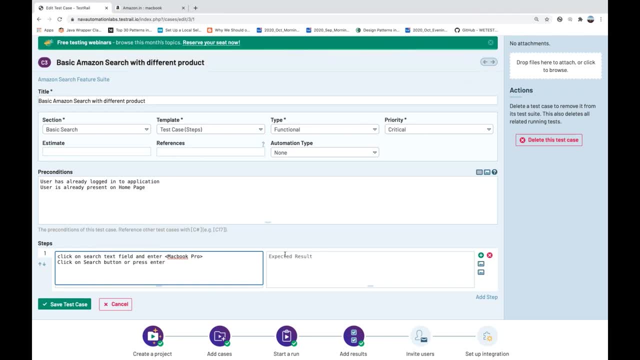 this right. when you enter macbook over here, you have to click on this particular search button or icon, whatever, or you can press enter also click on search button, or i simply right press enter. what is the expected result? so when you search for macbook air, you can just click on your search button right there. you can. 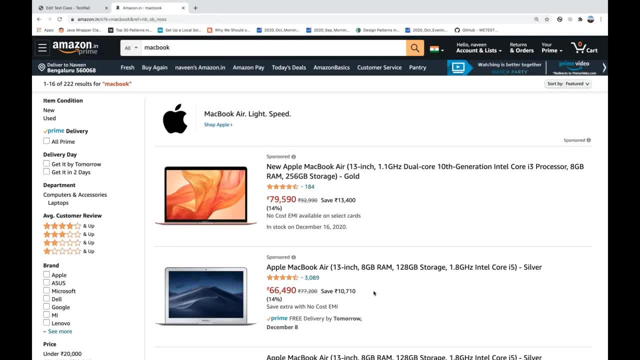 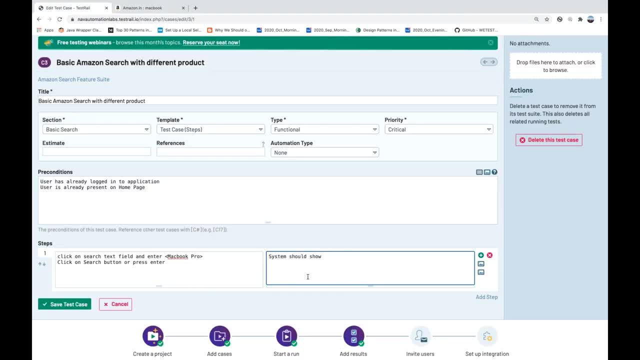 search for macbook air, as many of you have a X on it already. but look at this: correct that the respective test, respective results should be displayed with respect to macbook. so i simply write that system should show results for whatever data that you're looking for. 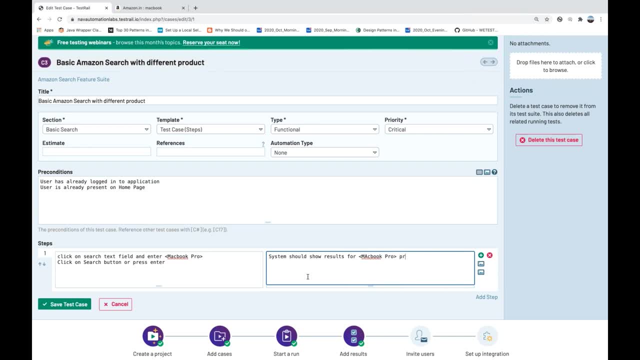 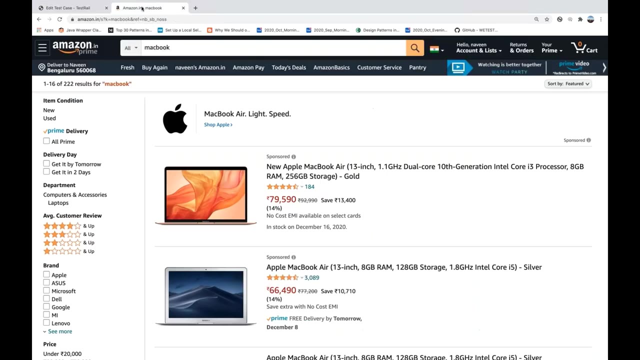 for macbook pro product. okay, in the results section like this, and then you simply click on add- step over here. so this is my first step that we have added. second thing: let's say i want to do that. okay, i want to click on a specific product over. 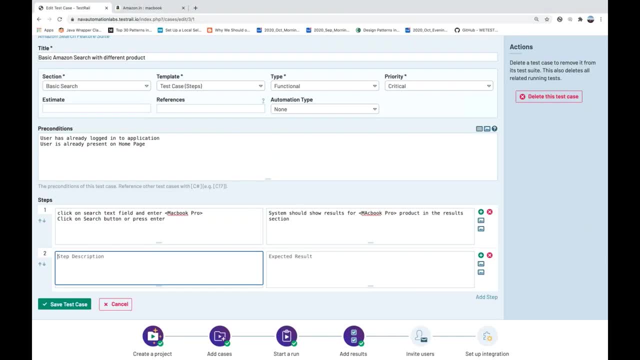 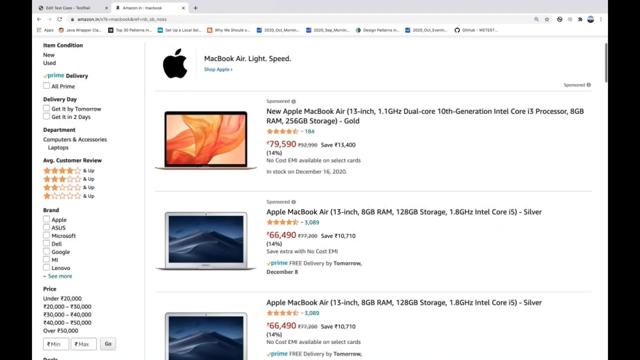 here and i simply say that, okay, let's see, click on the first product and i simply say that system should, uh, display what exactly we do, that let's say i'm clicking on the first product that we got. so let's say i'm clicking on this and i'm going to click on this. 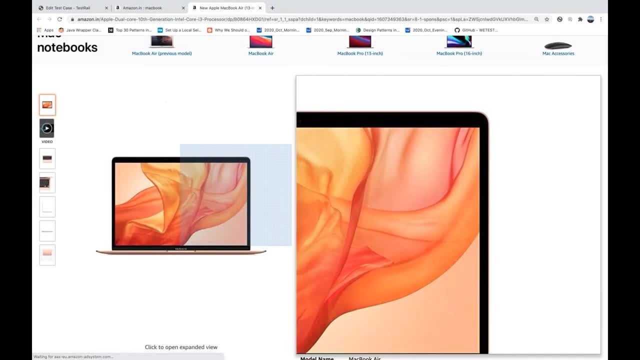 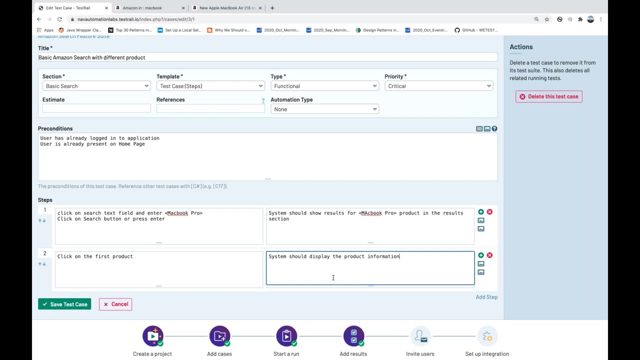 and i simply say that, okay, yeah, user should display the product information. i'm simply writing like this. so i simply say that, okay, user should display the product information. and what kind of information? like something, let's see price. then you are going to write description and then the seller details. 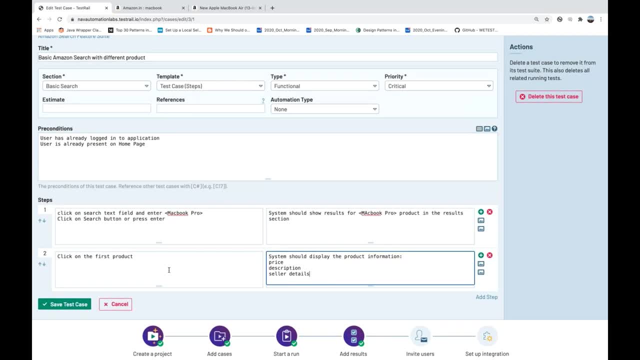 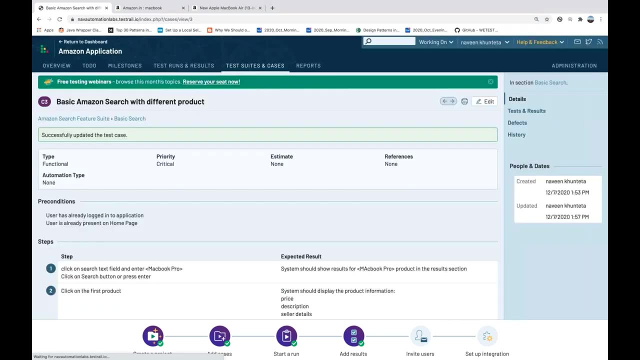 whatever. then blah, blah, blah, you can write it. i'm not going to write everything over here like this. so let's see, this is the two steps that we have written, and and just simply click on save test so it got saved. having to a test, uh, steps that i have written within this particular amazon search. 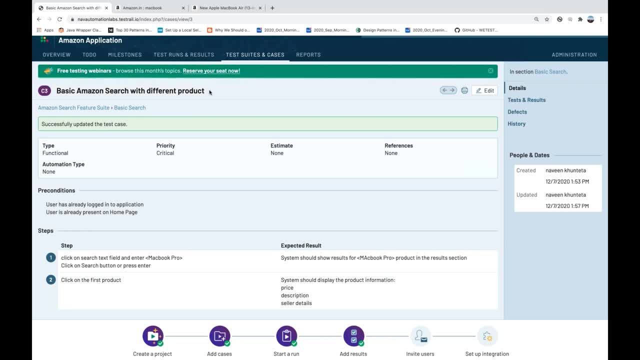 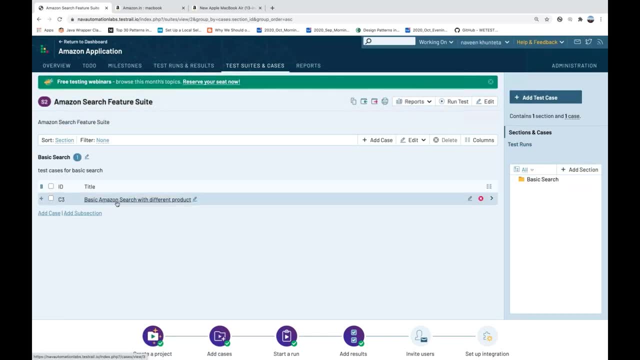 with a different product or a specific product. whatever you want to write, you can write it. okay, now you do one thing. you just simply go back to this amazon search feature. you can see having one test over here like this: perfect, now, if you really want to add one more subsection, that also. 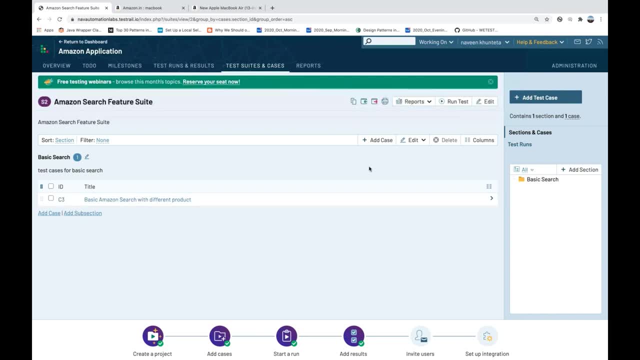 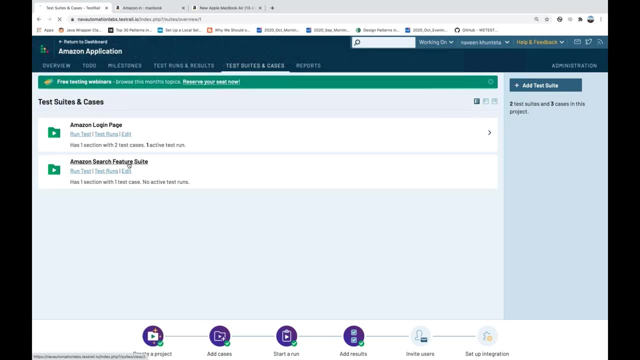 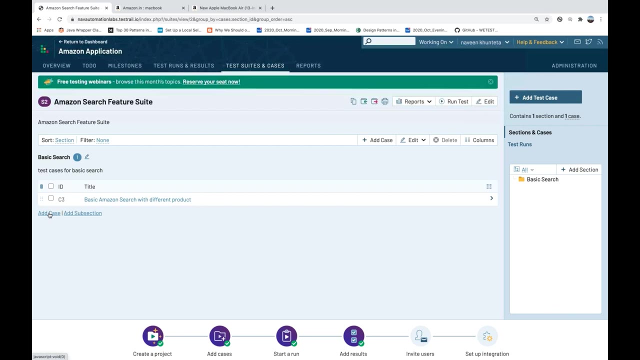 you can do it over here, guys, right? so i'll do one thing. i'll go to my result suite in cases. over here you can see that amazon search feature suite got created. you just click on it and you can see having one test over here. if you really want to add more, more cases, you can add it more and more. 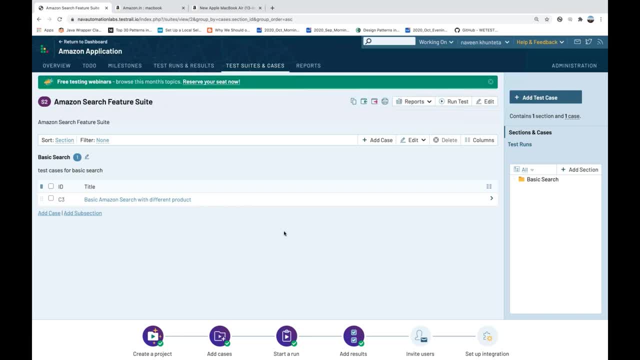 test cases over here like that. okay now, uh, we do one thing, that is us. let's do one thing. let's click on um, add it over here, and okay, this is fine and i'll add one more instead of subsection. i'll add one more case over here. 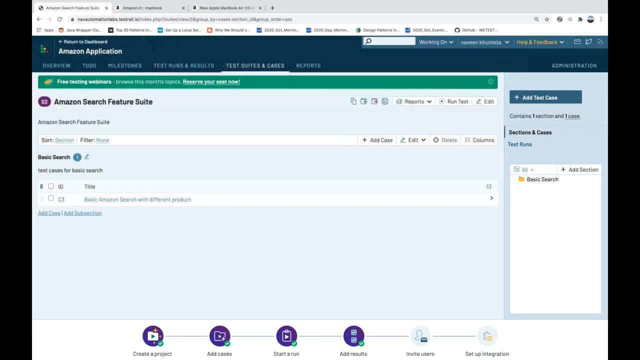 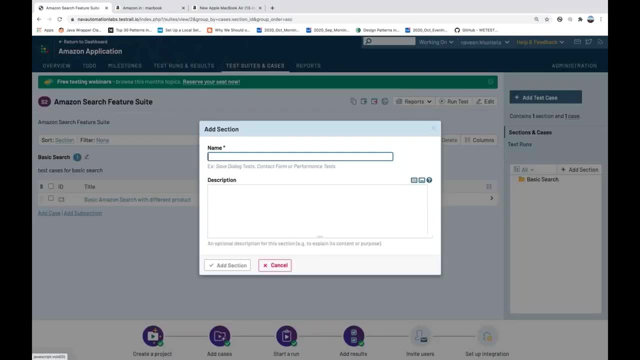 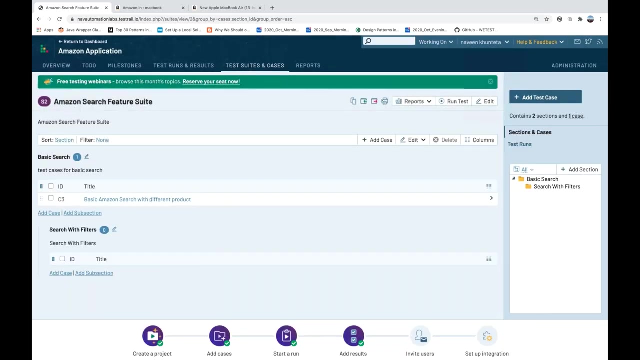 okay, can we create one more section? that will be good. so this is a section, okay, i think. uh, add a subsection and let's see if i really want to create one more subsection. let's see search. i'll simply write search with of filters, right, this is the section that i have created. so, yeah, one more. 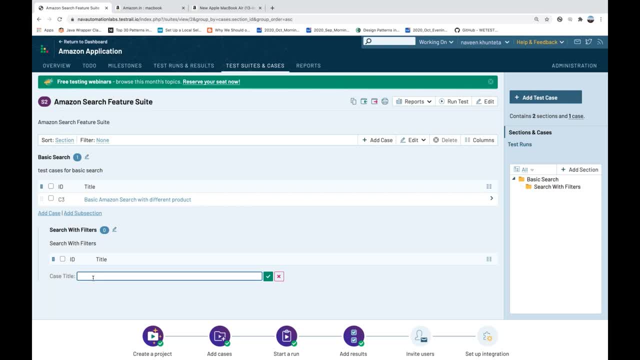 section got created and then you want to add one more case over here, i simply write that, okay, user is able to search with different filters. see, guys, why i'm writing all these things? so that i can show you this is what practically generally we do that okay, but i'm not writing all the full flash test cases that. 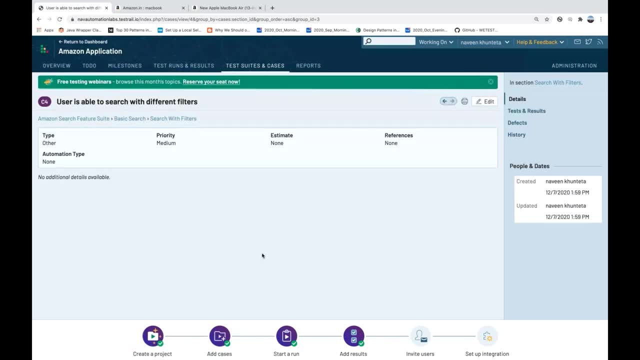 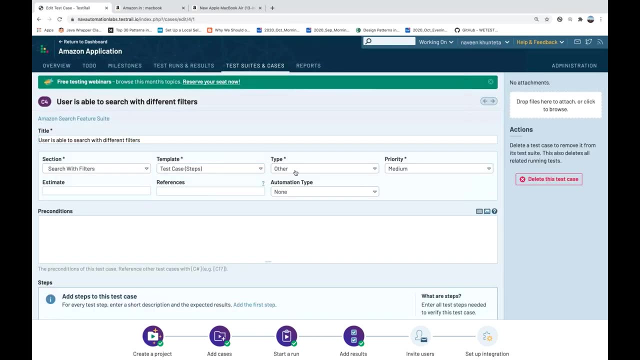 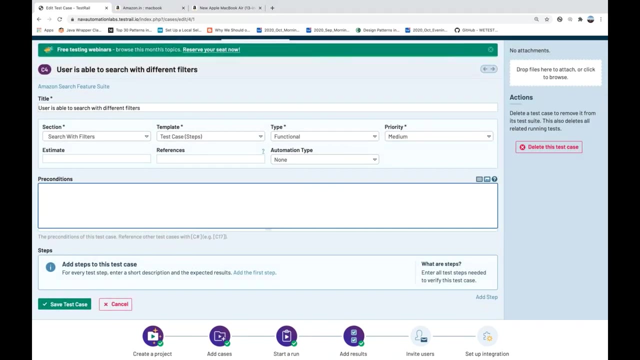 you can practice accordingly and then you click on this and then what you do? you simple edit this and let's quickly add uh, one more, uh test over here with different steps. this is again part of functional. the priority is let's see medium, not that okay filters, and i simply say that: okay, user. 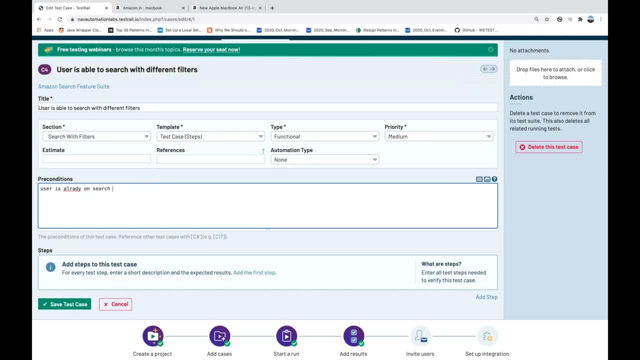 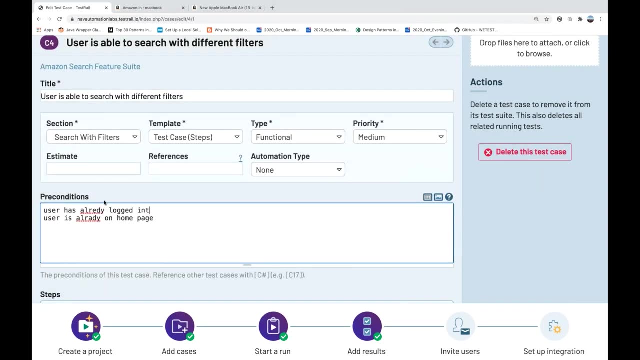 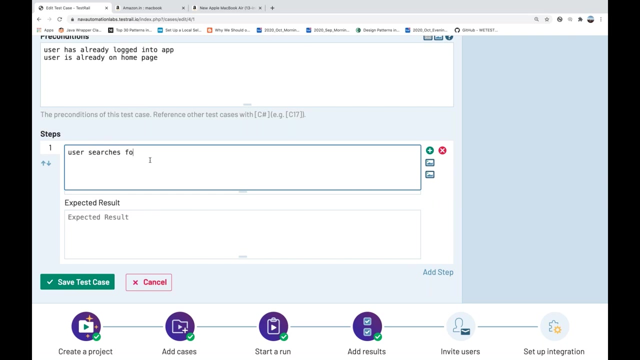 is, uh already on home page, like that. so user has is already on home page, and i would say that user has already logged in to application. okay, so, okay, perfect, and uh, let me quick add one or two steps over here, so i simply write: user searches for some different product. let's see my product name is: 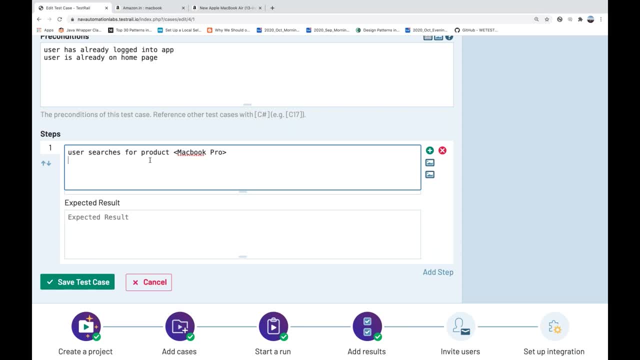 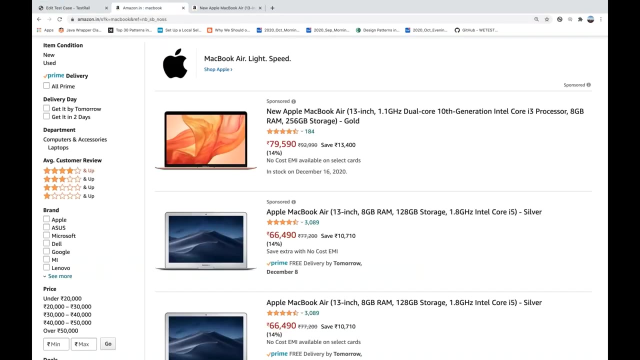 i simply write macbook pro like this. this is my first step. and what exactly you are expecting? okay, all the uh products with filtered section, because you see that when you display the product details with the filter section over here, this is these are called filters. all right, and uh, yeah, so this. 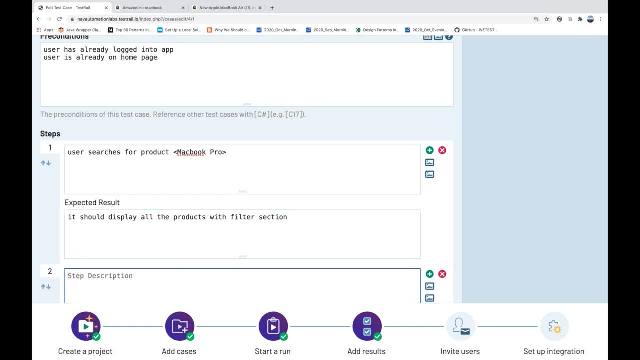 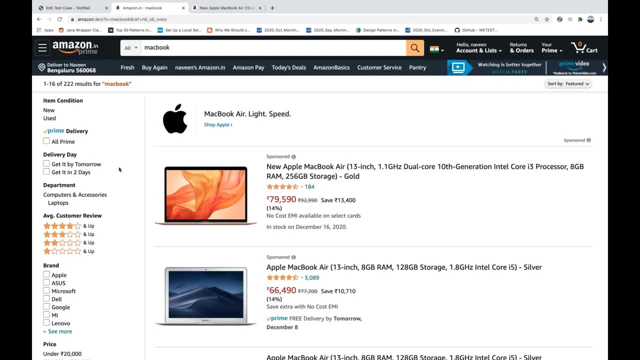 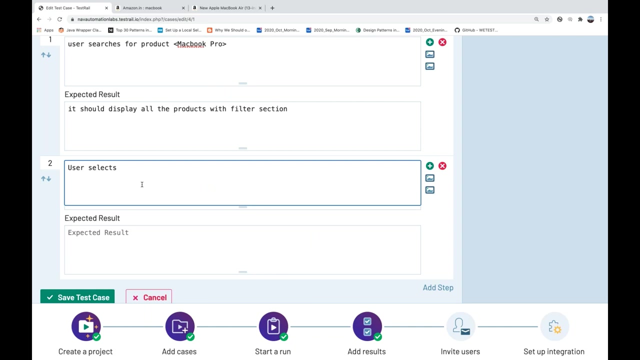 is my first thing and simple: add one more step over here and then i simply say: user selects or checks filter. let's see, uh, the delivery day, right by tomorrow, or within two days, or something like this. let's see: user selects delivery day as okay, let's see by tomorrow. then it should display what, then your 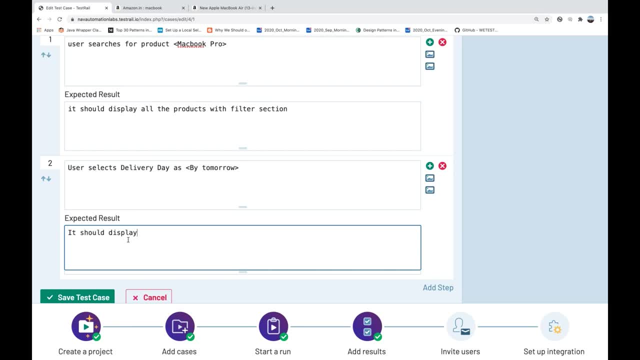 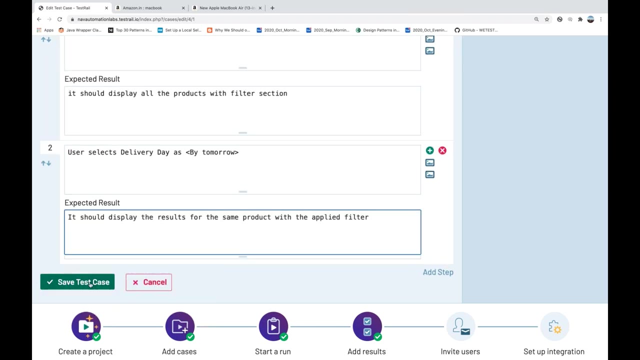 system should display the results for the same product- remember this thing- for the same product, with the applied filter, whatever the filter that we have applied over there. so like this: let's see, i have added this, i have added this particular test over here. having two steps now perfect. 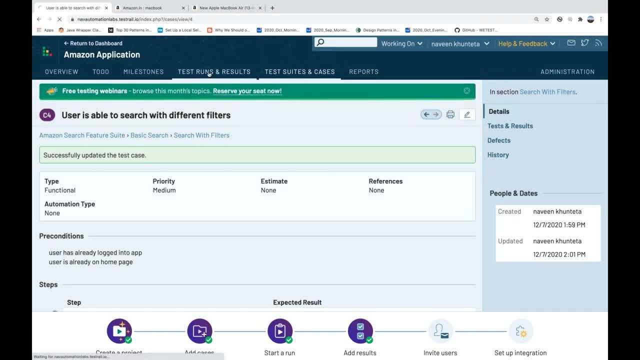 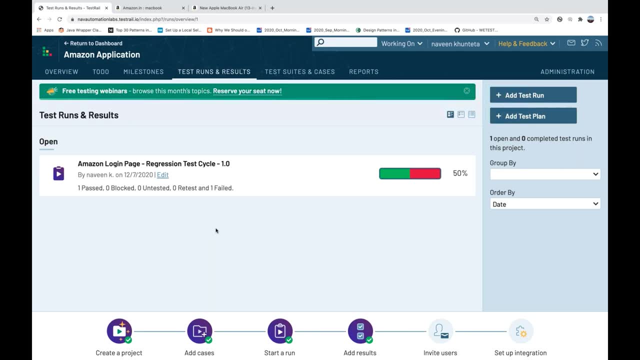 now it's time to execute the cycle once again. so i'll go to my test run and let's see. this feature is available in the next cycle, in the next build. and, uh, we have to do a regression. so i have to start my regression test cycle number two. so how to do that? i simple click on add a test run. 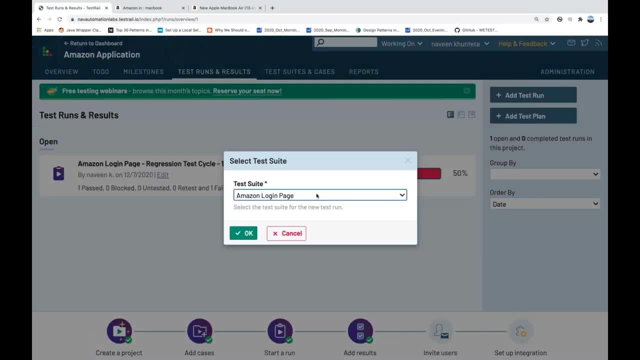 okay, and then simple click on add, test run, and this time i'm giving a different- you can select which suite that you want to select. so let's see, i say that okay, yeah, i want to select search feature suite because, uh, in the next regression- let's say you want to do that, i would say that. 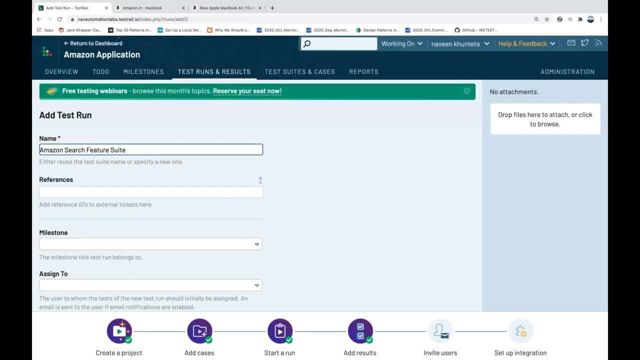 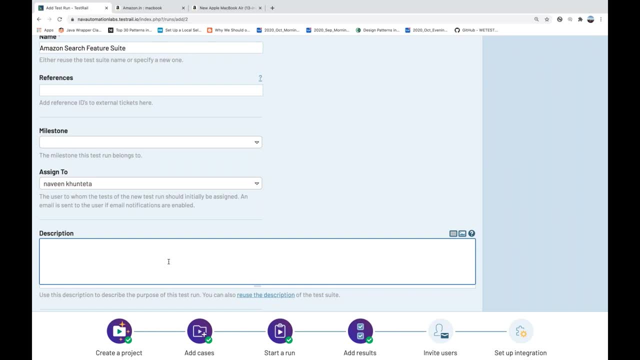 okay, i want to do a amazon search. you click on okay and then you can put your references, any user story or something like this assigned to someone, let's see to me, and the description you can write like this: include all the test cases, yes, or specific test cases. you can also do that. 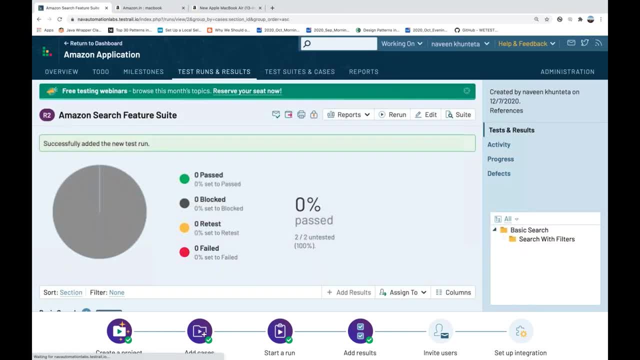 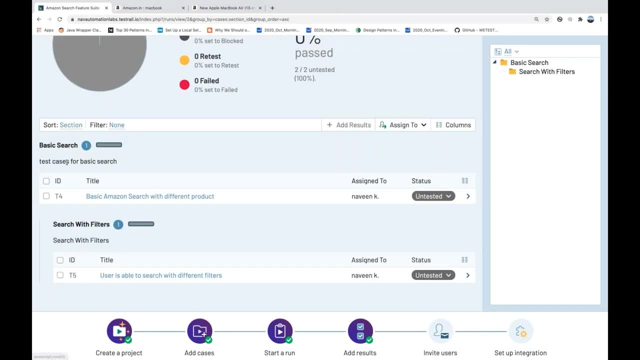 but let's include all the test cases. click on add test run. you will see that. okay, yeah, amazon search feature suite that i have created which is having a basic search, and then then we have subsection that is called search with filters also, and this is also having one test and this is having one. 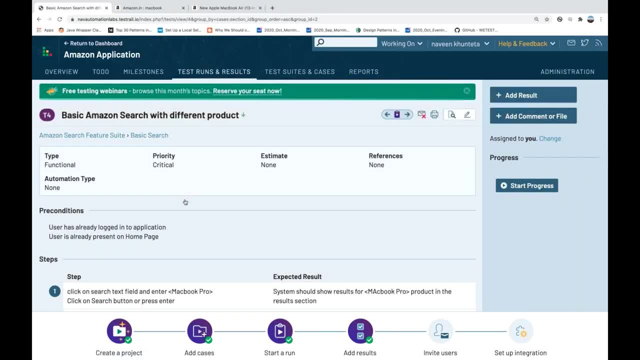 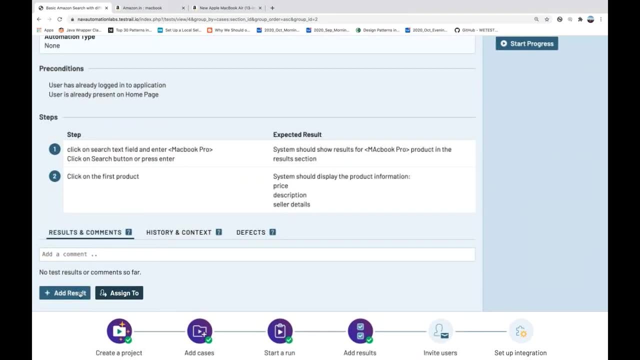 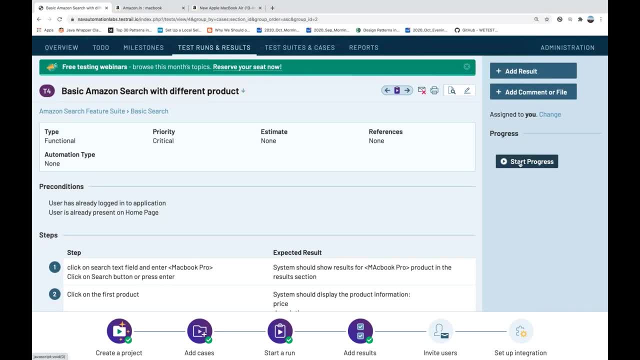 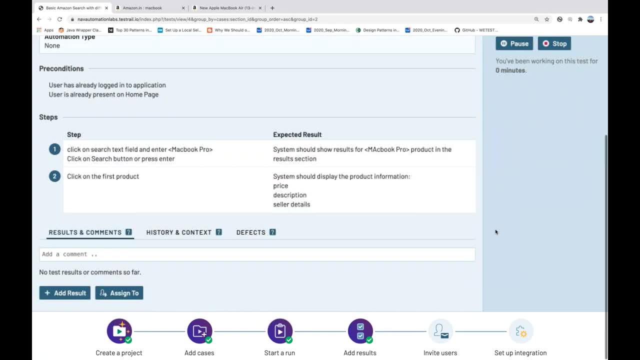 the result, what you can do. you can click on this: start progress. it will calculate that okay, how much time it will take. you can see that you have been working on this test for zero minutes so that you can actually time. you can actually calculate a time, how much time i'm taking it. so let's see. 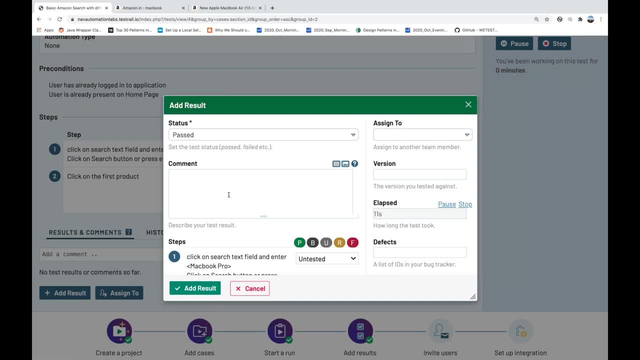 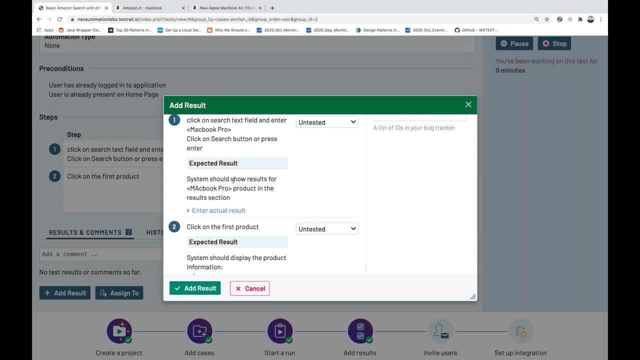 add result. i see that. okay. yeah, search is absolutely fine, and then i'll come over here. the first thing is that click on search text field and for macbook, and expected is that search system should show a result for macbook. it got passed, perfect and uh. second guy: 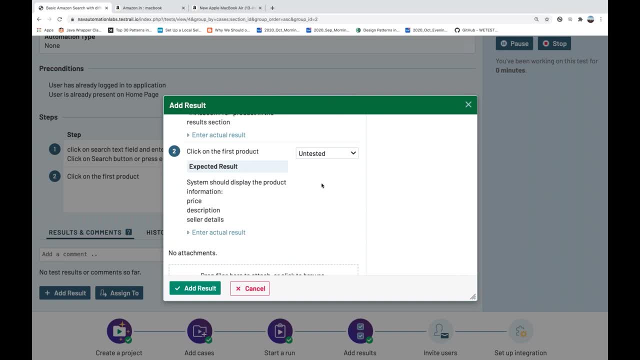 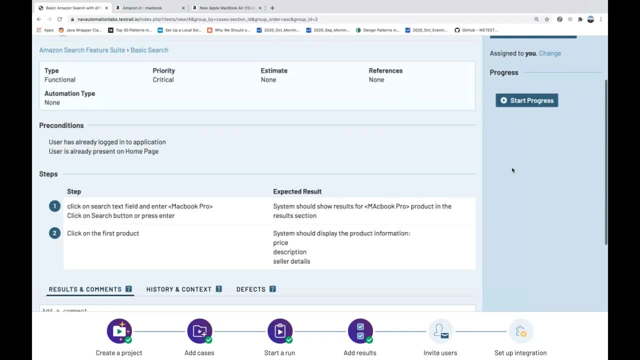 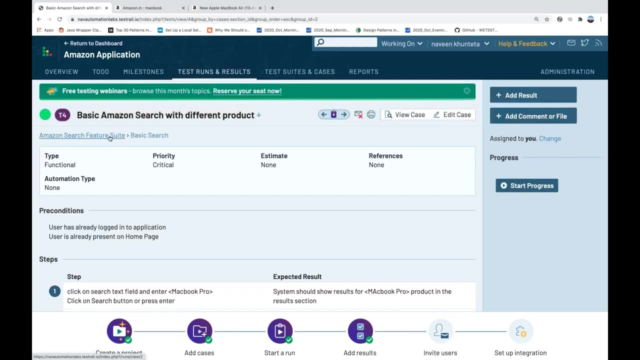 also, system should display the product information with price description, set of details. this is also got passed like that and then click on add result. perfect like this, so you can see that all these information over here again. i'll go to uh click on this. basic search is done, 50 test cases got. 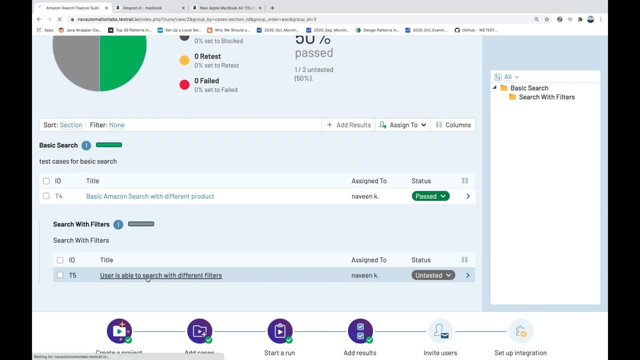 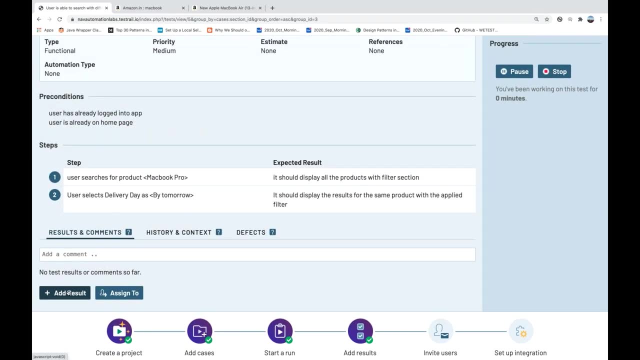 passed and then i'm going to search with a filter and then i'm going to click on add result and then the filters click on this and then i quickly again start the progress. i want to calculate my progress over here. click on add a result over here and let's see the filter is not working. so i simply 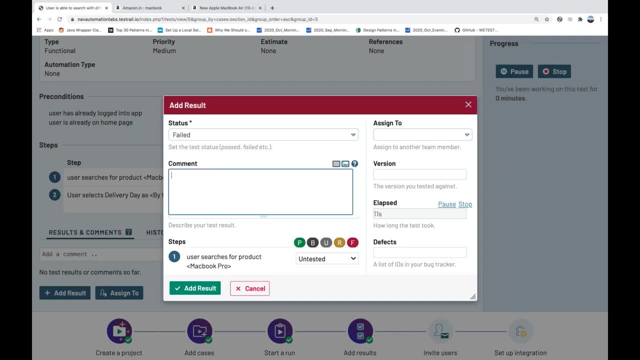 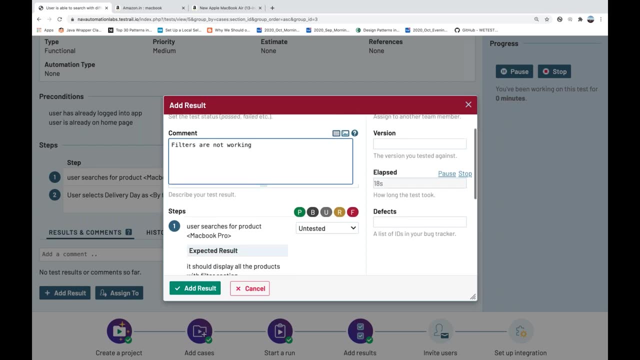 say that, okay, yeah, this is actually a failed over here, and i simply say that, okay, filters are not working right, and i simply say that the respective test got failed. user is able to search. let's see, this step got passed, but user selects delivery day as tomorrow. this is also passed. okay, but it should display the result for. 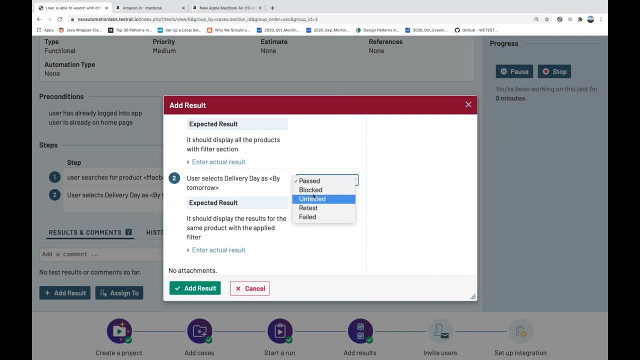 the same product with the applied filter, which is not getting passed. so let's see, overall, the step got failed over here. so i mark it failed over here. it's not a blocker, but it got failed and if you have any specific defect, let's use the same defect you are going to raise and then you can put over. 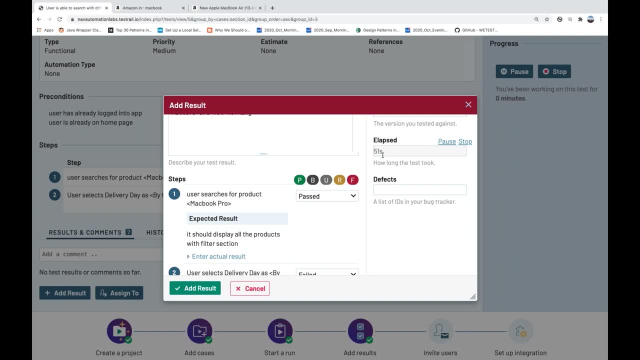 here so you can start a timing timer over here, because we have given one minute, i think, and it's taking that. okay, yeah, elapsed 53 seconds. oh sorry, 53 seconds or something like that. so let's see if we can stop it. you can pause it, okay, like that. sorry, forget about one minute. that was. 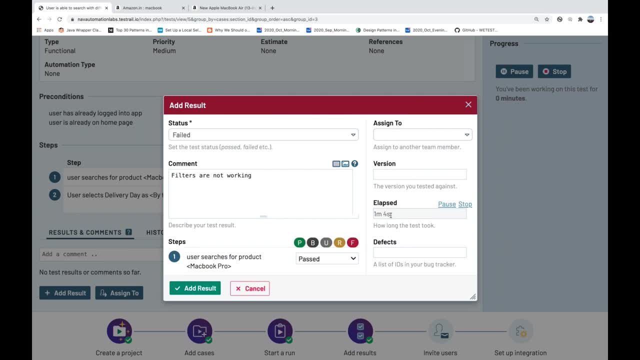 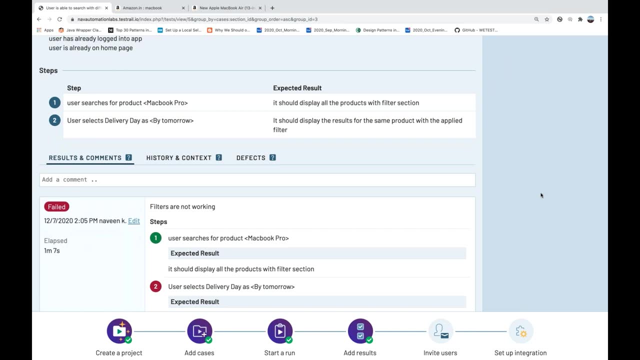 nothing related to over here. it means how much time you spend on this- one minute, two minute and all those things- and click on add result so that you can calculate this thing, that okay, how much time for this particular test generally we take so you can calculate the effort estimation and. 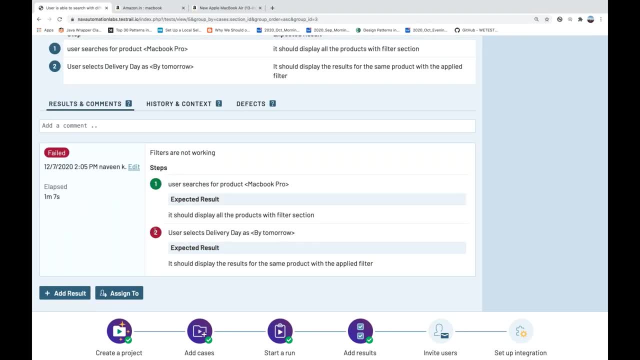 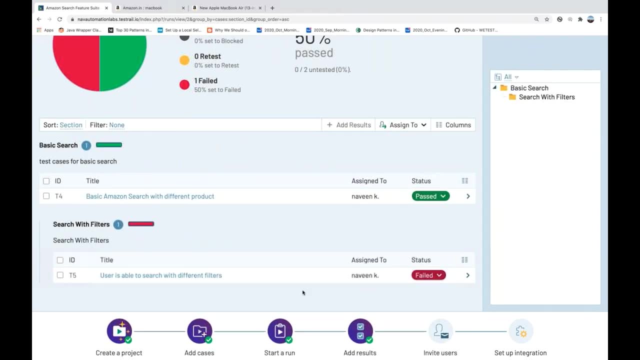 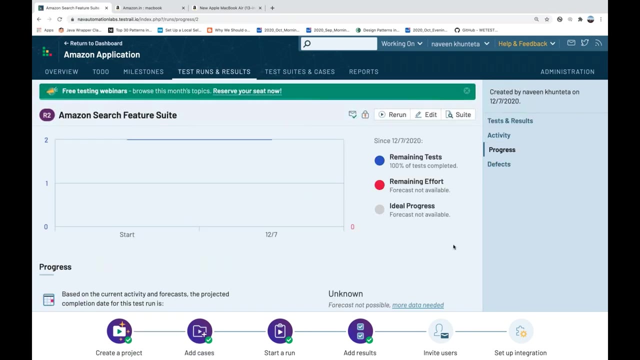 everything you can calculate accordingly, you can see that, yeah, expected result: one got failed. you go back this and then, this way, you see that, okay, yeah, 50 got passed just because of this thing. one got failed, like that. so this is the overall result. then, uh, you can see the progress. you click on this progress and then you will see that, uh, 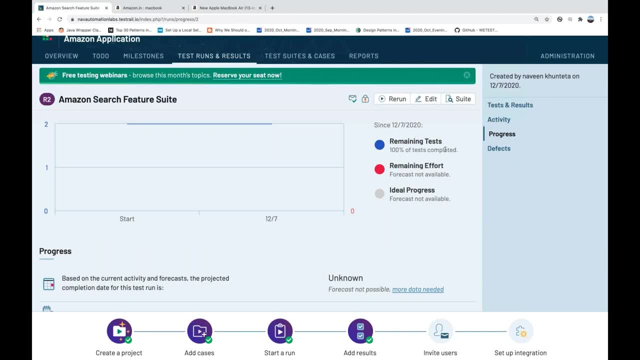 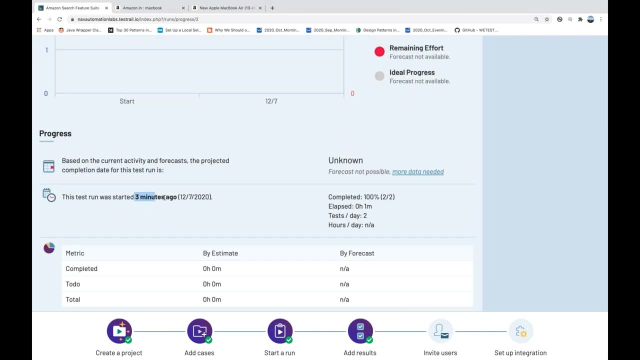 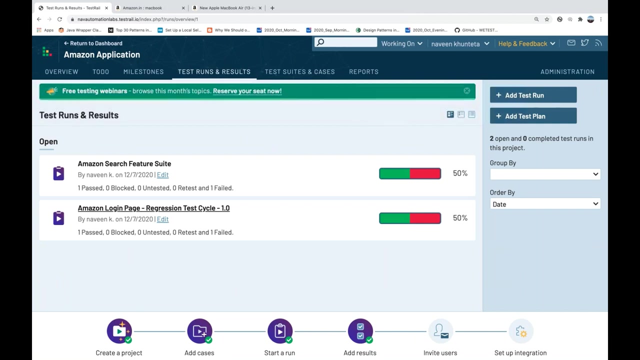 remaining effort forces. no, uh forecast not available. 100 test completed over here and and uh, yeah, so this test actually started three minutes ago, completed and left time. it took around one minute like this, so it will calculate the data accordingly or time accordingly. perfect again. go back to your test runs and result and in the test cycle number two, if you really 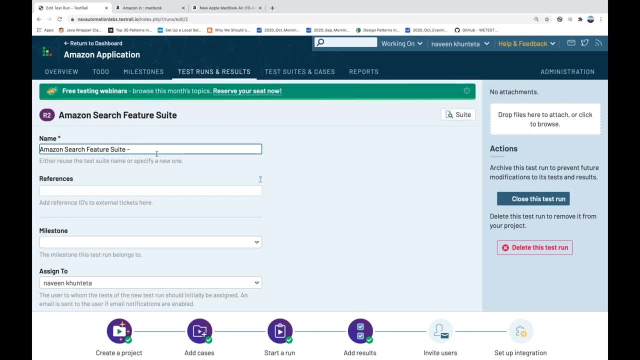 want to add it, let's add it over here. that is my. let's see, this is not a regression. we're just going to check test only, search feature suite. so instead of calling good regression cycle, let's see, this is my uh sprint number. uh, five is going on, so sprint five. 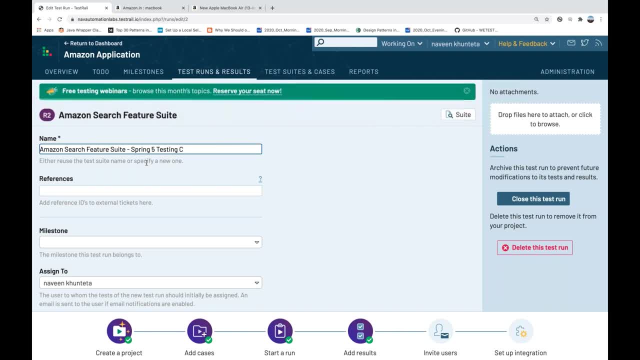 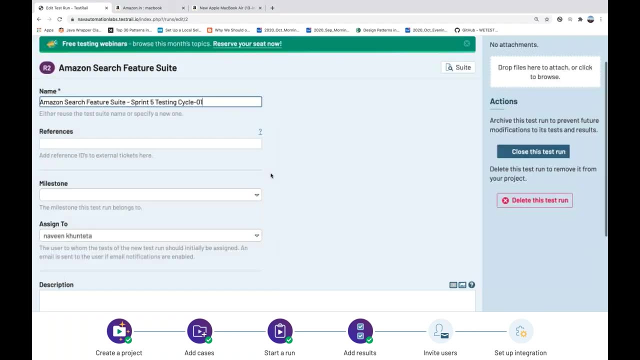 testing cycle that we have created. so i simply say that this is my sprint five testing cycle and, and by the possible in the same sprint, you might be using a couple of uh cycles. so let's say this is a sprint, the first cycle over here, like this zero one, so you can do it and then you simple save it. 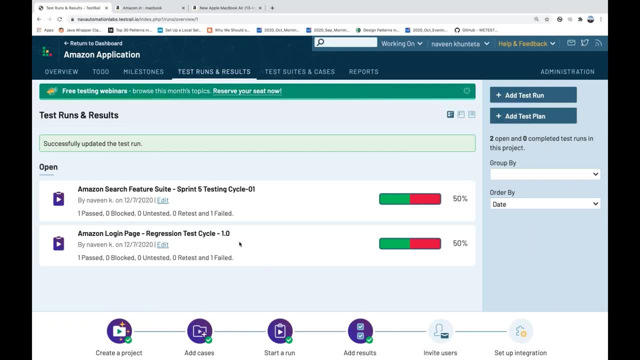 with this name. that looks more proper, because last time we executed with the complete regression. this time we are going to execute with the sprint five testing cycle, zero one, and this is the current status. now let's see the same cycle. we want to in the within the same cycle. let's see some test case. 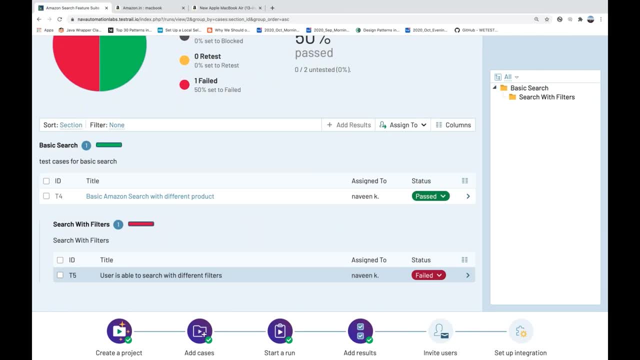 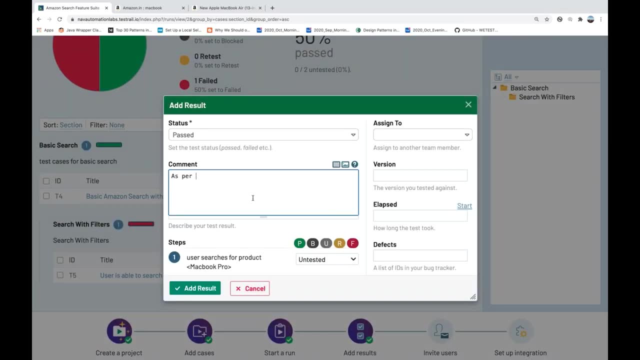 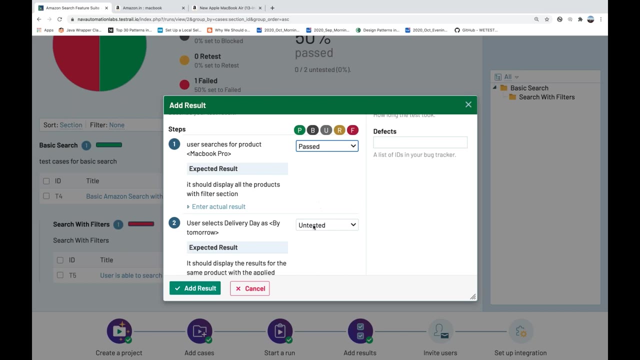 fixed, the failure test is working fine, the build is available once again, and what we have to do this time is getting passed. i make it pass over here and i simply say that, okay, yeah, as per expected it's. let's see it's working fine now, and then all other steps are getting passed. this is also 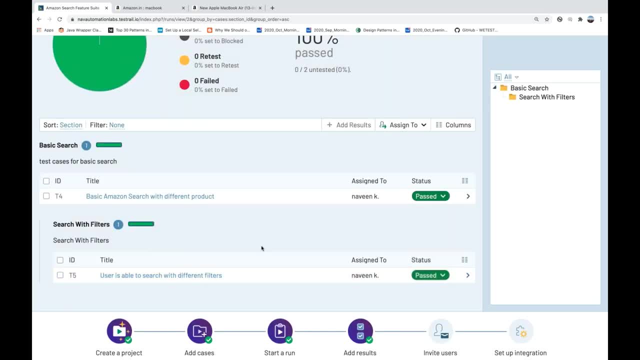 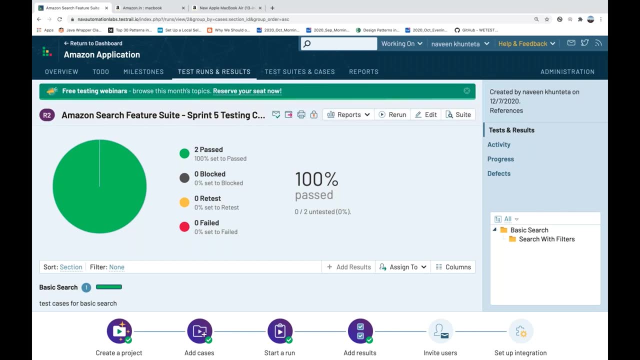 getting passed and you simple add the result, and this time in the cycle two, i mean this within the same cycle in the next iteration. it got passed over here, so you can check. it's absolutely fine. now okay, go back to the result, and this time you can see, so you can maintain a complete. 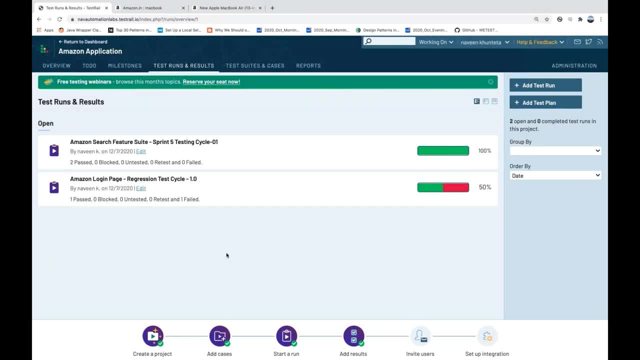 dashboard kind of thing over here, and then, uh, you can see all the different cycles, your regression cycle, your feature cycle, your sprint cycles, and you can maintain like that: okay, now different plans also, you can do that, let's see, you are, uh, different test plans you want to do, let's for. 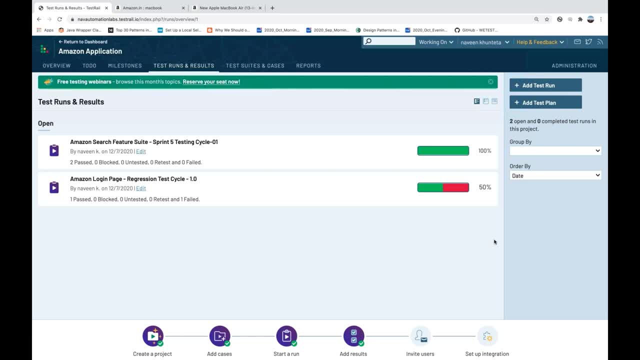 example, it's a cross browser testing i want to do. i want to do: let's see a performance testing or security testing for that particular feature, so you can click on that and then you can see the test plan and then you can create, add a test plan also. so just click on add test plan. what is the 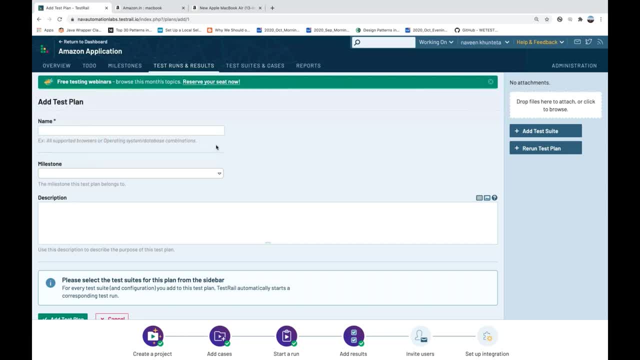 name so you can see this example. example, like all supported browser or operating system database combinations i want to test. so this is a test plan i want to create and then i'll be associating our different test cases over here. so i simply create. let's see, this is my uh cross, a browser. 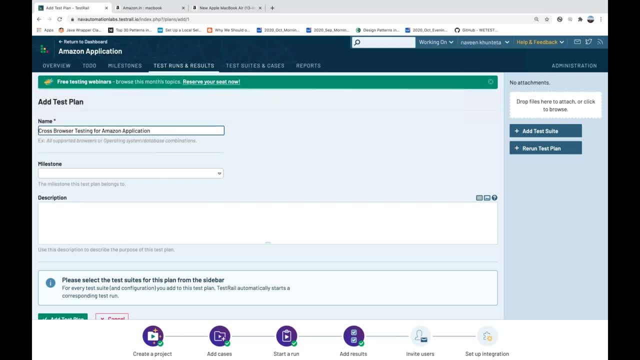 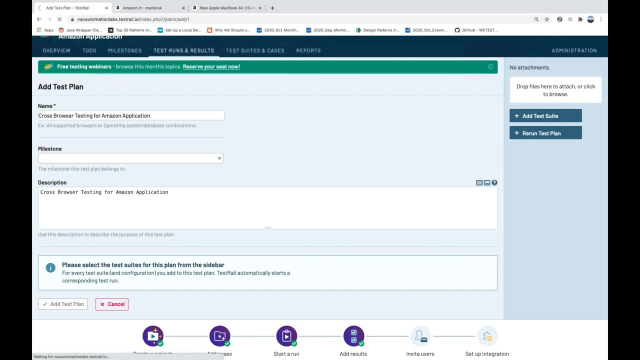 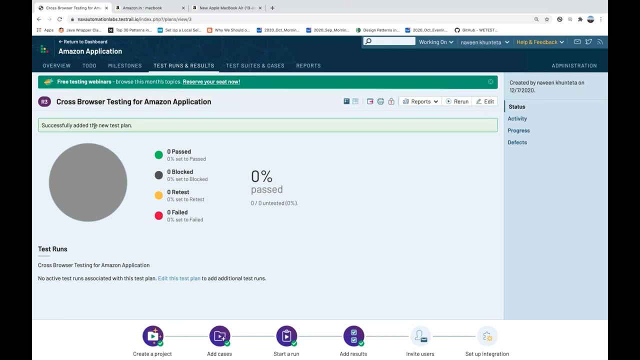 uh, testing for amazon application right and description. also, i'll be writing the same thing over here so i can just click on add a test plan over here. so you will see that, okay, the plan got added, you can edit the plan and you can see this successfully. edit the test plan over here. 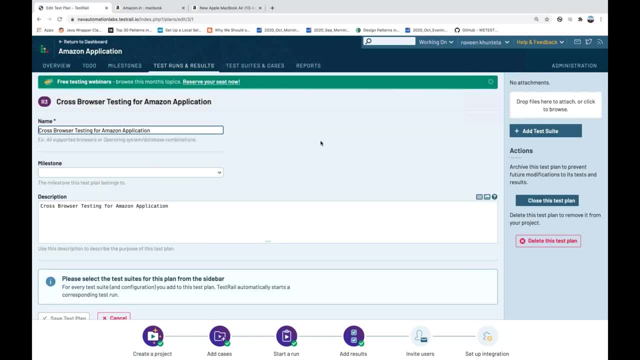 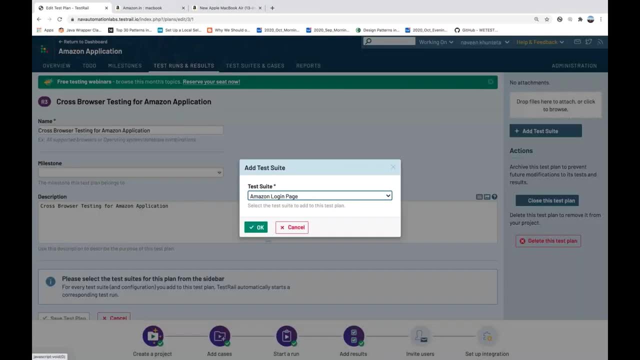 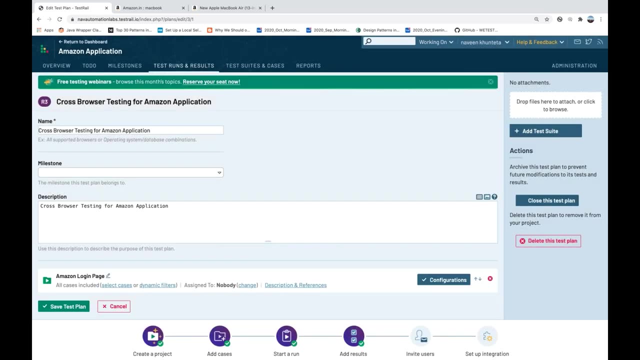 right, and if you click on edit once again, you can add it and you can add your test suites now in that particular plan. so, uh, click on this particular ad suite and which suite that you want to add. so let's see, i want to add my login page and click on okay. 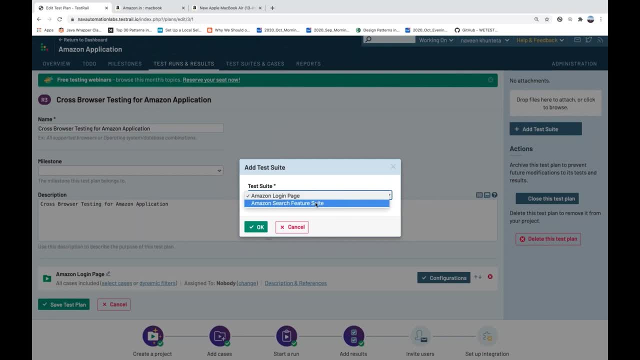 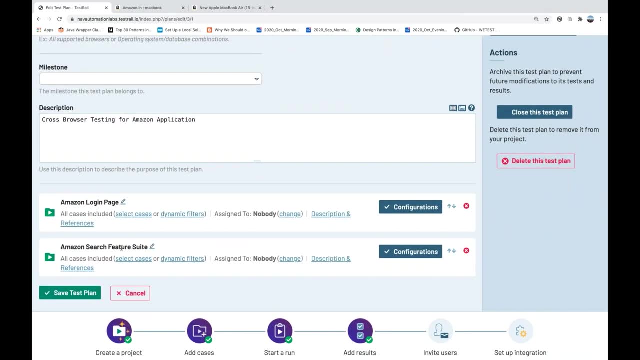 perfect and again i'm going to add the second suite once again feature, that is, the search feature. click on- ok, you see that, okay, both the login page suite and amazon search feature suite also got added over here- and click on this particular save test right and yeah. 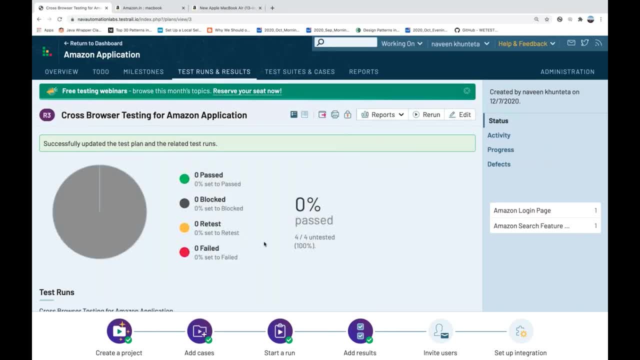 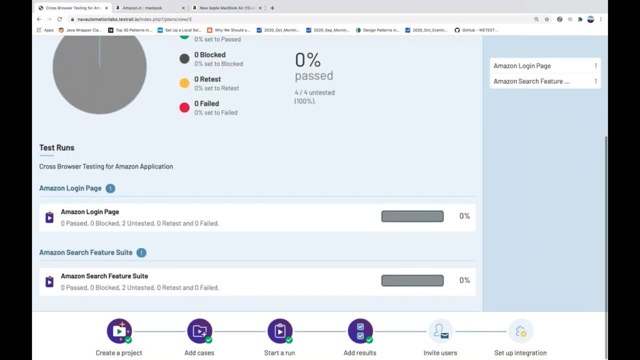 we are adding these two guys. click on ok, perfect, it got added. so my test plan is that cross browser testing for amazon application. i want to test it on multiple browsers, something like this, so we'll don't need to create multiple test cases again and again for the different browsers. and now you can. 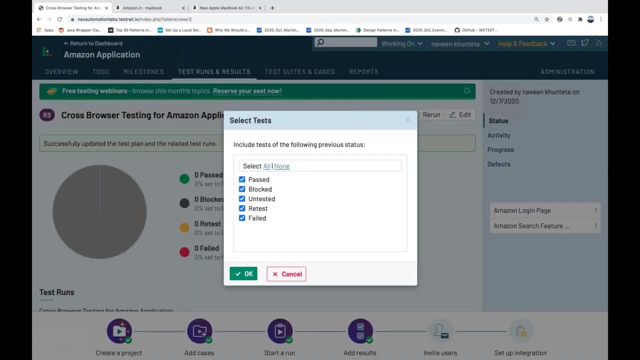 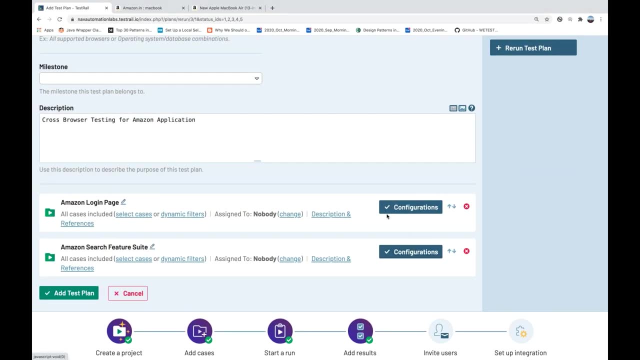 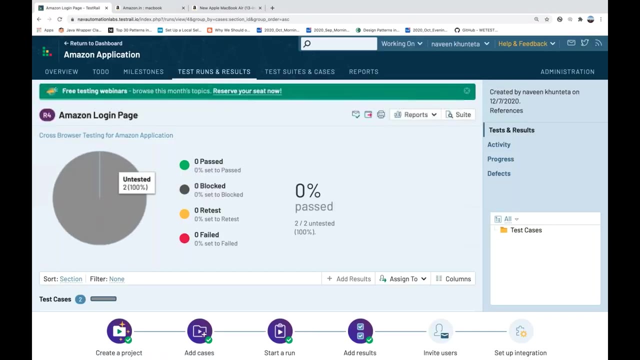 start executing your test cases. click on rerun and then you can simply click on ok and then you can start reading over here. so let's uh do one thing: uh, plan got added, okay, and uh, let's click on this individual test over here and now click on this particular pass. you can add your steps over here. 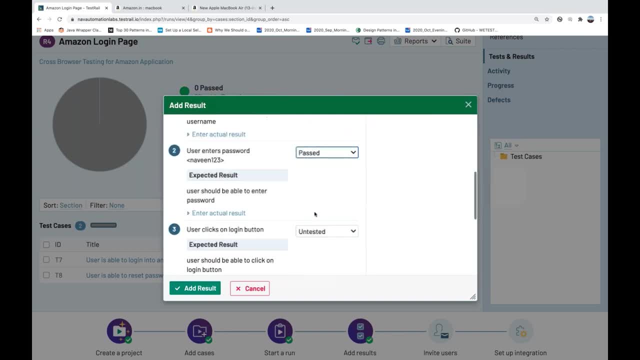 individual test. you can mark it. steps, you can mark it pass fail or pass fail, whatever. let's see everything is getting passed for different browsers and you can put a note over here: uh, test it for a chrome, firefox, internet explorer and safari, like this, let's say randomly, i'm just simple writing these: uh, four browsers. 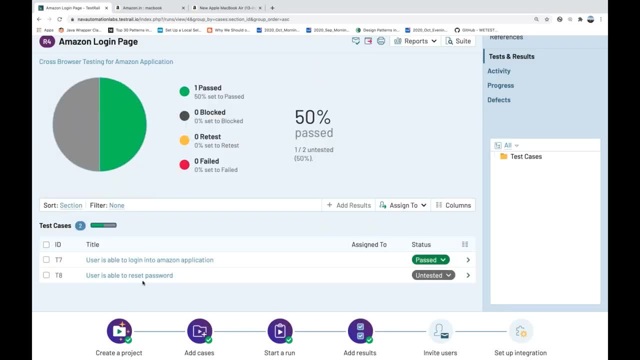 i'm using it and simple add the result. same thing: user is able to reset the password is working on. okay for all the browsers. i simply put a comment over here, add the result and then we are good to go. so this is perfectly fine, that crossbar testing for amazon application. 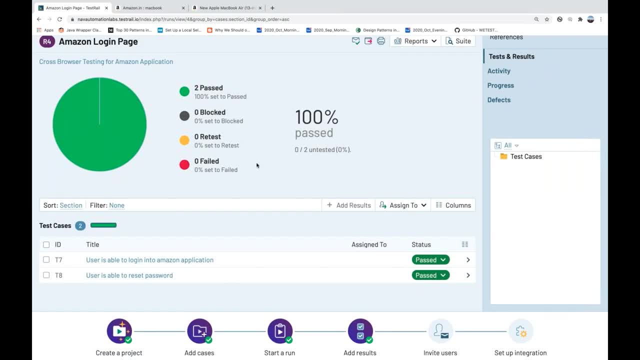 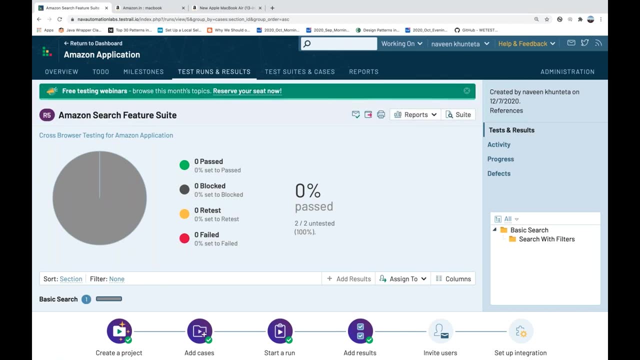 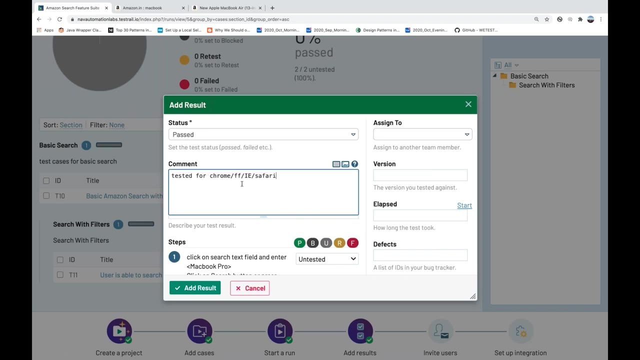 the login page got passed without any problem. again, i click on this particular test plan and then we have one more uh test suite. click on this particular test suite guys. you have to click on it and then you have to execute test cases. click on pass again. are tested for these. 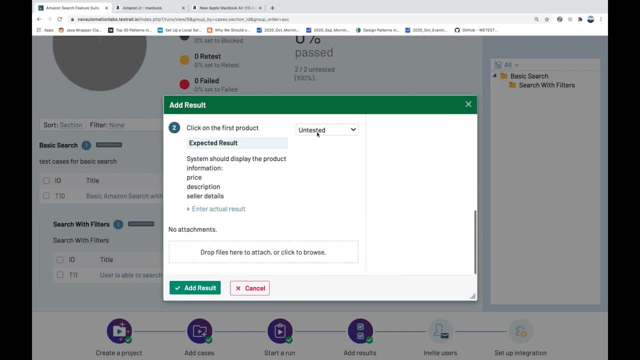 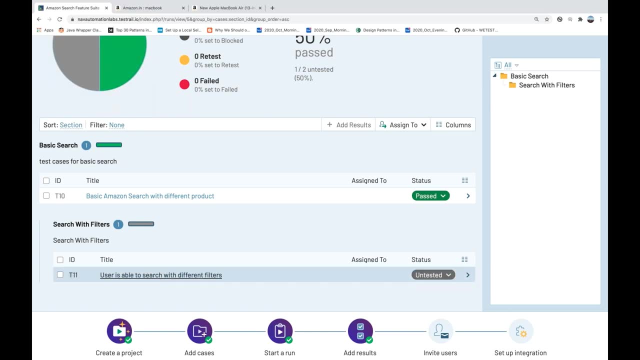 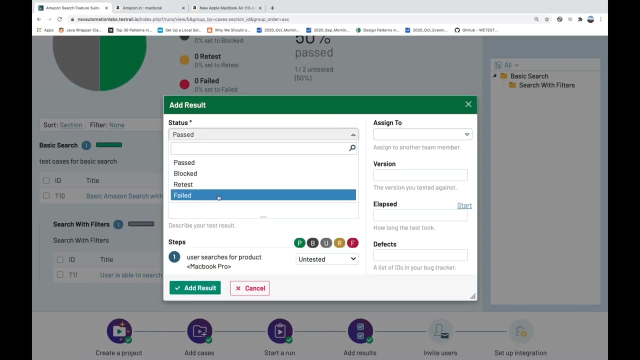 browsers. everything is getting passed. and click on the first product, this is also getting passed. and click on add. the result: perfect, same thing. user is able to search with different filters on different browsers. again, let's see, this time this is, uh, getting failed. assume that, okay, we are. 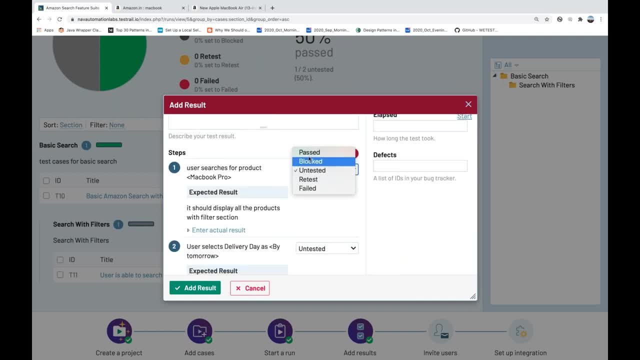 testing on this and we are just clicking on this. uh, let's see, this is a god pass. but the second one got failed over here and uh, it's saying you can write the individual actual results all the ways. so what is the result over here? so let's say i'm writing, this is aspx. 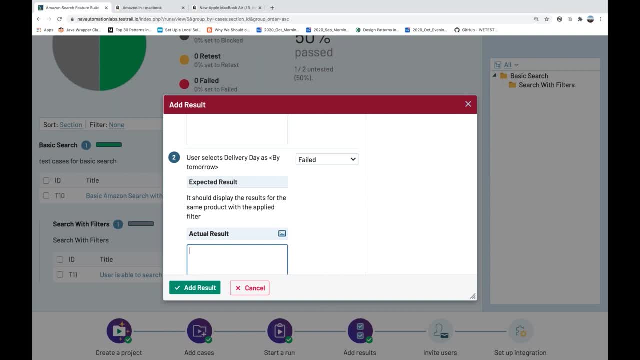 were expected. but let's see when we apply the filter, i simply say that okay, filter is not working. firefox browser: let's see, there is a bug in the firefox right, only for that particular step i make it fail. and if you have any defect you have to gonna raise it. you can put a defect over here. 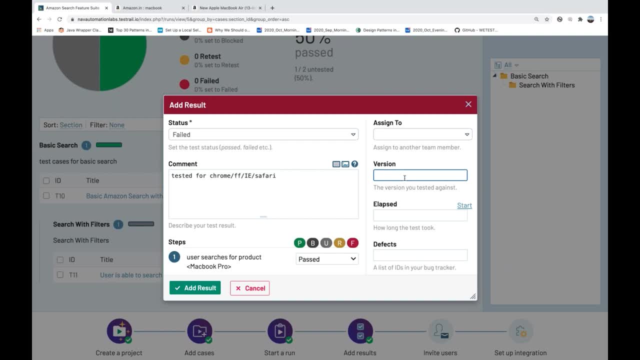 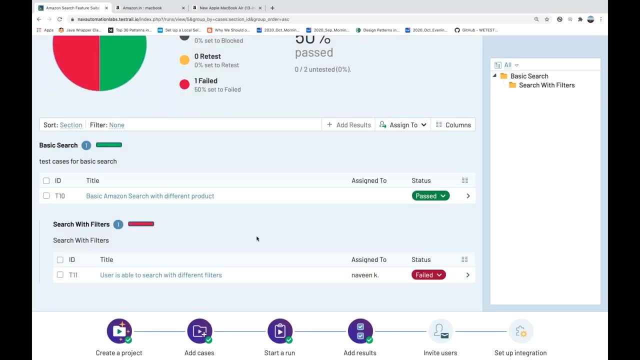 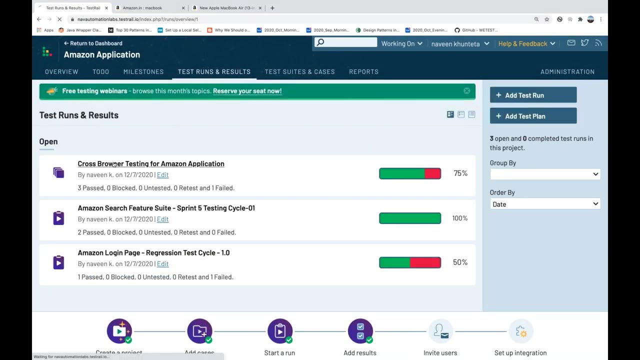 like that, the version you tested against. let's say i'm writing 1.0 version assigned to whom? assigned to? let's see to me, navin, and then click on add result. it got failed like that, perfect. you go back to your results and here you see that, okay, this is my. 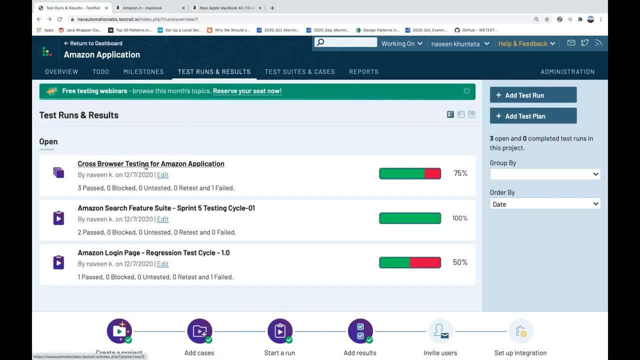 test. see, i'll go back once again. this is the test plan, actually, and these are my cycles. these are my test runner cycles, guys. that's why you can see that, okay, these are my runner cycles and these are my test plan, so you can create multiple plans, okay, for the different types. 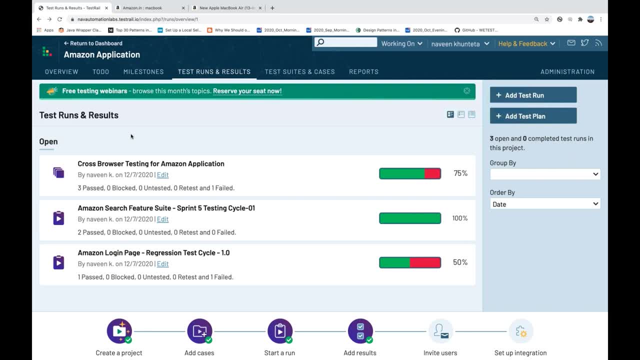 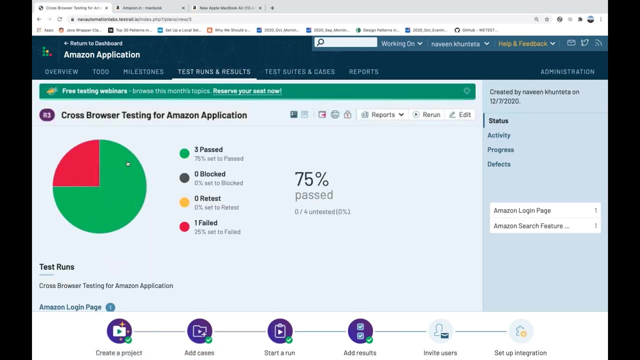 of testing. or you want to do performance testing, you want to do a complete regression, or um, uh, uh, or maybe database testing or maybe security testing or some database validation specific for specific test suite or test cases. you want to add that also. you can do that and then you can check the status. 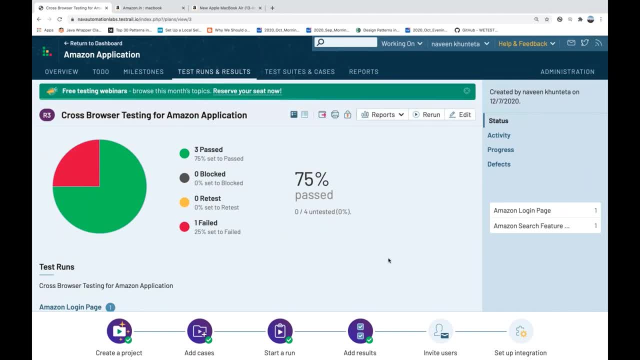 So it will be really good for the PO, developers, everyone and manual testers and automation guys that, yeah, this is a current result. That is what we are getting amazingly good right. It's very dry stool and a lot of companies are using it as plan. 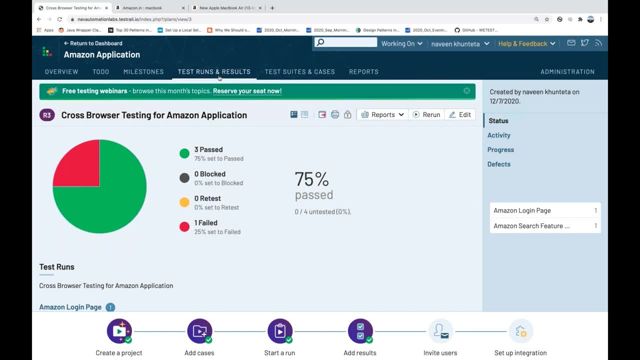 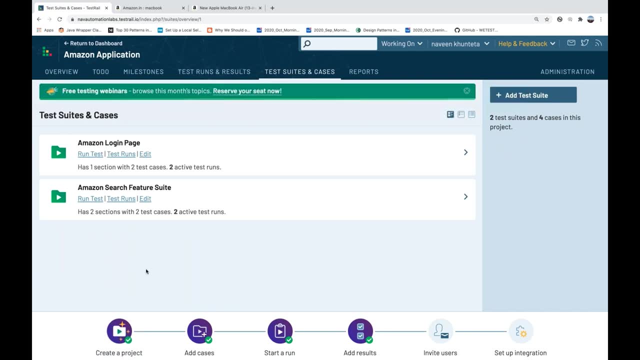 So make sure that, okay, you guys are used to with these things. Now go back to this particular test suite and cases. once again, if you really want to add some more test suites, you can add it. if you really want to update the existing one, 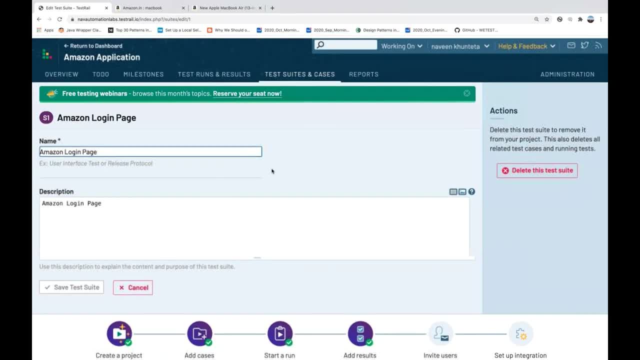 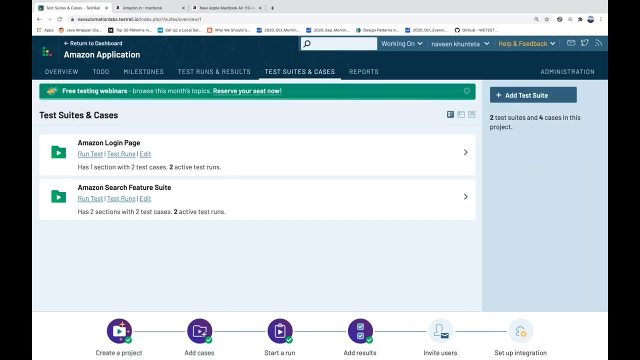 Let's see on the login page, Some other features also got added, So you can again add some more and more test. You can delete the test also. So I'll do one thing: Let me just cancel this and let's go to this particular Amazon. this: 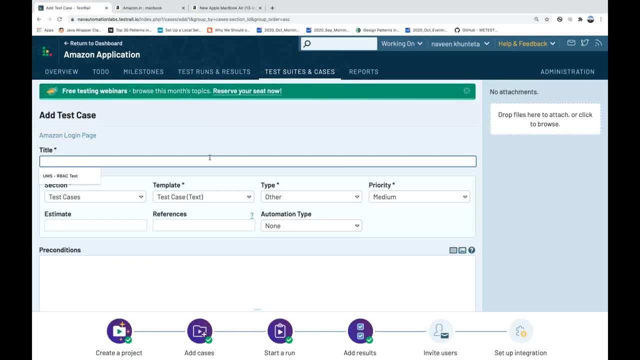 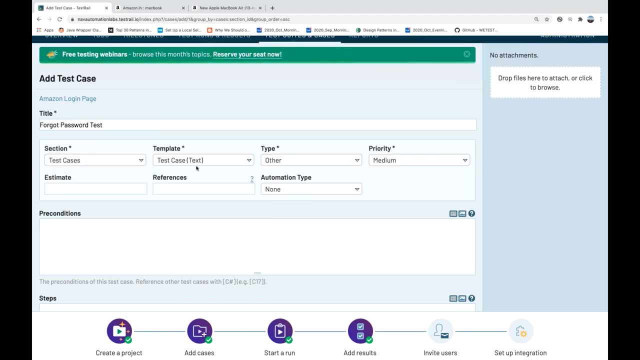 if you really want to add some more test cases, let's see forgot password got added by simple right. that okay, forgot Like this. This is a quick section, the test case section, and I want to use let's see test case as a step or text. 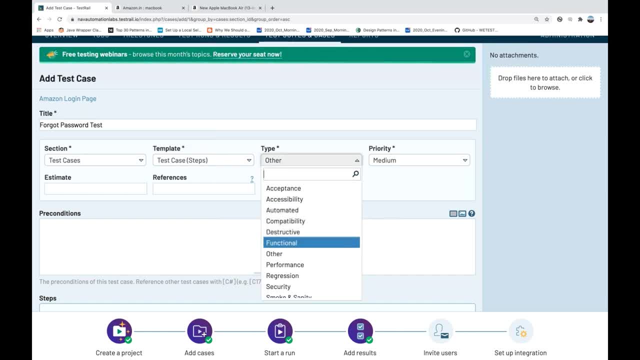 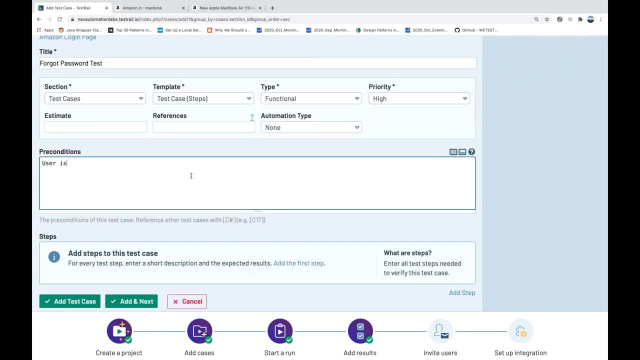 Let's see as a step and what type of feature. it's: a functional type. The priority is again high priority and simple write it and I simple write it. Okay, user should be and I'm going to write some step over here, So click on add step. 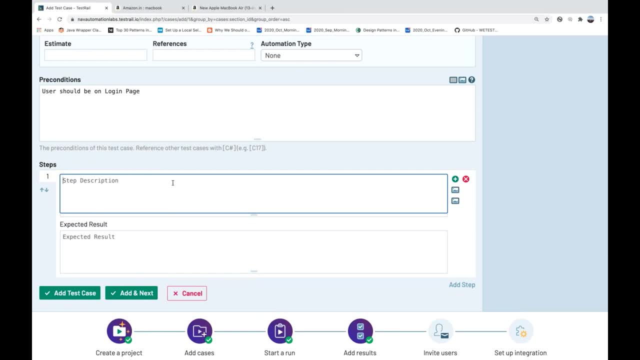 and I simple write a simple basic description that first step over here. user, not step. Sorry, I'm not. definitely a description, It's a proper step. So user clicks on forgot password, a link. This is my first step and user should be able to navigate a page. 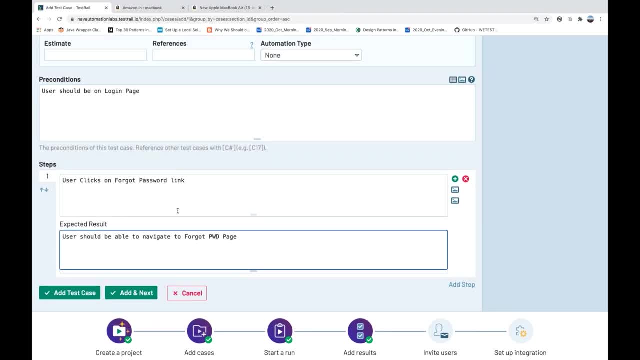 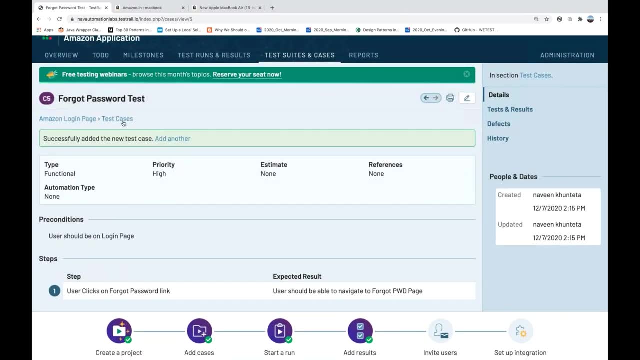 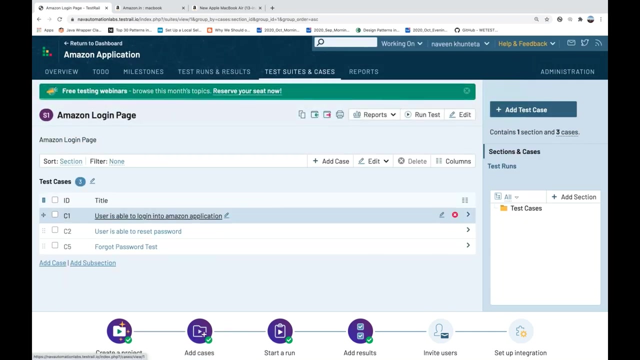 over here something like this: Okay, user clicks on forgot password link and then that's it. So click on add test over here got added. only one step right, So I'll do one thing. Let me go to click on test cases. This is got added. forgot password test got added. 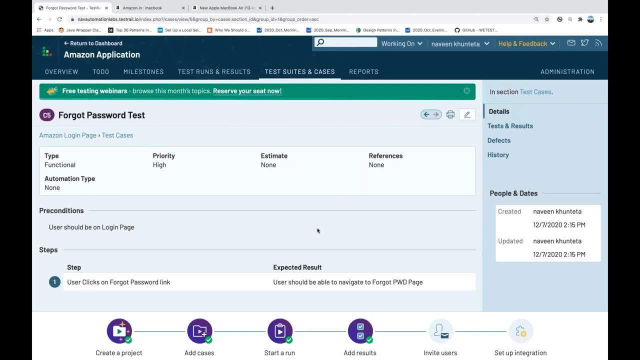 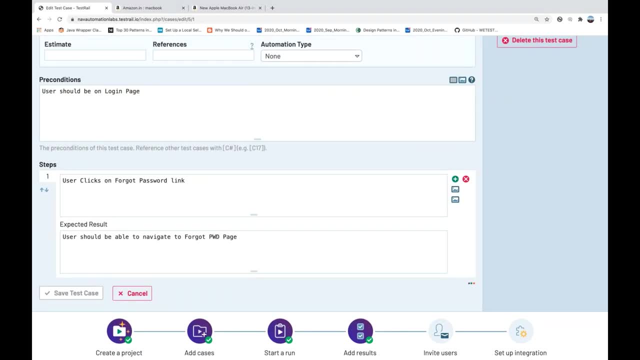 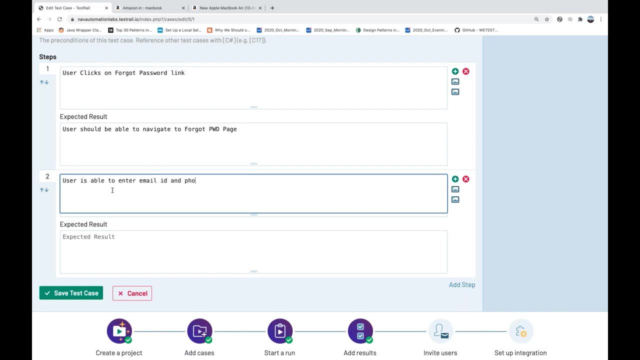 I want to see this thing, perfectly fine, Okay, and I just click on add it once again. I want to add some more steps over here, So click on add step and the next one is: let's see, I just have to enter my email ID and phone number. 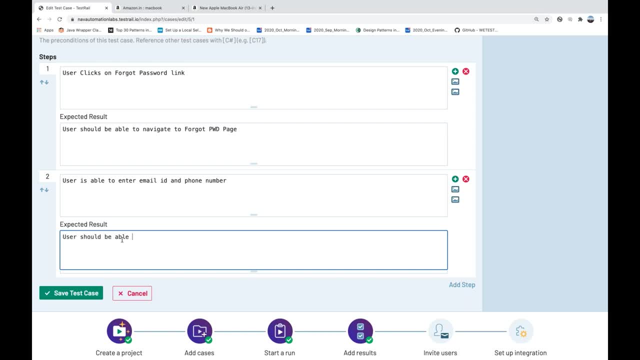 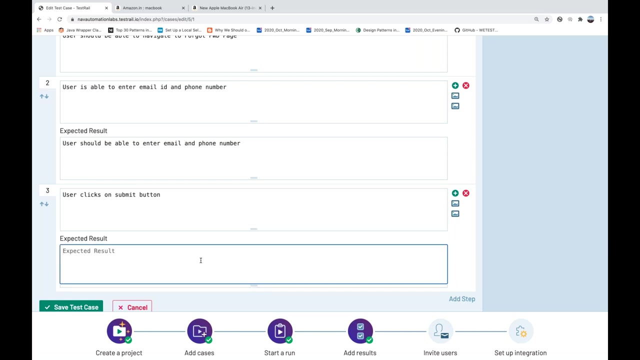 and I simple say that okay, Yeah, user should be able to enter email and a phone Number like that. This is my second step And the third step is that user let's see There is a submit button which will okay use when you use a clicks on submit button. 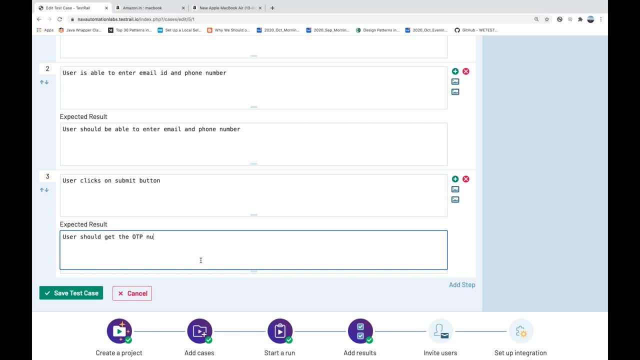 Then what happens? then? it should OTP number to change the password, or let's see OTP number, or a temporary password, I simple right- and or phone number. I would say something like this: Whatever, the feature is accordingly designed like that, Okay, Okay, at this step. 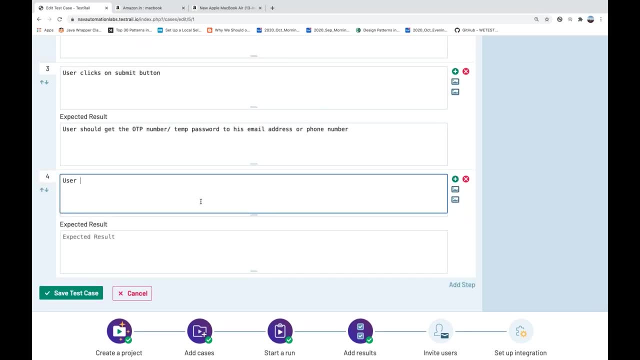 Over here. and then I want to write my final step: that user OTP, perfect. So the step is that user is able to change the password using OTP and this is the last step. or maybe we can add one more step: that okay, user is. user enters the new password. 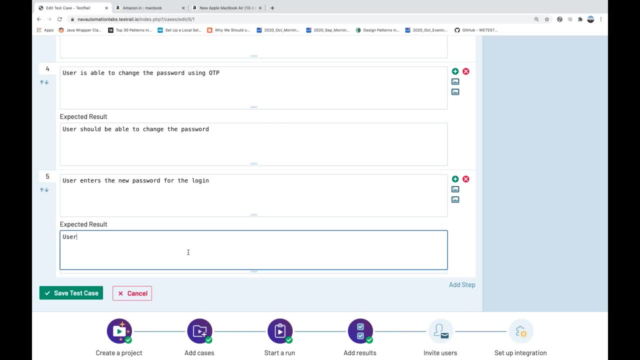 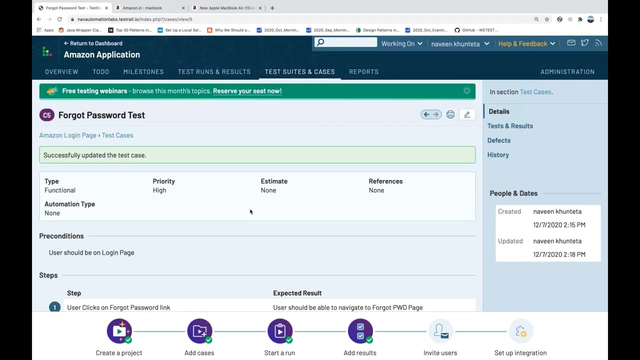 For the login and I simply write that user is able to log into Amazon application and then user should be able to see the home page like that. So this is the two expected result we have written, and now the save the test. this particular test is having five steps over here. 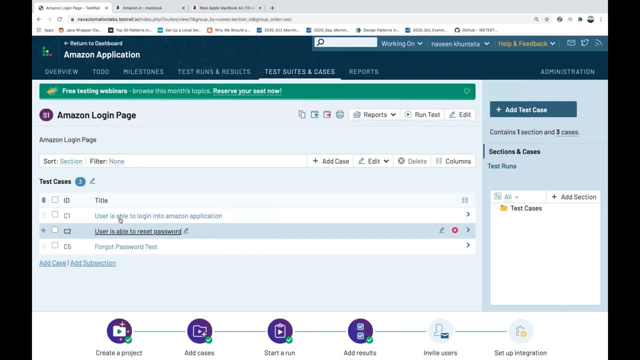 Okay, so in Amazon login page we have actually now three test cases and every test will have the respective test ID over here. See once you do see three like this. If you really want to add some more subsections, you can do that. 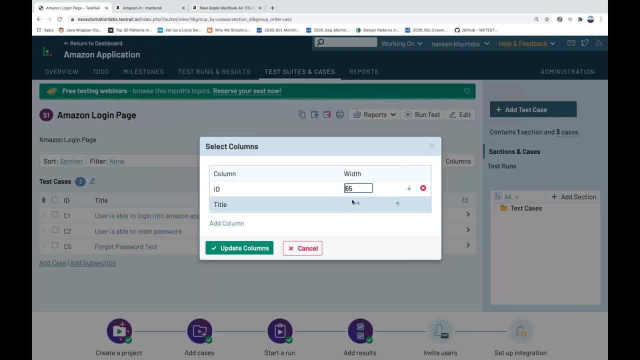 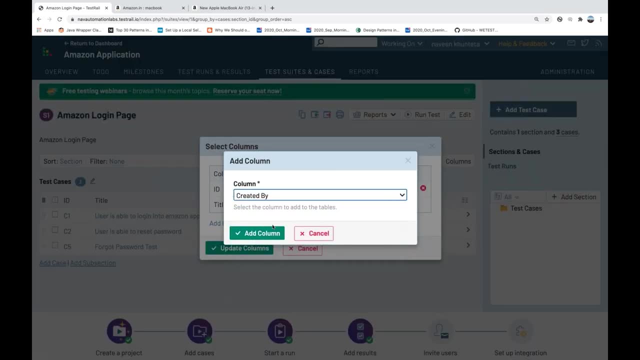 You can edit it. You can add some more columns over here. Okay, the width of the ID. you can do that. You want to add some more columns? that automation type- who created actually like this? You can add this particular column. click on update the column created by my. okay, by Nabeen. 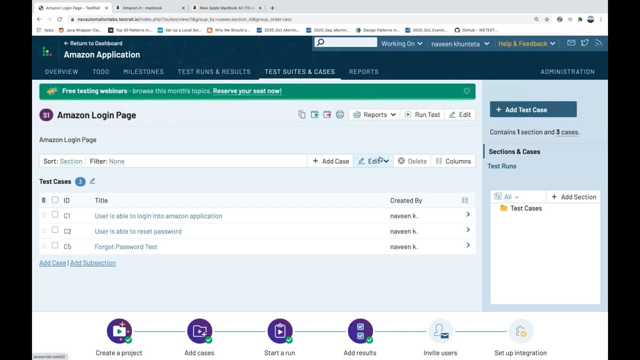 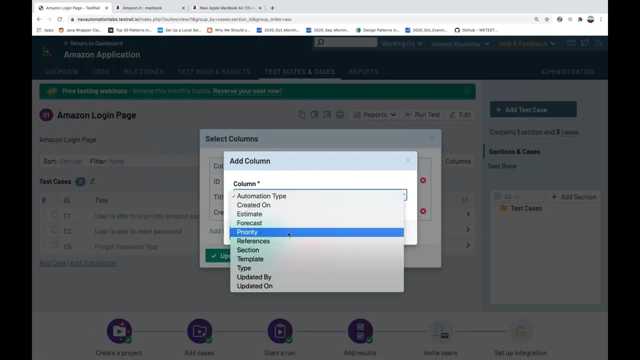 So you will get to know that. okay, Yeah, who is the creator of this guy? We really want to add some more columns, So simply click on add column and then let's see what is a priority, if you have given add the column, and then 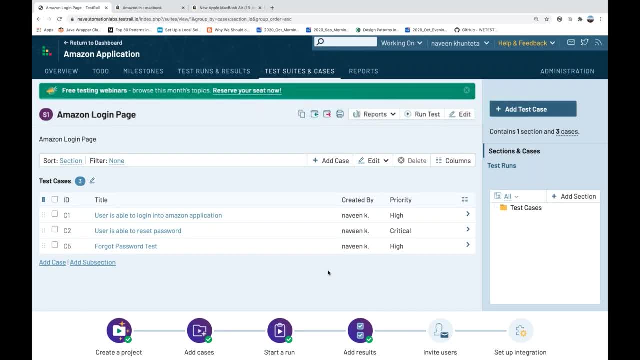 Update the column. So we have given high critical, high priority, like that right. This is what generally follow in the okay, in the, in the excel sheet, Also in quality center. Also let's see. Let's see What are different columns are available. click on add column. 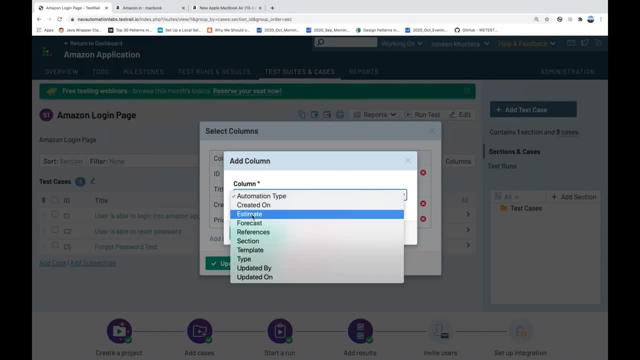 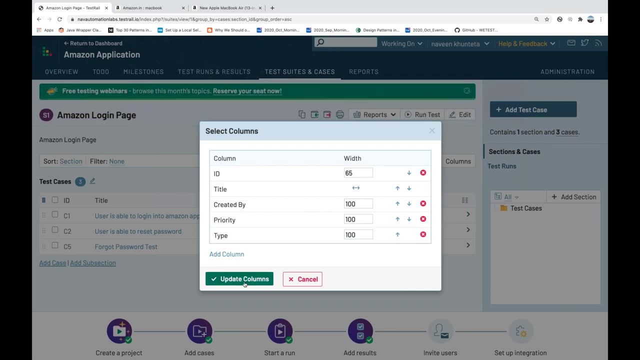 and then updated by type: template section: forecast estimate- Also created on date. Also updated on all those things. What type of test cases? days? all these are functional test cases. According to me, you can design the width over here How many characters. 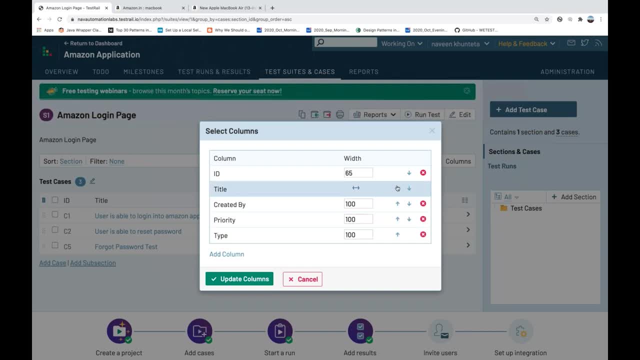 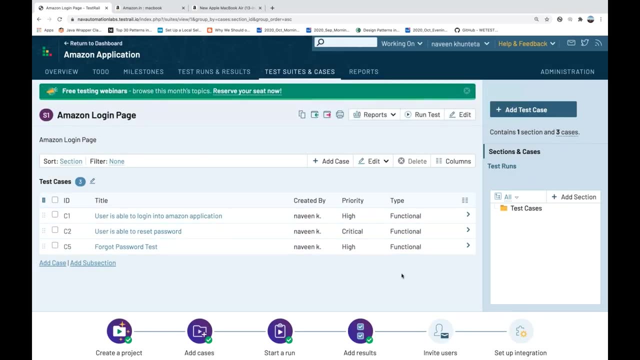 It will take like this, and you can change the order also with these arrows. You can do that, So click on update the column. You can see all these are functional level test cases over here. This is what, guys, you can do. This is a designing part. 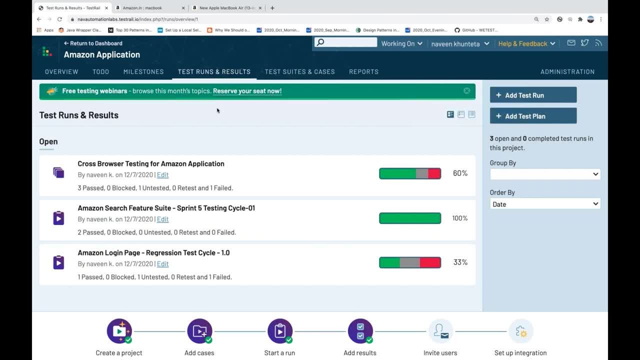 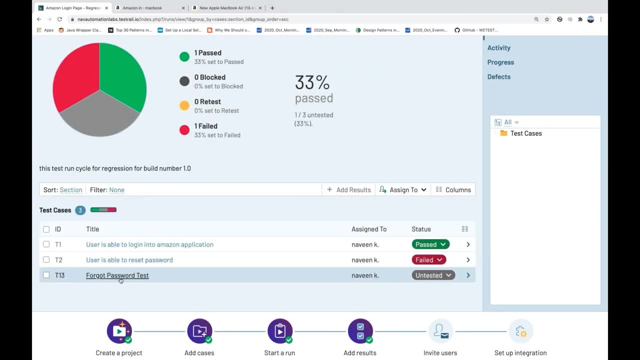 and this is a runner part where you execute your test cases like that. Okay, Now I'll go to my regression cycle 1.0.. Once again, I'll see over here that, okay, the forgot password also got added, which is actually untested. 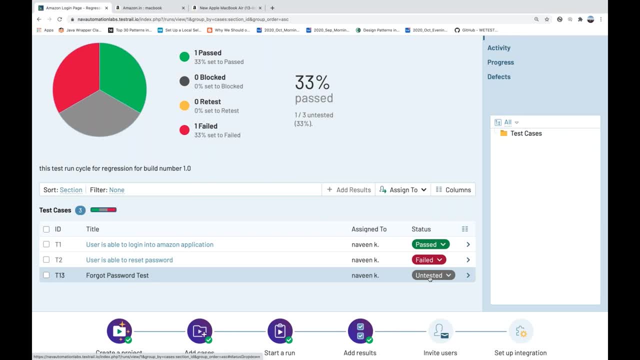 because this is a new feature that we have added. So whenever there is a new feature and now let's see the build is ready for the, for the production, So what we have to do instead of updating over here, because you never know, because while adding, while adding this feature, 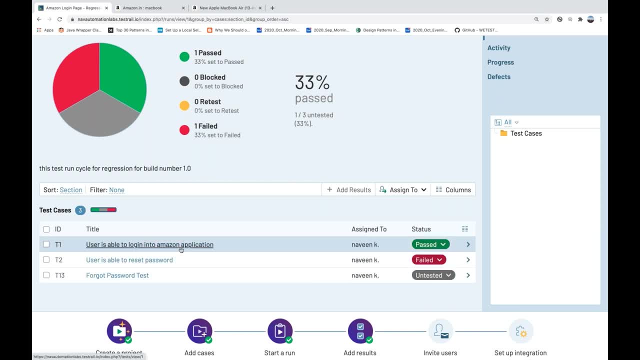 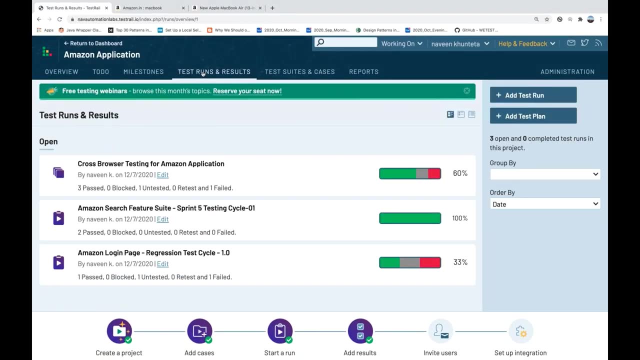 forgot password might be possible. that, okay, the login and the reset password got changed. You never know. So, in that case, what we have to do, we have to create a new cycle all the time. So whenever new features or maybe a new release, we are going to do, okay, deliver. 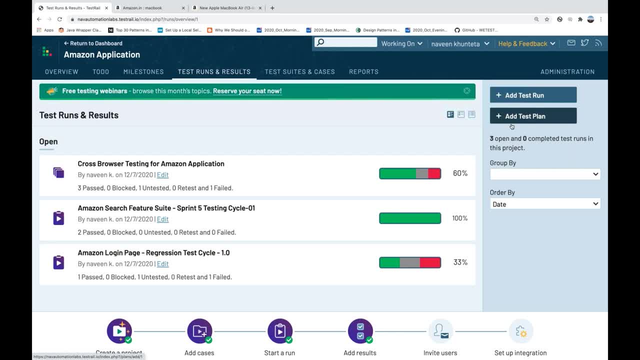 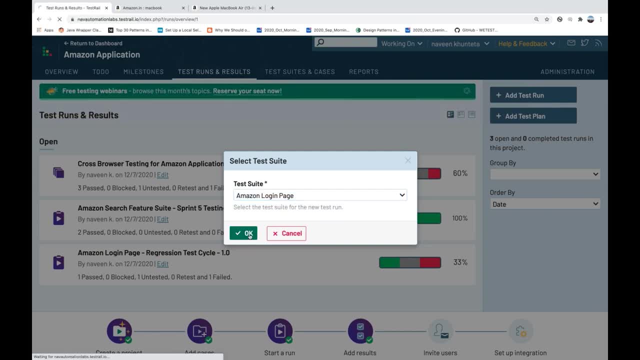 So once in a sprint we should have at least one regression cycle. So what I'm going to do, I'm going to add a test run over here and this time I'm going to add: let's see first login page, click on: Okay, it got added over here. 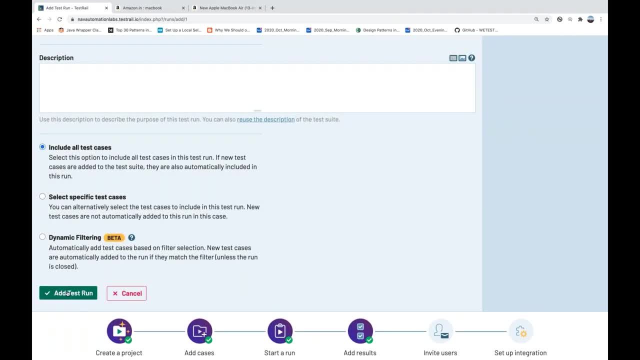 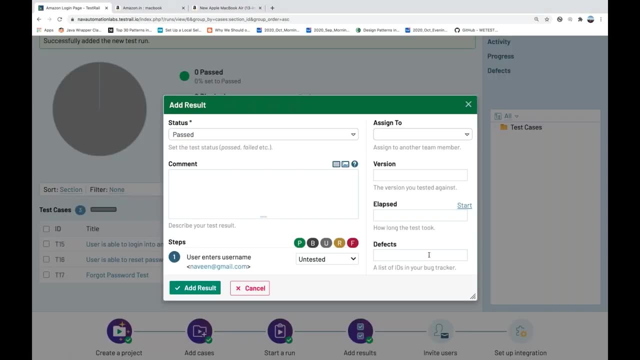 I simply say that include all the test cases, right, and I can simple forgot password. I can test it Now. I click on. this is got passed and I make. everything got passed now, So let me write it. This is for the first time login with a different username. 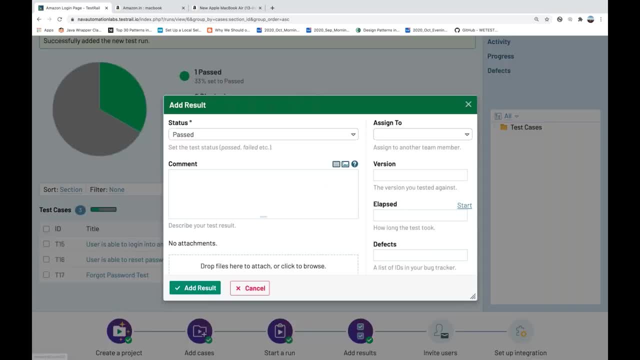 Let's see, Fine, Let's say password- I'm going to check this- is also got passed. So I'll say that, okay, Yeah, this is got passed, forgot password. Now I'm going to test it and I simple say yeah. 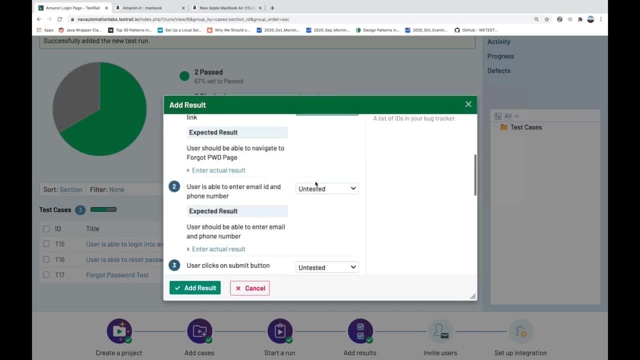 this is also got passed. click on forgot password link: Perfect, This is getting passed and I can write individual result Also like as: but this is fine. It's okay to write guys as per expected, Otherwise it will very time-taking. It will be very time-taking that you are writing. 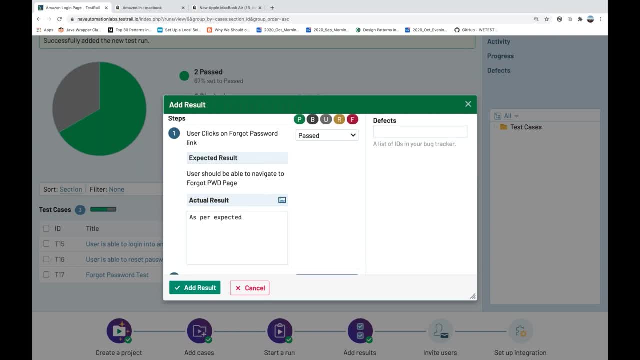 Yeah, user is able to see the forgot password link and user is able to do that for each and everything. If you're writing actual result, that is again time-taking, so you can write as per expected, whatever you are expecting. as for expected some managers, they oppose this, or you know. 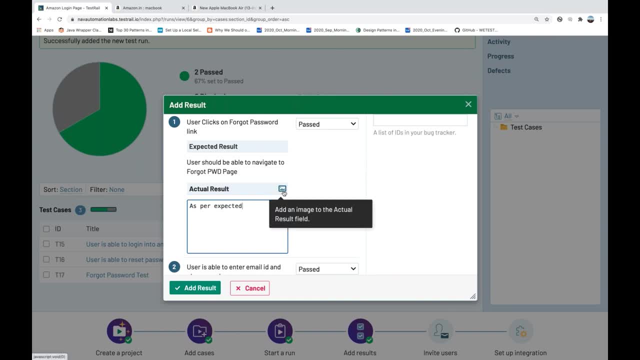 you have to write what exactly is happening and then you have to put a screenshot over here. But again, that is very time-taking. So running the cycle you should take care about you know what kind of actual versus expected result that you are writing, and it's not compulsory that okay. 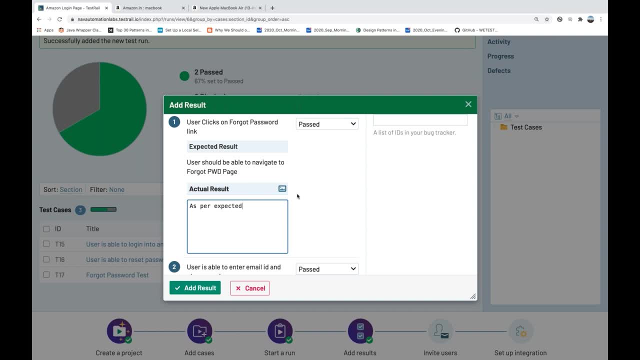 you are writing too much amount of information about each and every step. Otherwise it will take a lot of time to execute thousand test cases, or if you have 500 test cases like that, Okay, so let's see a simple. generally I put: follow, follow. 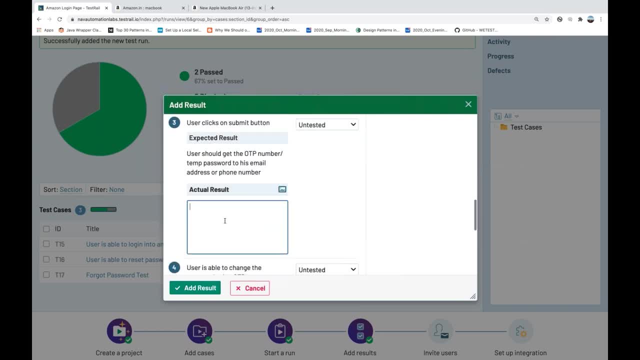 as per expected and actual result also as per expected and this is passed and user is able to change the password using OTP. Yeah, this is also getting passed and the result is expected and the user enters new password for the login. This is absolutely fine and the actual result getting passed. 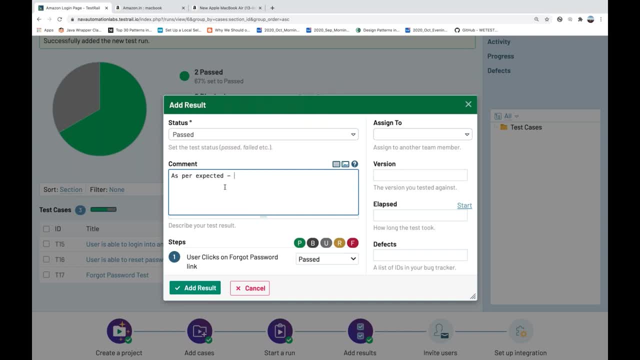 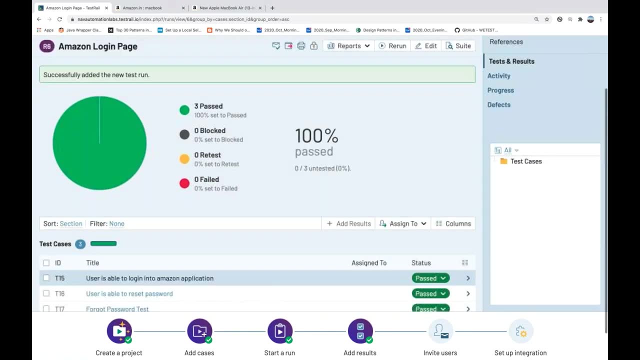 and overall everything is fine. You can write as per expected: Okay, something like this: You can write and then click on add result: So everything got passed over here. like this, here Also in the result. Also you can add multiple columns. 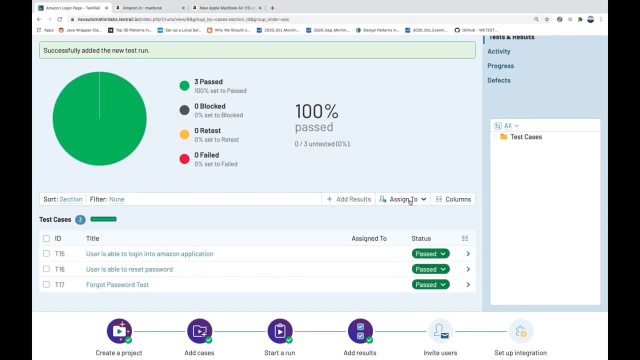 Okay, you can add multiple columns, You can assign to a specific person. Let's see, you can sort it on the basis of that. This is a sorting feature, you can sort it and when you running your test cases, that time also you can assign to someone. 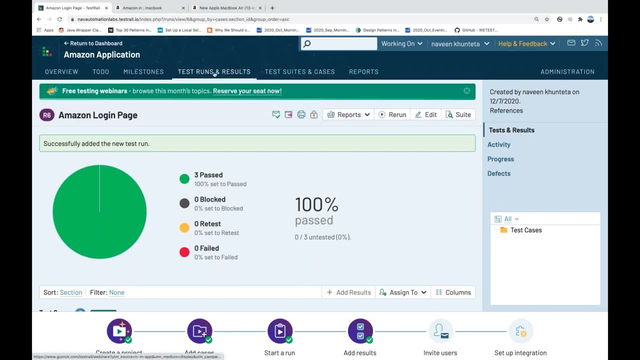 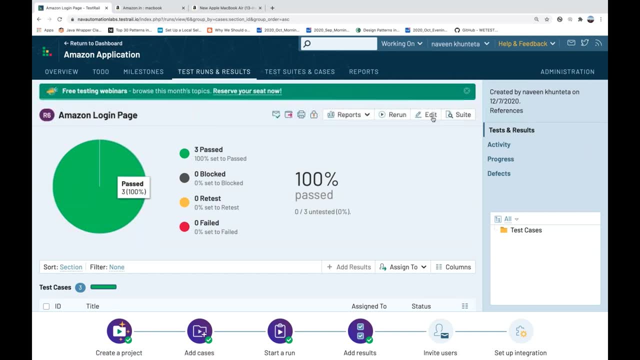 if you really want to read on, you can read on like that. Okay, And then let's go back to this and you can see that here. Amazon login page. Let me do one thing: just click on it and let me edit this name. Let's see this. Amazon login page. 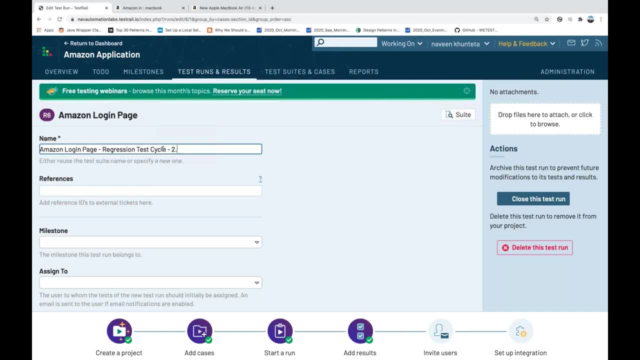 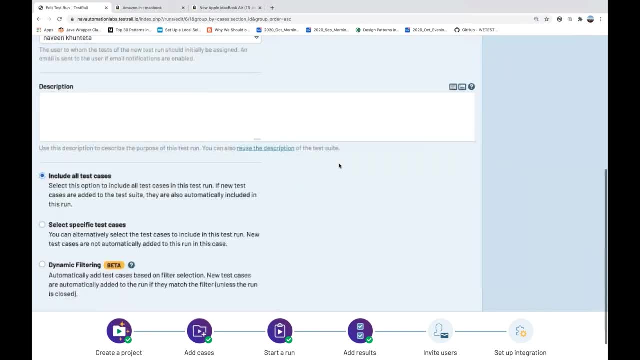 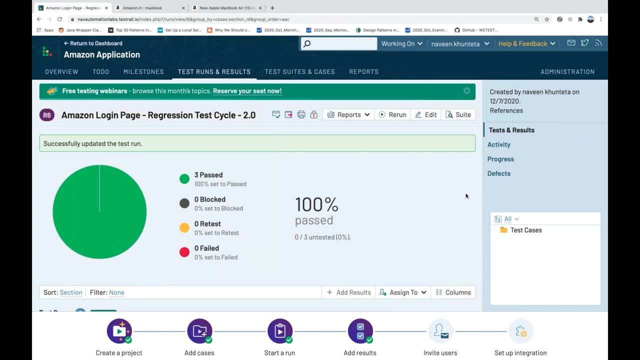 We actually tested for regression cycle number 2.0.. We did that, Okay, and it actually assigned to me. Let's see some kind of in and like this: Okay, So once save the test over here, It got passed with regression cycle 2.0. 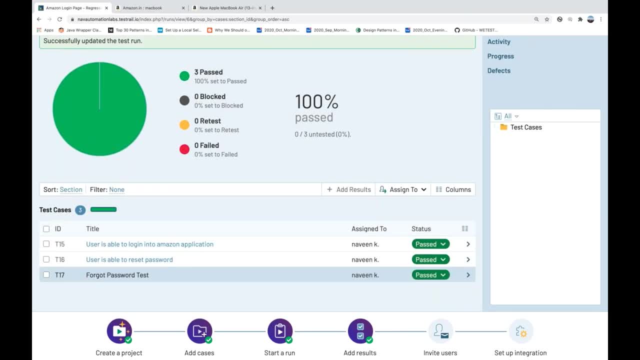 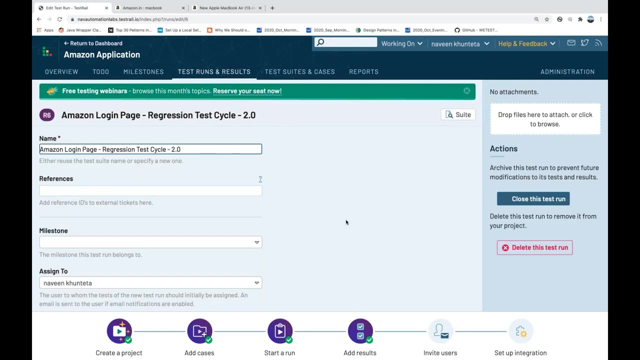 Let's see Right. So, like this, guys, you can add multiple test and execute multiple test cases over here. Now, one thing is that once you let the cycle is gone, I mean is absolutely fine, Protection release is also done. I want to close this particular run. 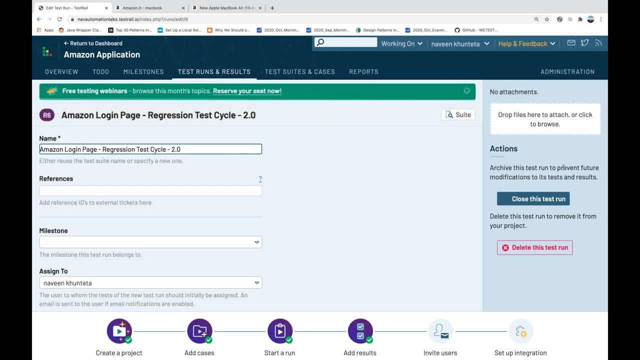 So it's important, guys, that this test run to prevent future modifications, so that nobody is going to change the this particular runner. Otherwise, what will happen? that, okay, mighty possible to get some other guy is making some test case fail and in the production you are getting some bugs. 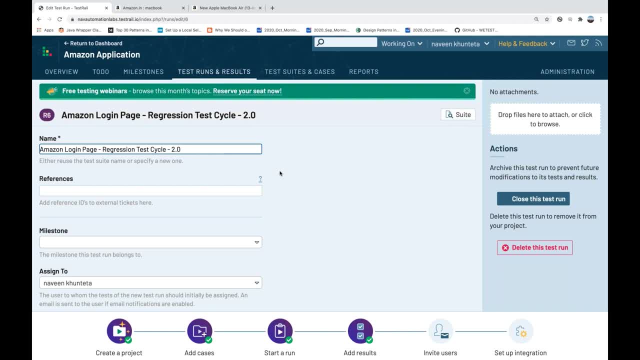 And then immediately a manager will see it. Okay, Hey, show me your results and then you can fight over there. that okay. No, my test case were absolutely fine. I don't know. some of someone has actually a mark them failed, So you should have some proof over here. 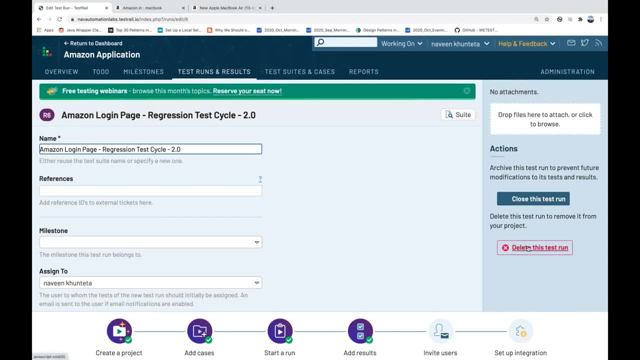 So best thing is that please close this run, don't delete this. please close this run for the future point of view, so that no one can modify. if you don't close It, people are still able to body find this, So just click on this and then yes. 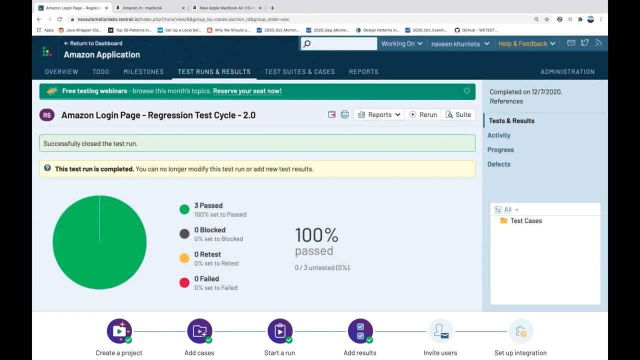 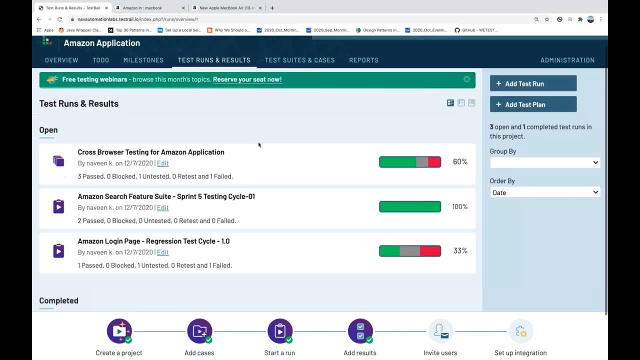 and then it's closed. now, perfectly fine, This is a final result: successfully closer test run. The test run is completely so. this feature is also very important, right? Let's see you. the spin 5 is still going on. assume that. so in the sprint 5 you are doing multiple iterations. 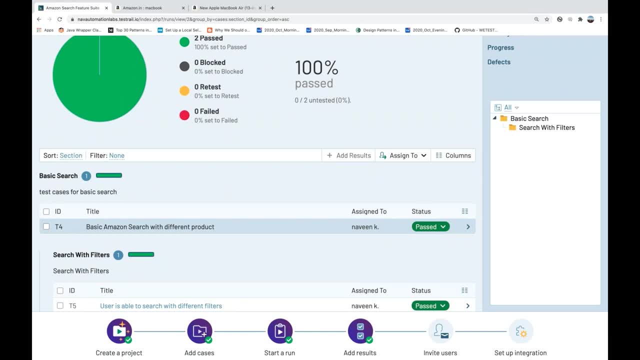 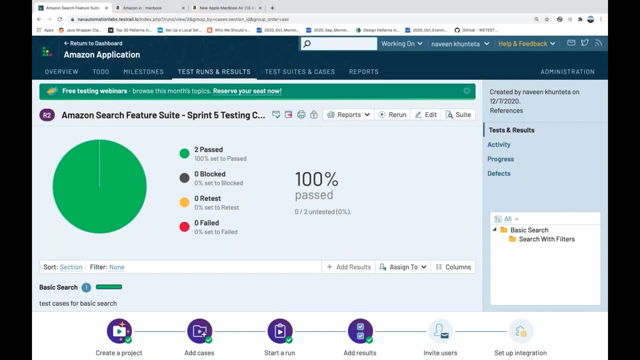 Today also your testing. tomorrow also testing three, four days multiple times. We have tested it so you can change the status. you can change or update the status accordingly Multiple times within the same cycle. You don't need to create one more test cycle or test run cycle over there. 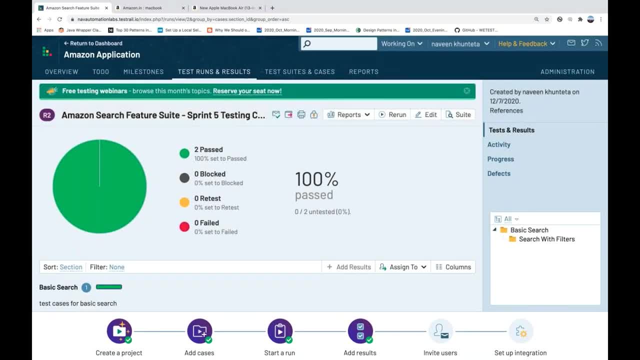 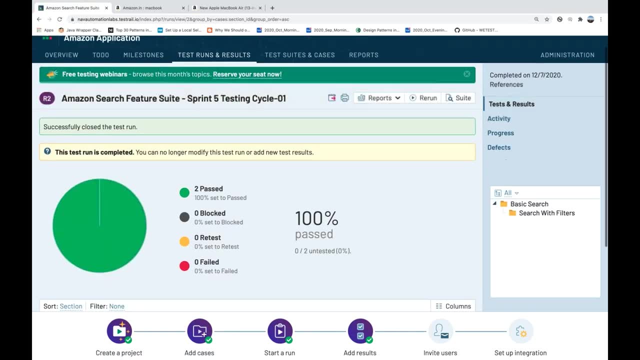 Once everything is done, then later on you can close that particular cycle. Okay, then you can close this. So moment I close it. Okay, Now no one can modify that, Let's close perfectly. Okay, if you really want to close it, let's see. 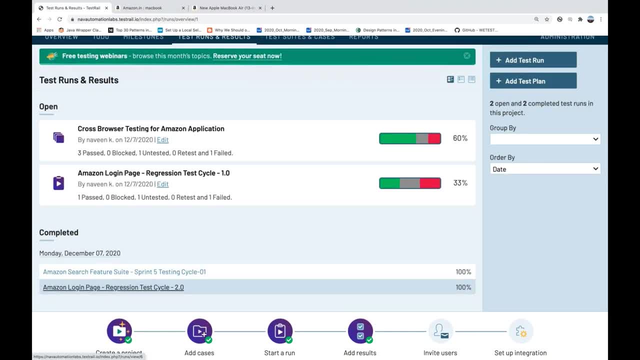 I just see it's close. It's going in the completed section over here And these are the open cycles. That's a good feature, that right, These are my close cycles. I can check the history from here, And these are the open cycles. 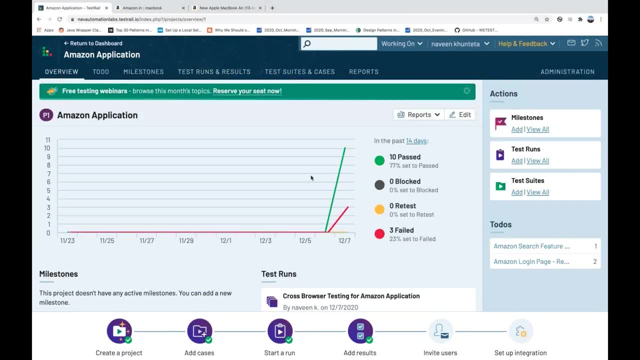 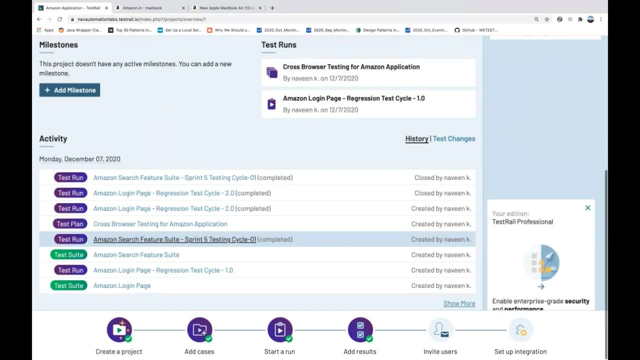 And then, guys, this is the overview dashboard. You will see that this is about your application. This is what is happening. These are the test runs. These are the current activities are going on. Okay, These are the test run that we have created. 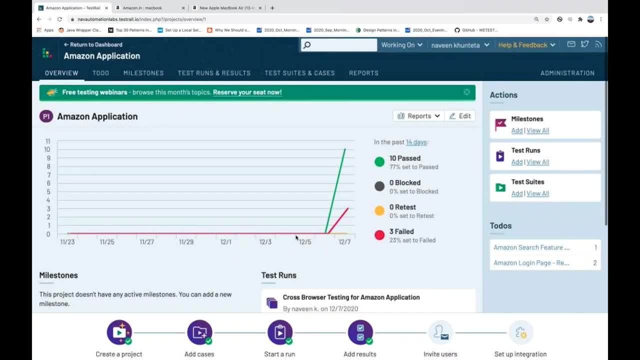 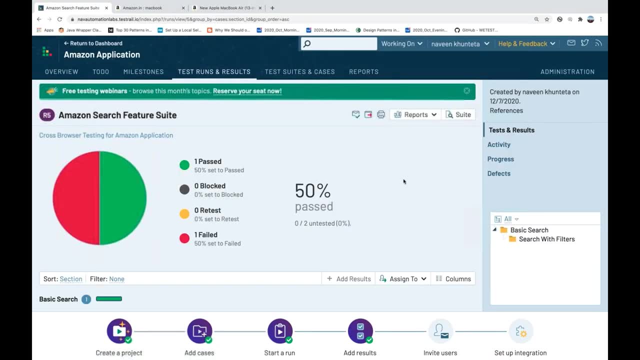 We have two test suites over here, So overall a dashboard also. you will be seeing over here like this: And these are the to-do's things It will show over here. Let's see what exactly saying: introduce. It's saying okay. 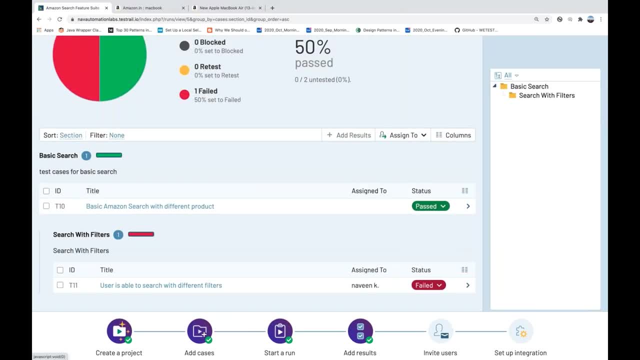 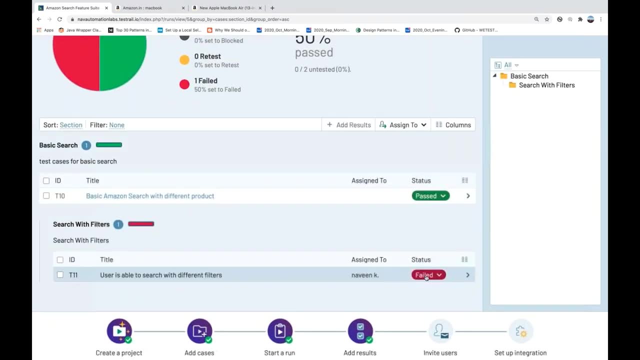 Yeah, you have two cycles which are not in the computer state. So let's see I'll just. if you really want to make them close, you can close that as well. Okay, let's see, This is still in fail. 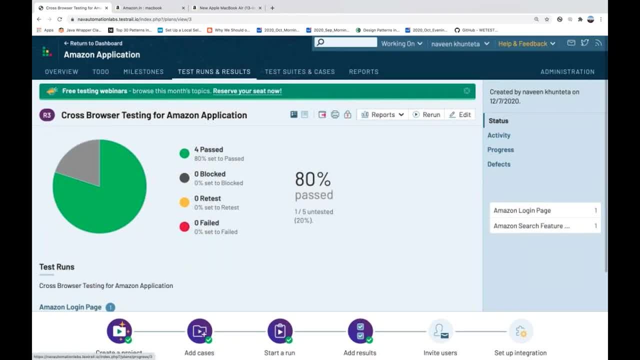 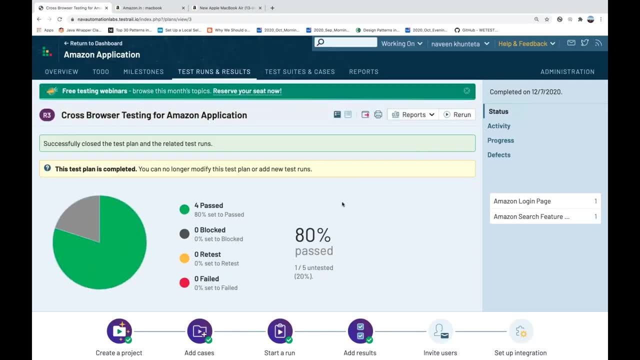 Let's see. I'll just make it pass. click on the result. Okay, if you add it, just close this test plan also. So test plan on. the same way you can close it. Let's see: cross-border testing is completed. It's closed like this. 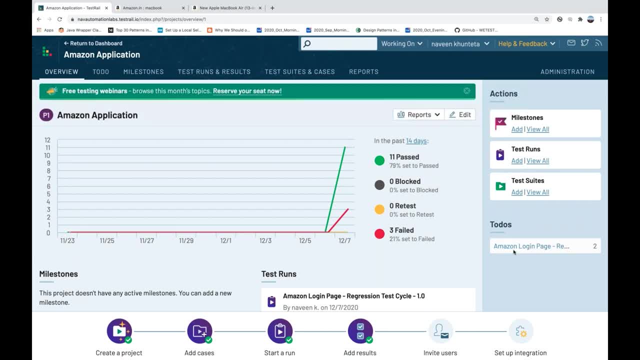 I'll go to my overview and now you see that. Okay, Now we have in the to-do's list only this particular cycle. That we can do it later, Okay, So if you really want to see all the test reads, all the test runs, all the different. 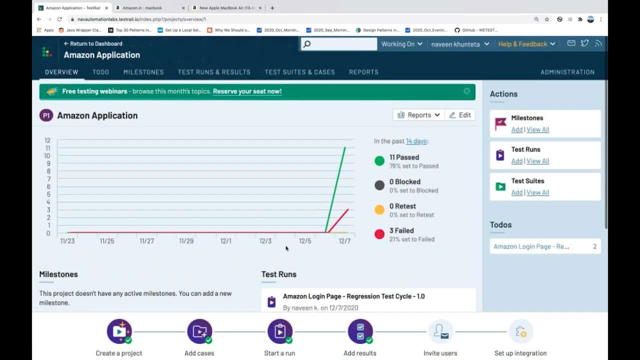 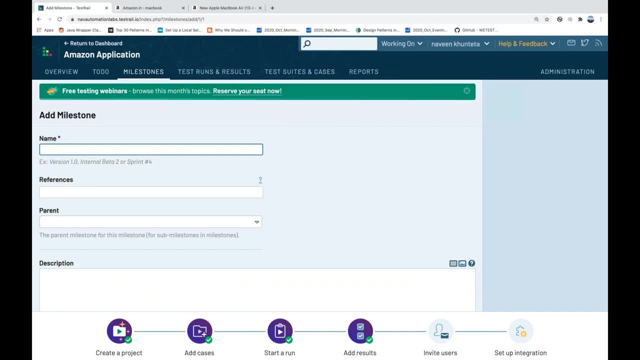 Milestone. you can check it over here like this: Now, if you really the project doesn't have any active Milestone, you can add a new Milestone. So let's add a Milestone now. So Milestone means let's see internal beta or Sprint 4 or version 1.0.. 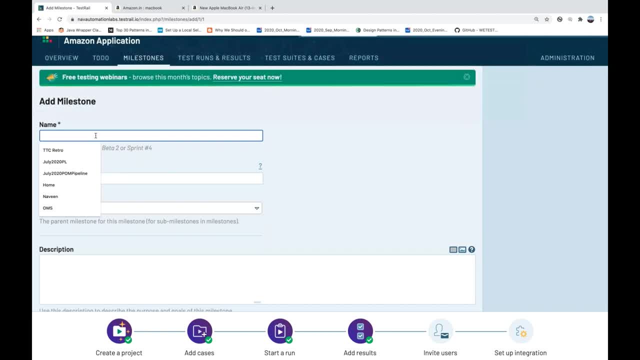 This is, this is what I want to achieve with this particular Milestone. So let's see- I simple say that a version, Or let's see some I would say beta release for Amazon like this, and which beta release? I would say beta 1.0 release. 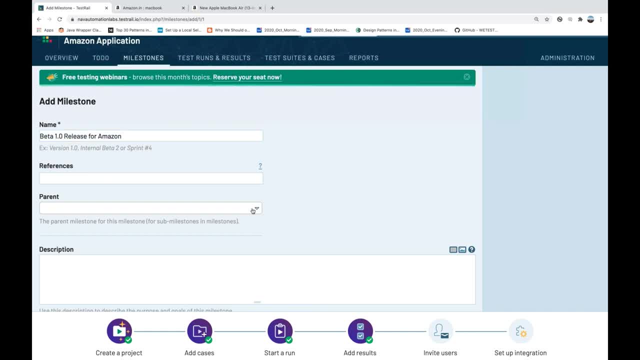 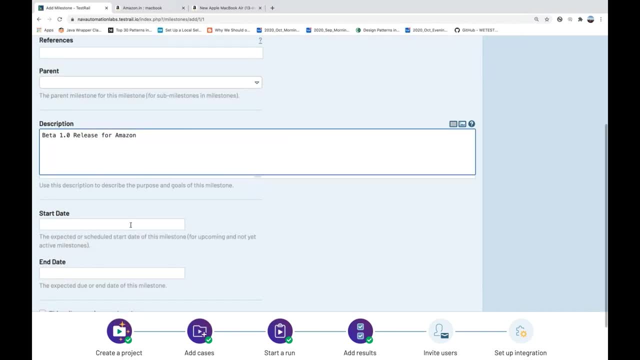 Okay, If you have any reference documentation or wiki page or something, you can do that. If you have any parent Milestone? No, we don't have any miles paid in Milestone And this is a description. I'll just copy paste the same thing. and this is a start date and end date. 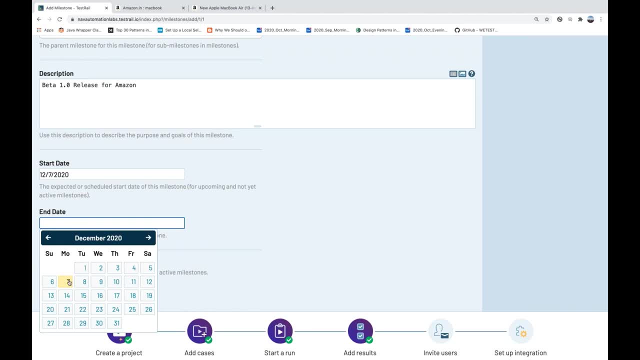 You can do that. So let's see, This is a starting today and end date is on the same day. or you can add multiple days over here And this milestone is completed. No, It's just simple: add this particular Milestone So you can see that. 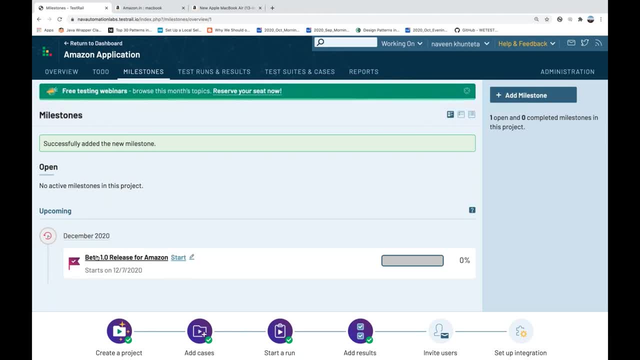 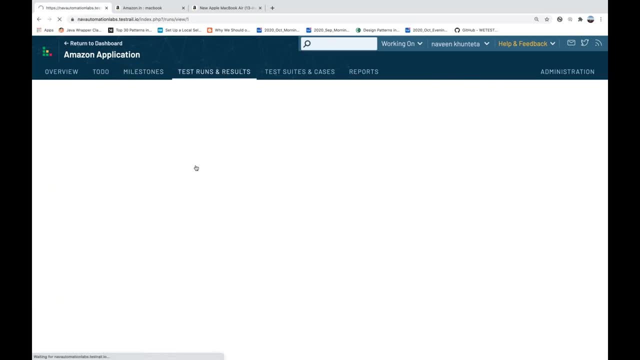 Okay, Yeah, this is the Milestone in December month and upcoming Milestone that we have. Okay, So when you go to a test runs and the results and you simple click on your cycle number 1.0, and if you read on it, 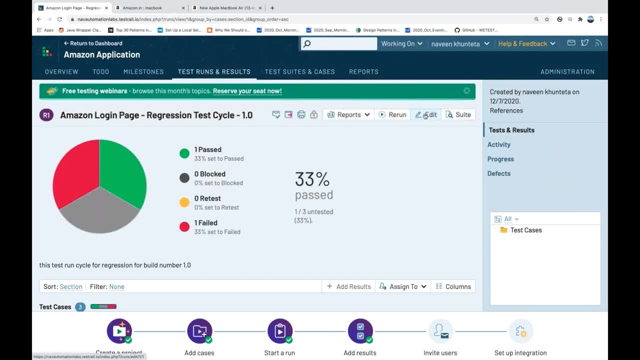 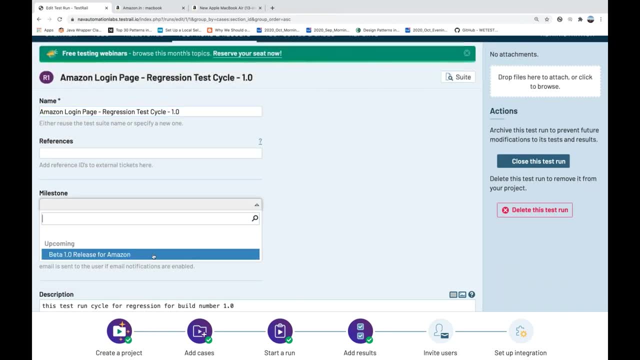 let's see. I just going to read on it once again. So let's all, let's see, go to edit over here and here you can actually select the Milestone that we have created. It means this particular cycle Is a related to my beta 1.0 release for Amazon. 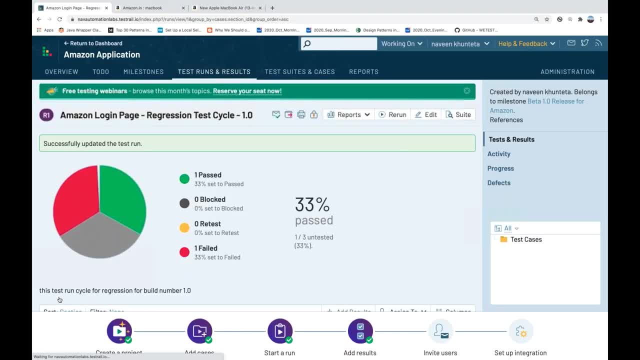 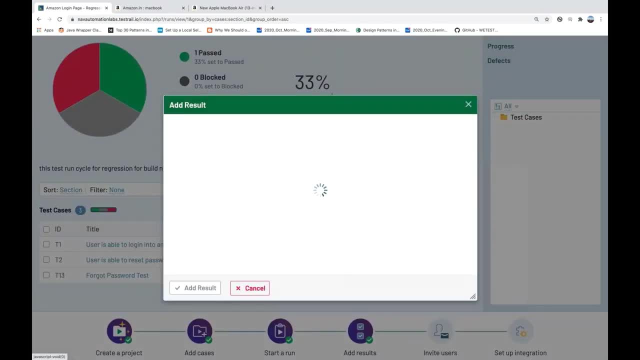 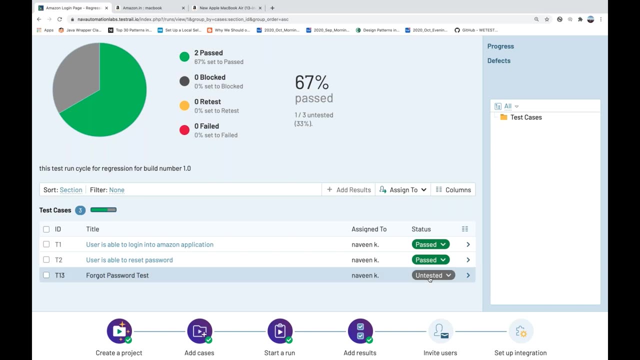 Okay, and you simple save the test run And once everything is done, I make that. see this for this reset password functionality also fixed and it is getting passed- and you simple say that okay, Yeah, this is as per expected over here and click on the result over here and the forgot password in this cycle. 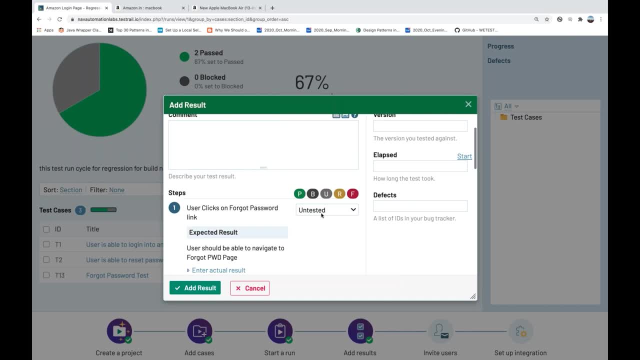 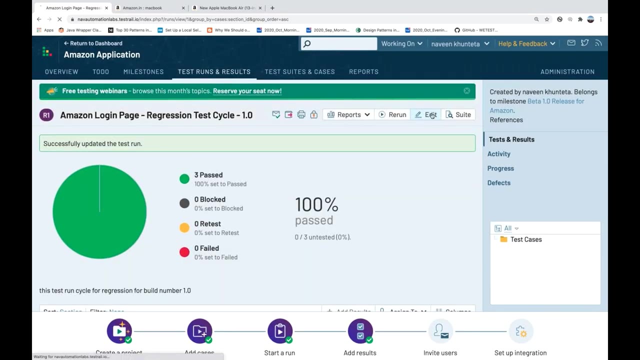 Again, I'm making it pass and I simple say that let's see, quickly make them pass over here, Because this is a new cycle. actually get guys that we created and we have added all the test cases over there. So click on result Once again. everything got passed, perfect. and then simple click on this added and close this run also and yes. 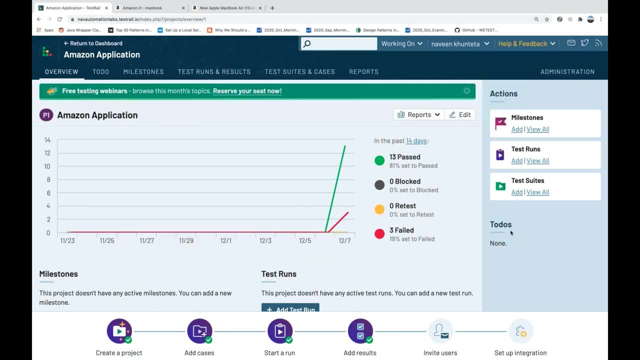 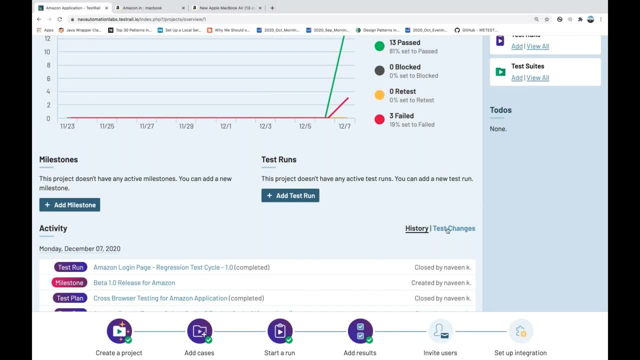 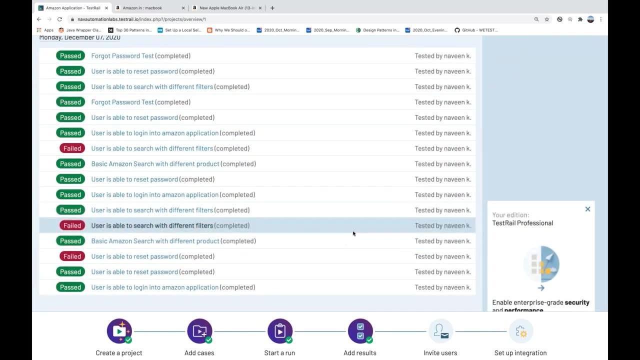 Now you go to your overview, You see that, Okay, you don't have any to lose and this is, these are the activities. Okay, that you have. and you can check the history. You can check that The test changes over here. Okay, like this. so complete dashboard. 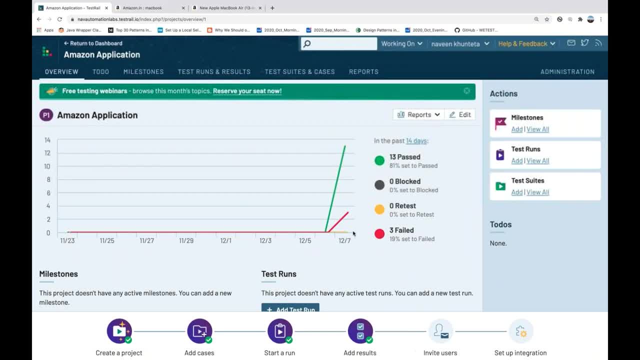 It will, it will show you and, yeah, if you click on reports, So different type of reports, you can check over here. Somebody, somebody for cases, somebody for references. all those things, guys, You can, you can explore by your own later whenever you okay. 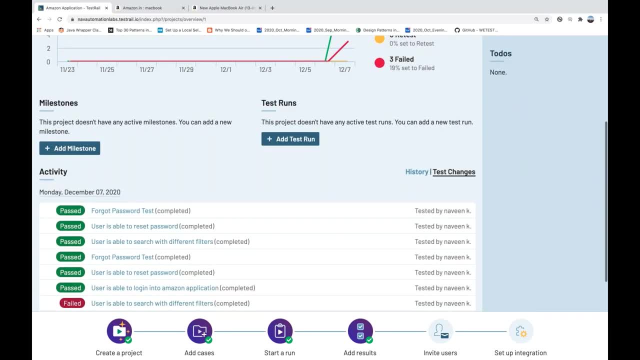 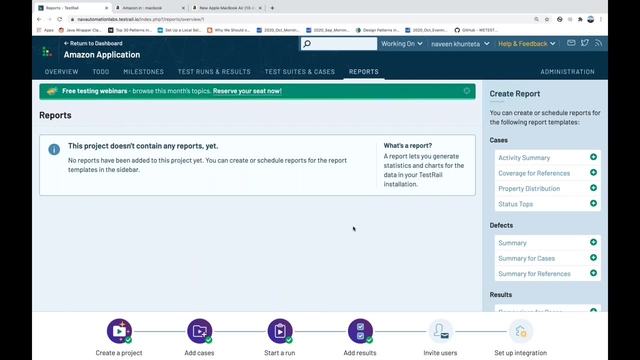 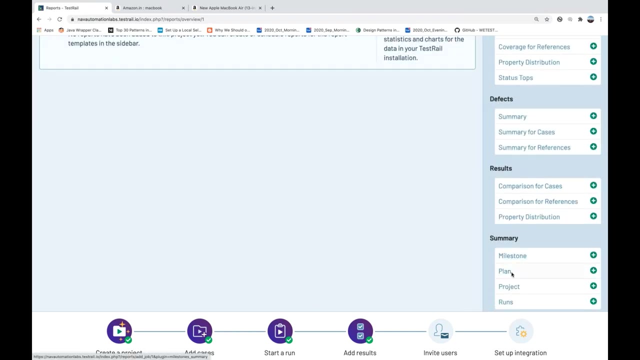 It's very simple, very straightforward. You can check it, right, guys? Okay, I'll go to this time report Section, and the report section Also. it's a. there are a lot of types of reports. You can say that case wise, defect wise, result wise, the summary wise, if you have any milestone, if you have any plan, or something like that. 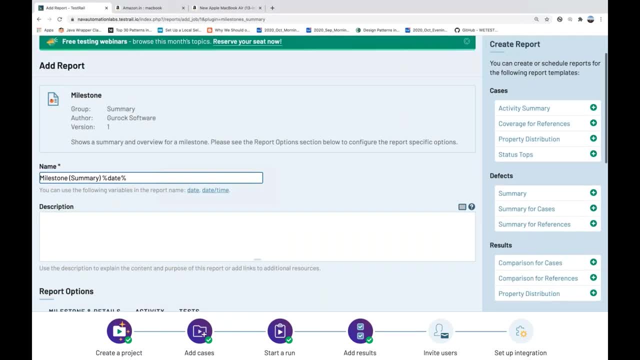 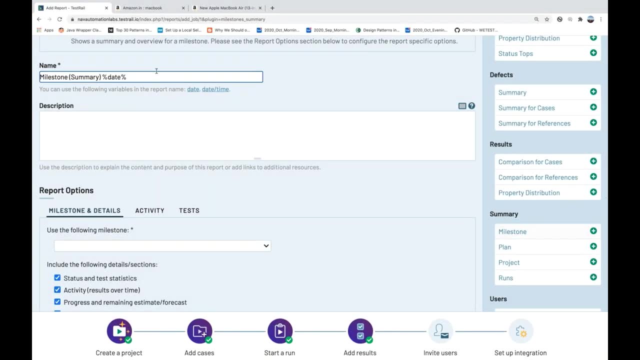 So let's say, go to milestone over here, You see that we have one milestone. Okay, So this is actually a template. Okay, this is this. is that milestone template and what are the name you want to give of the milestone you can give that? these are different configurations. 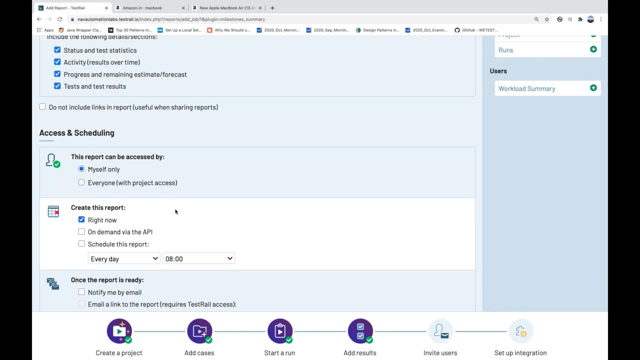 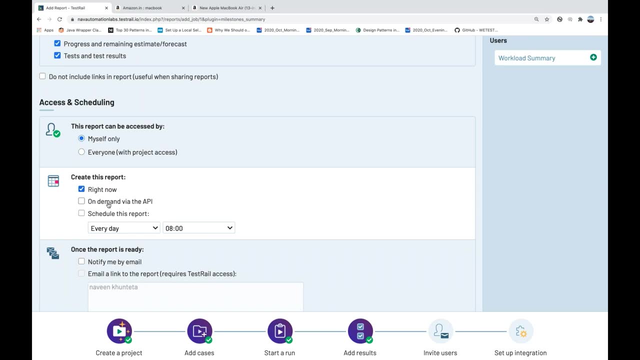 You can see they'll milestone will be accessed by everyone or By myself. Okay, you can create this particular report right now or via API or something. So generally we don't use on-demand by API. Someone is trying to use this particular milestone. 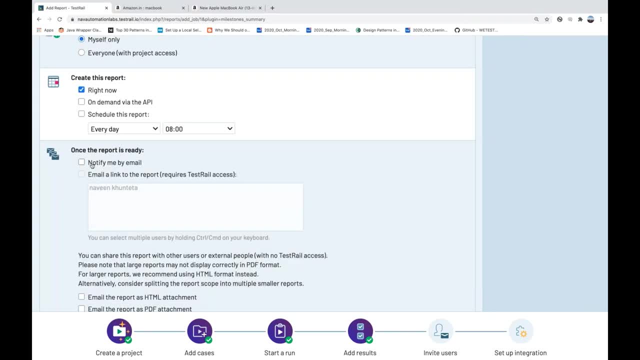 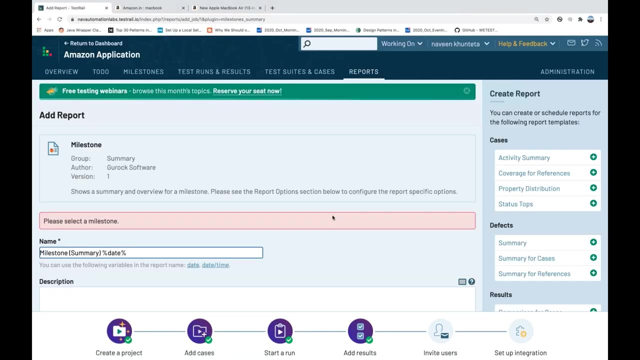 We can give an access via API and once the report is ready, notify me via email or email a link to the report. Okay, to this particular required test rail access. So you have to give the access over here, like that. So there are a lot of options. you can see that and then let's see, click on add the milestone report. 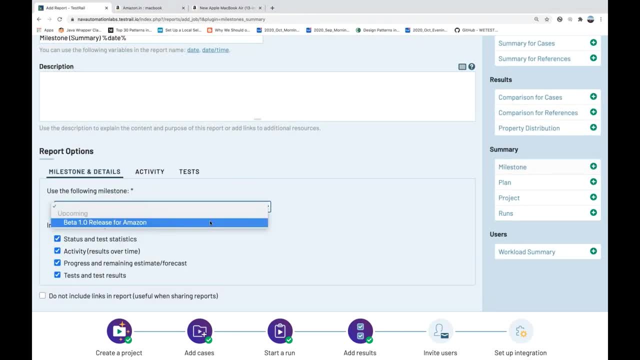 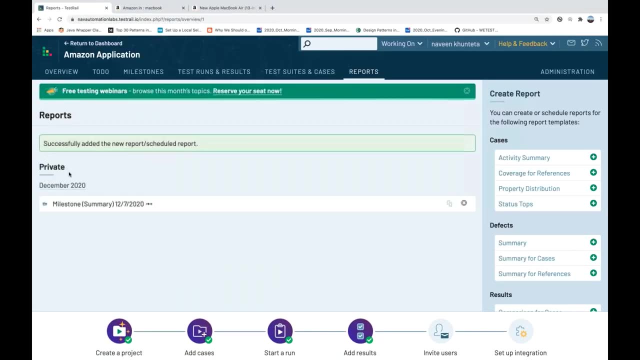 So please select a milestone. So, yeah, we have to select the milestone. This is for beta 1.0 milestone and simple add the record over here So you can see that this is a private report because it's selected only by me and it's actually creating a report over here like this. 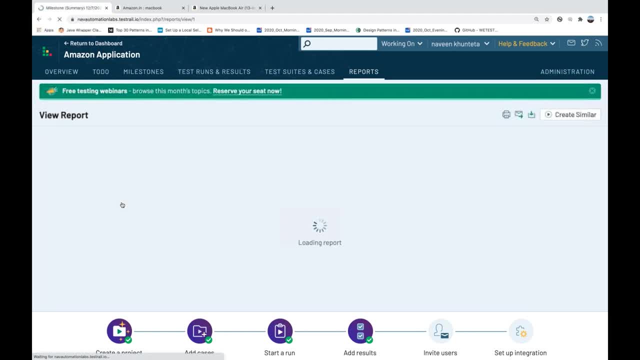 And once it is ready, you can just click on it. Let's see, click on it And this is the complete report We can see. for that particular beta 1.0 release for Amazon, We had three tests got passed, Zero blocker, like this, and you can share this particular report to anyone and how many cycles. 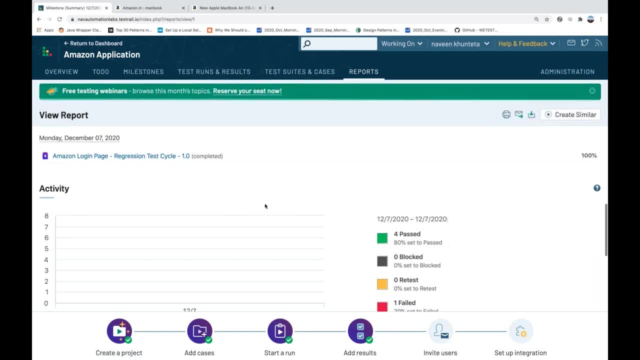 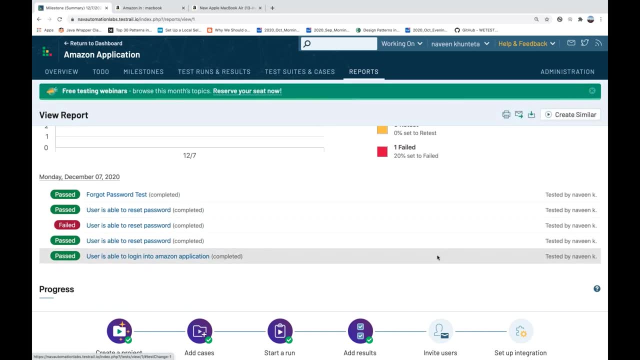 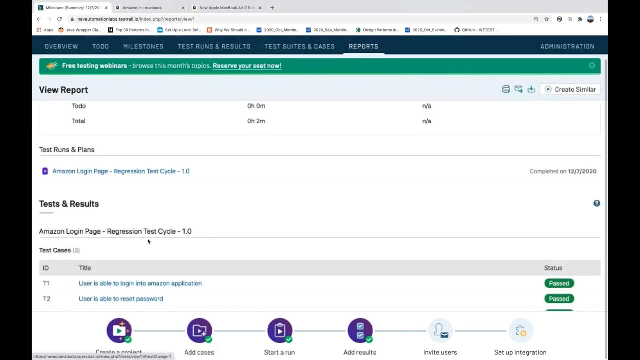 Yeah, we had this particular 1.0 cycle which got completed on this particular date. These are the activities, These are the test cases that we executed, completed by Naveen, tested by this guy. So complete report with the properties graph and everything you will be seeing over here: different mattresses, different results, cycle results. 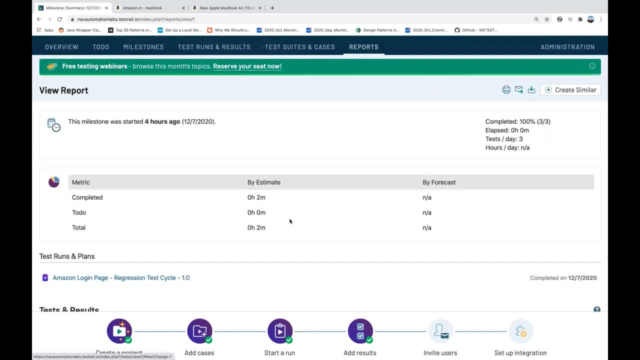 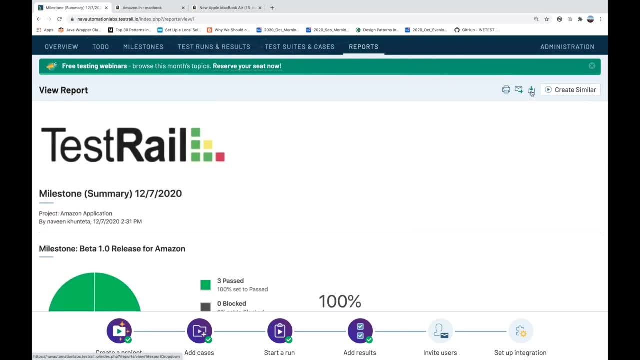 You will be getting it over here with the proper estimate and everything like that, So you can configure it, You can prepare it. different type of report. That's really good, And you can see this download by with HTML or download a PDF report. 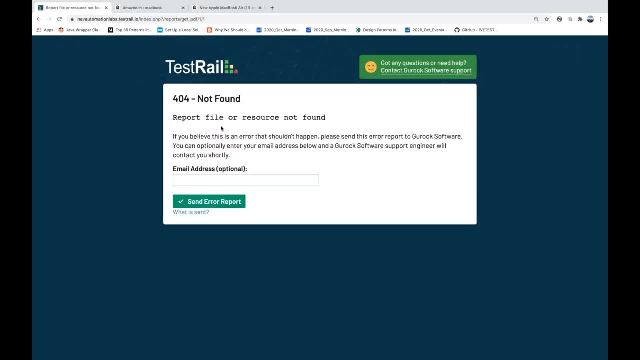 Also, if you really want to do that and you can put 404 not found, maybe, Okay, maybe address we have to pass and the same report. No, I think something some happened, maybe with the test account, Maybe this feature is not working. 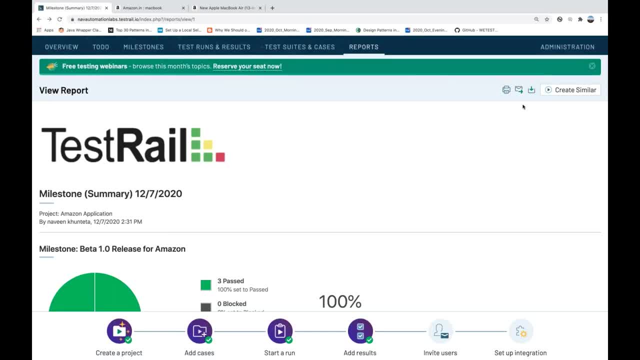 So let it be like this: You can explore it later. Okay, go back. Let me check with the Download. HTML is working. Yeah, HTML is working over here. It will give you a zip file. It will give you one HTML file. 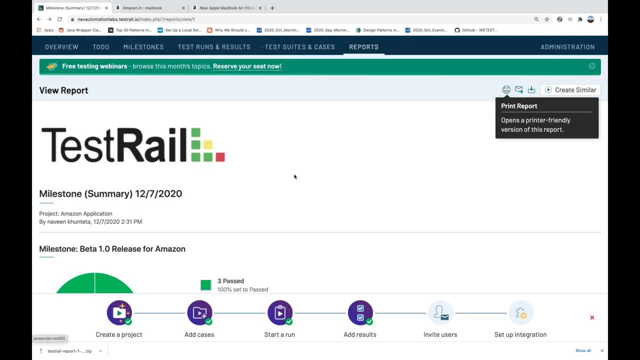 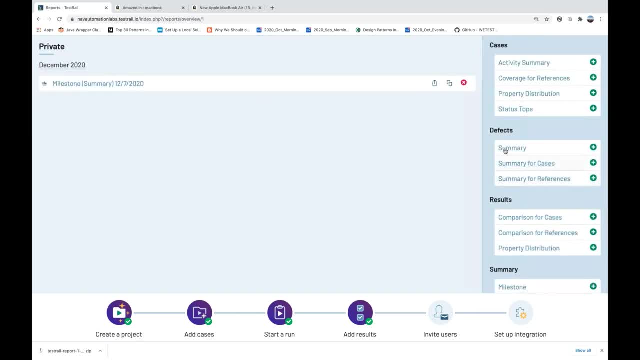 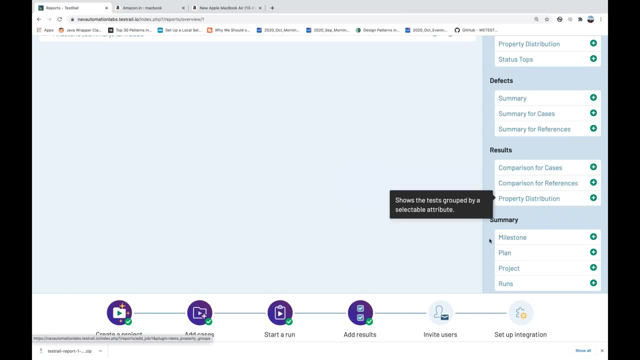 You can directly send me the send this email, You can print it Also this particular report, like that, Let's click on report section once again and then case-wise also you can do that and summary of a defect Also. you can get it over here directly and the result also: comparison for cases, references, property distribution. 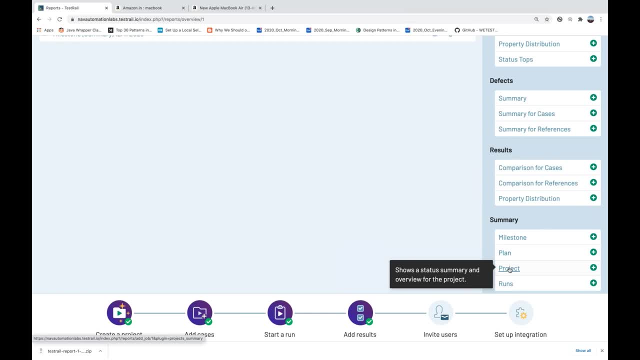 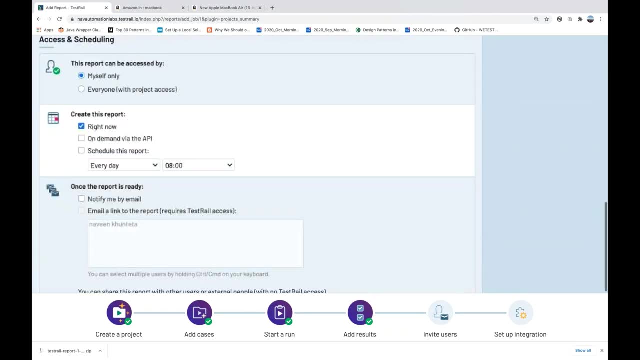 How many test plans that you have created. project-wise report also, you will get it. So let's see, We have only one project right like this and you can select. all these are different template properties. You can select that and then you can generate a project-wise report. 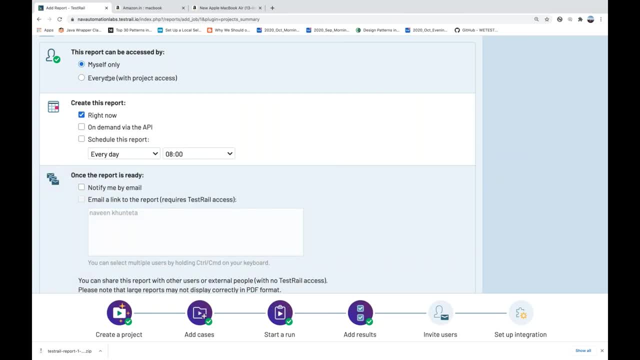 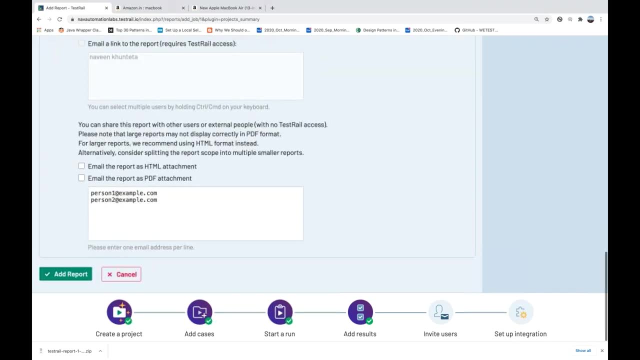 Also, you want to generate right now. Yes, only to me. Yes, if you everyone, then you can select with everyone also like this. So let's make it only for myself and click on add the report. So earlier we created the milestone report. 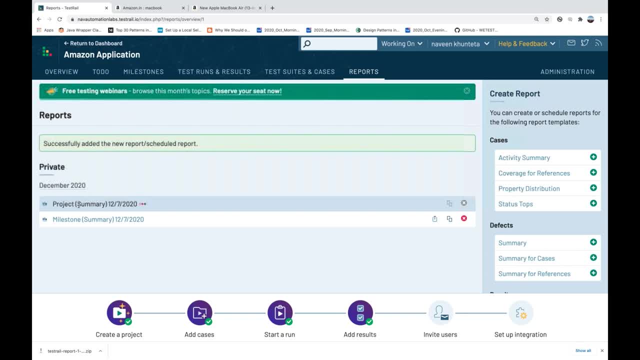 Now, this time we are creating the overall project Report. so overall project report, a case report defect, Somebody report defect for cases report, Milestone reports, lot of different types of report which will be helpful to create some mattresses. or you can share these reports to your team, to your management. 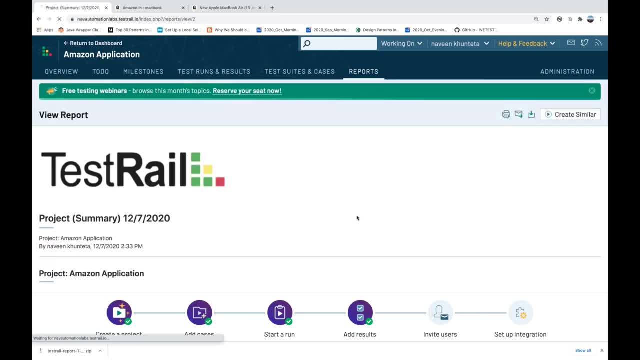 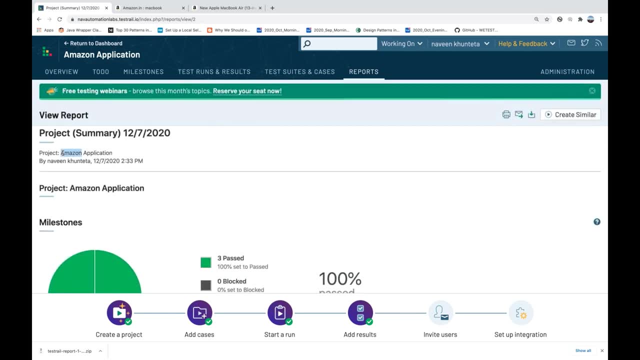 or the client. also, you can do that. The report is ready, Just click on it and you see that. okay, with the proper logo. test will logo and the complete summary by Navin on this particular date. This is the project: Amazon application and different graphs information. 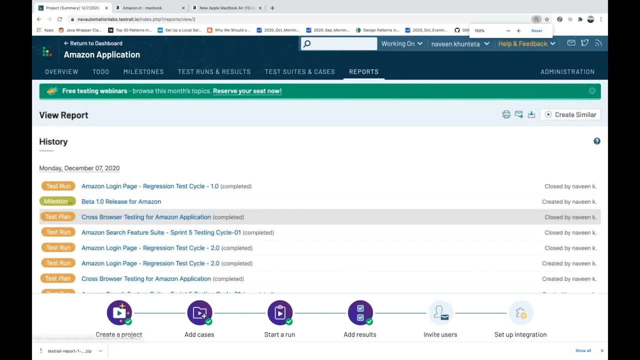 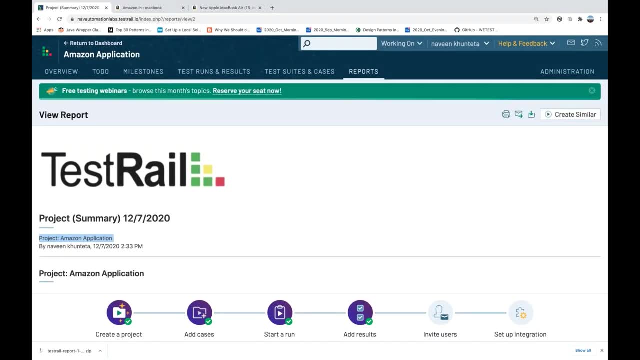 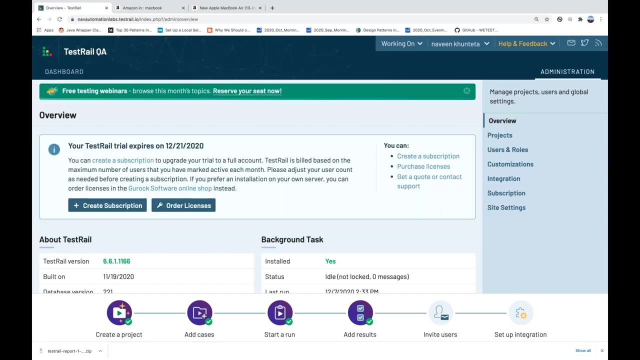 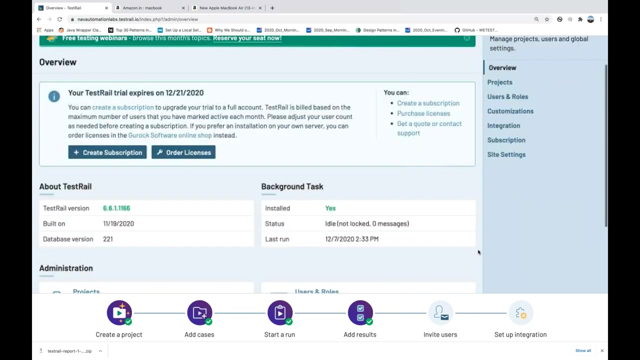 How many test cycles, test cases, history, everything. you will be okay seeing over here like that, Perfect. So likewise, guys, you can do this thing as well. Right now Let's go to the administration part. administration part is not that important because it will be for the overall administrative label configuration that, if you really want to add some plug-in, 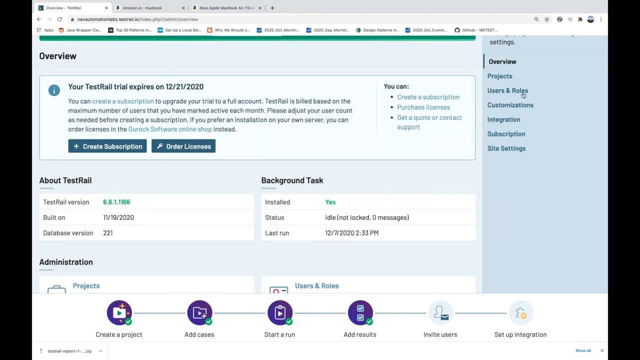 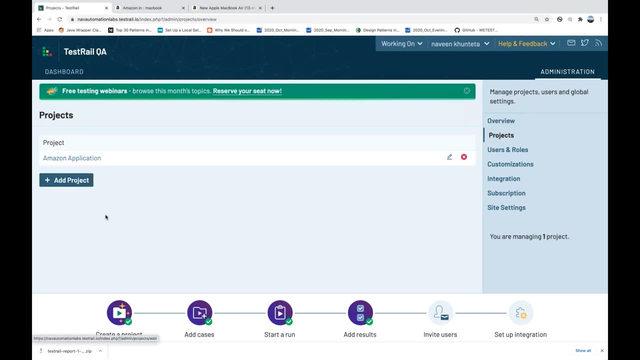 or you want to add some API in a enablers you want to do that. user and roles if you want to create, So let's go to the project level administration. We have one project. you can add multiple projects, So it's not like everybody is able to create the project. 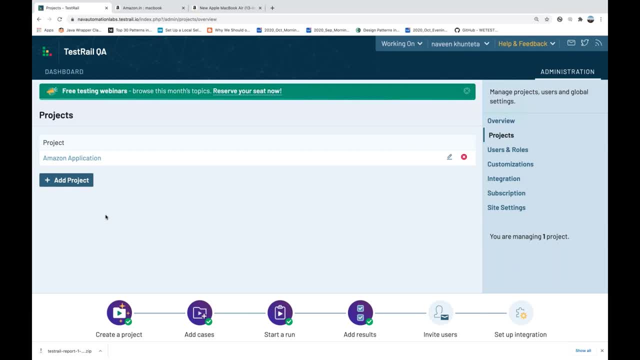 So let's see, you are the admin and there is a new team over there, So they will request you to create a new project over here. So let's see, you are going to create a new project over here. Let's say this time: 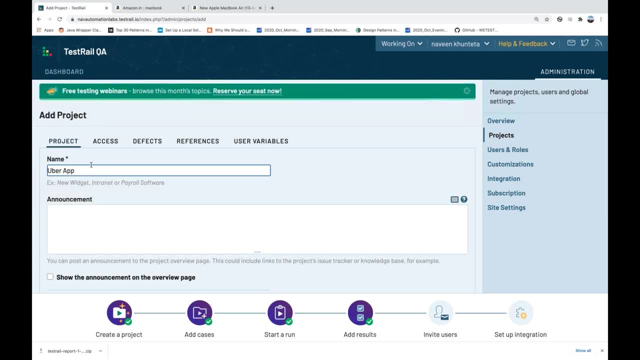 I'm going to create a project. name is: I want to test Uber app, or let's see in Amazon only. Let's say: I want to take order order management team over here. Okay, So order management for Amazon. like this and you can announce it. 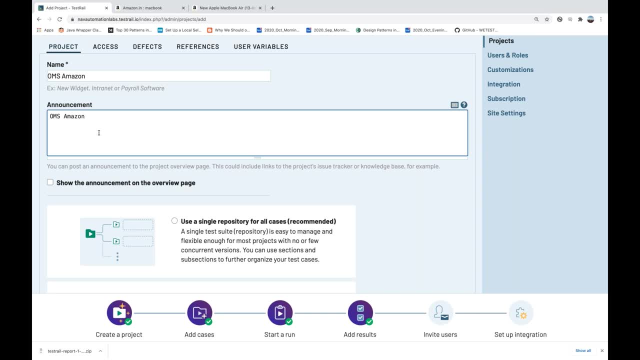 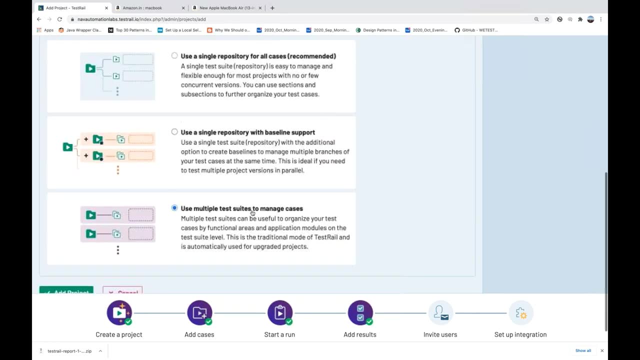 Okay, Yeah, this is a project that, okay, We are going to launch post announcement Also, you can do that. and the same formula: single repository. You want single depository with baseline support and you want multiple test suite to manage that also. 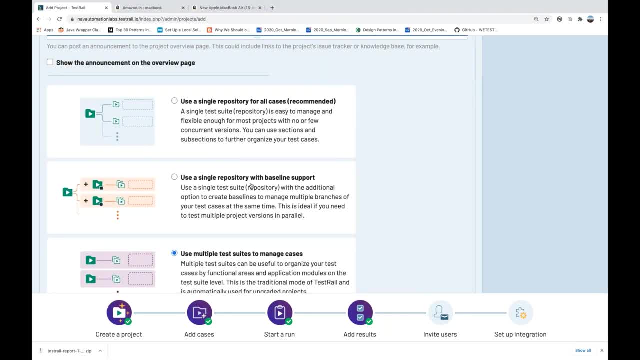 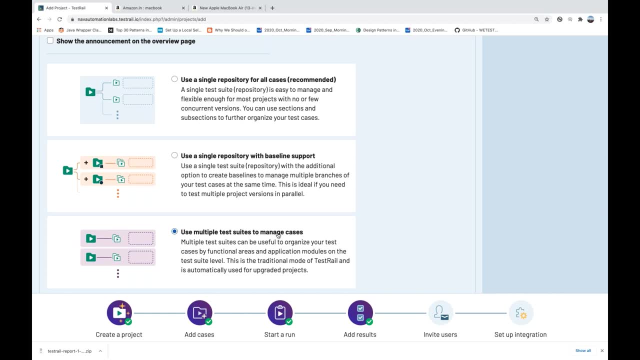 You can do that, Okay, so it's up to you. I have already explained what you mean by single repository, single depository, with the baseline support. I would prefer multiple test suite to manage cases because we really need multiple test suite for for the single project. 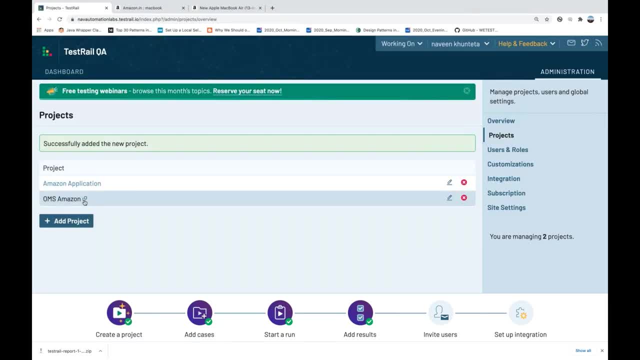 or for the single application, and let's see, click on that project, project got created and then and then we are good to go with that. Okay, Now let's see the user and rolls here, You can see that. Okay, Yeah, I have this admin user. 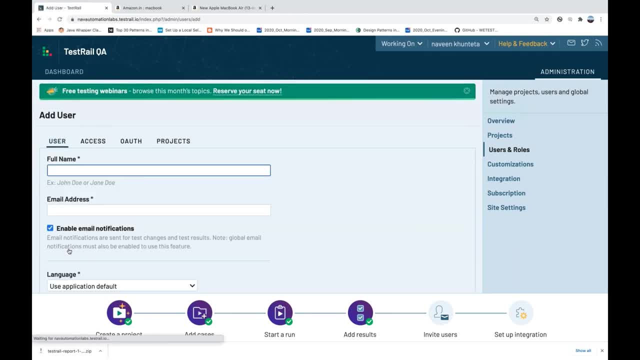 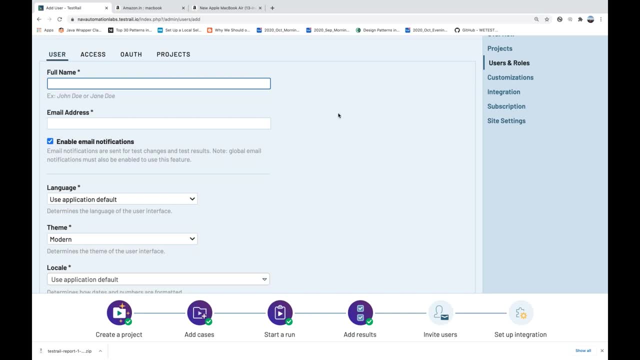 You can add multiple users over here and simple click on add user. Once again, full name email address in your company. Let's see a new joining. It's there and you want to create an account for that guy and then give the X's and everything. 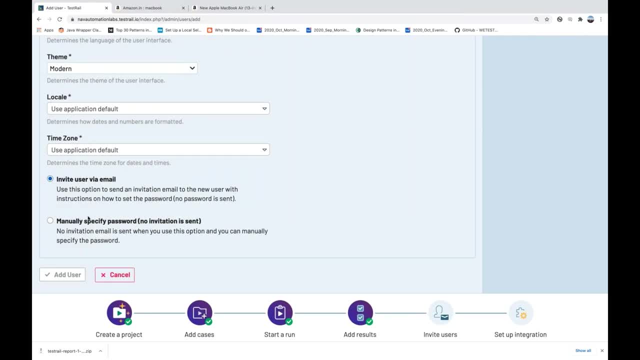 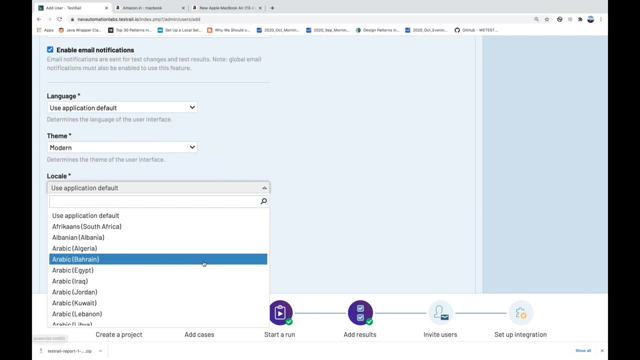 Okay, you can do that, all these things. So invite user via email or manually specify password. No invitation is sent like this: Also, you can do that. local specification Also you can do that. Let's see, you are in India and that person in somewhere in, let's say, in Japan. 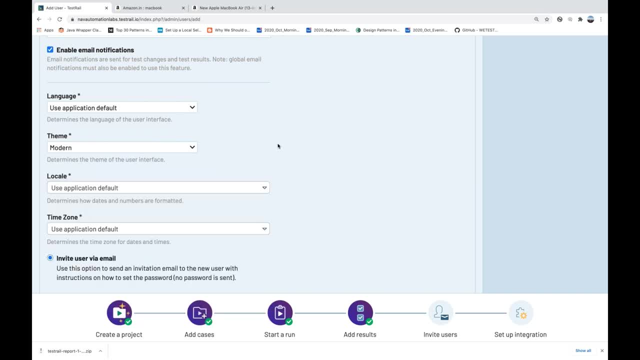 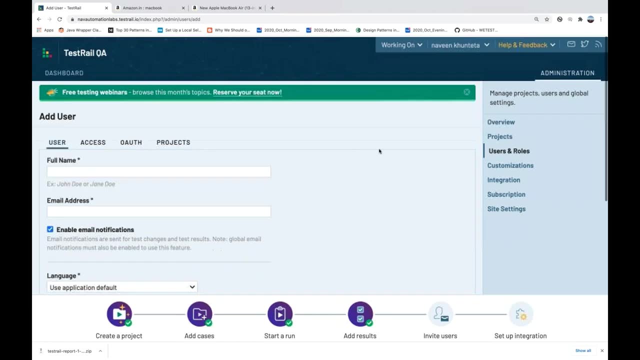 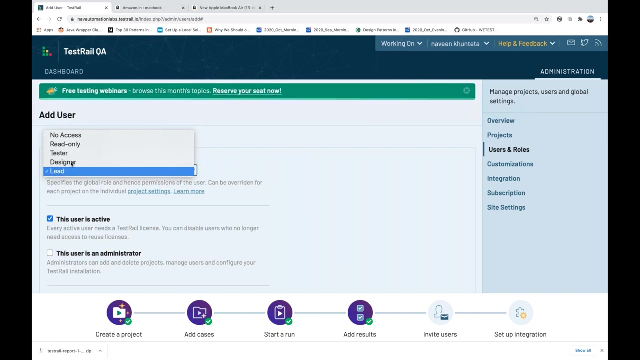 So, according to the local wise also, you can select the country wise Also, you can select that, which team, all those things you can. overall It's a common theme across the organization. You can decide and you can do that. Perfect, You can give the X's what kind of role we have: tester, tester, designer, lead role, read only or no access, only read only. 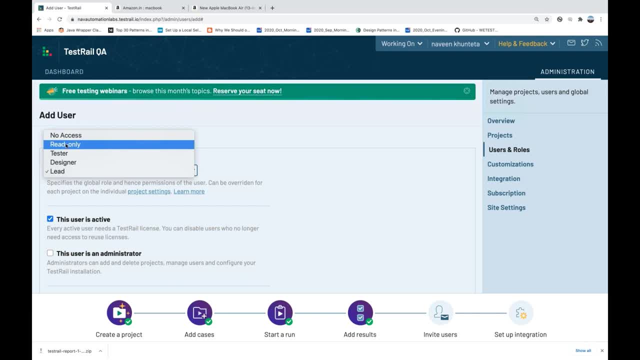 Let's see There is a, there is a contractor You just want to give only read only access for all the test cases, test suite project and everything. So that guy will have only read only like this. Okay, you can make that guy as an administrator also like this. 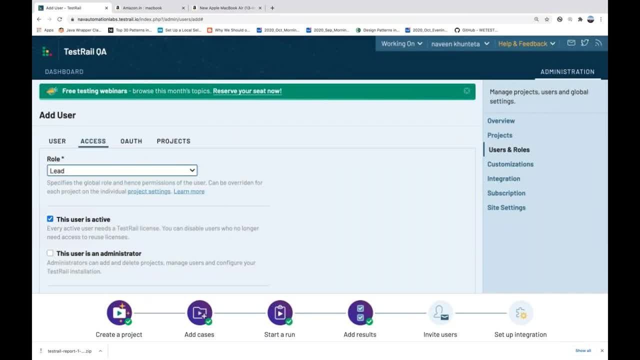 You can do that Right days. Then we have OAuth, So configure OAuth. generally it is for assemble instance might be configured by the administrator before connecting via OAuth. So you have to first of all install it and you have to connect the account. But generally you can ignore that part. 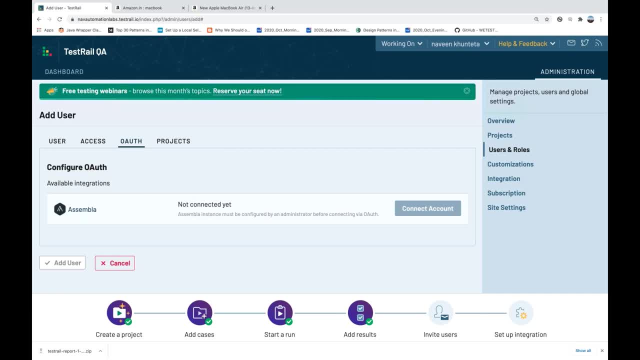 Even I haven't explored much, I haven't used this thing, So you can ignore that- and which project this guy is associated with that. So you can see that. Okay, Yeah, this guy is the in OMS Amazon. He is a tester. 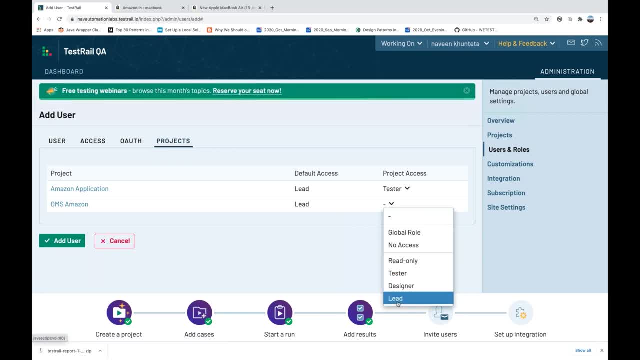 But here he is, Let's see lead over here. So like this, you can select: or let's see someone is working as a developer over there- designer, developer, lead role or global role. He's a VP, or maybe testing testing head is there or a test manager is there, so you can give according a different roles over there. 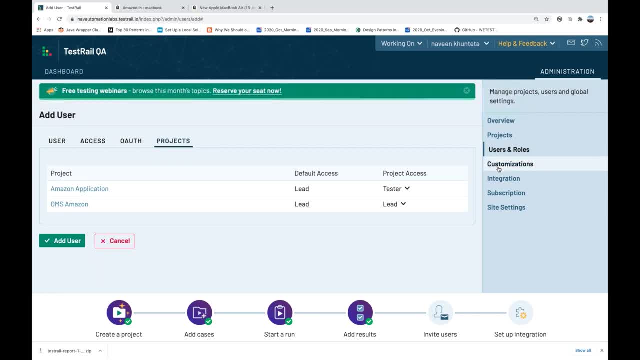 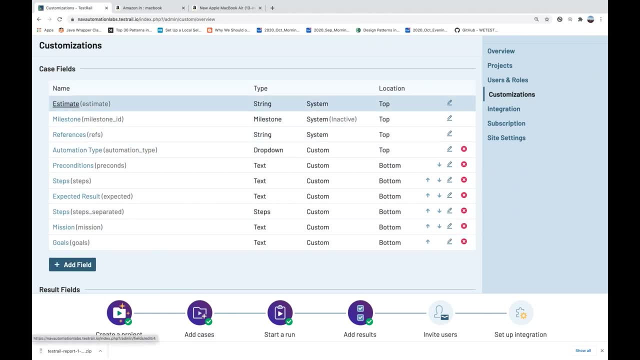 And then you simply click on add user and then the user will be created. some level of customizations Also. you can do that. Okay, you can add multiple fields: What type of estimation Milestone references, So you can customize at the admin level. you can do that in the result field. 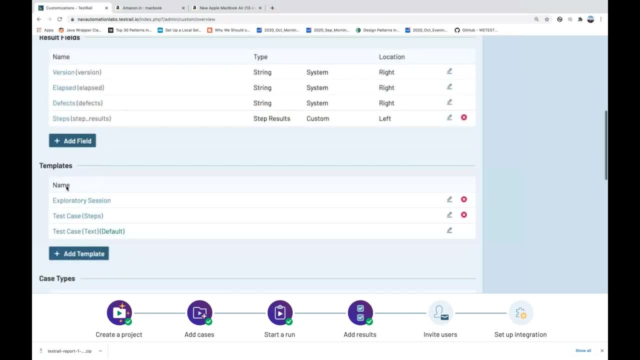 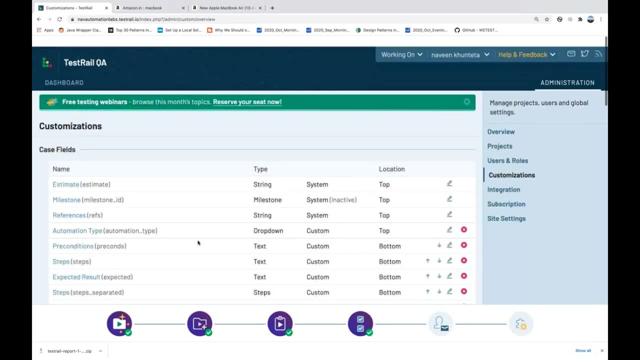 What exactly want to show: version labs, defect steps. You can do that. These are templates. If you have other templates, you can add more templates over there, But this is not important for you guys, because you will be working as not the test rail administrator. 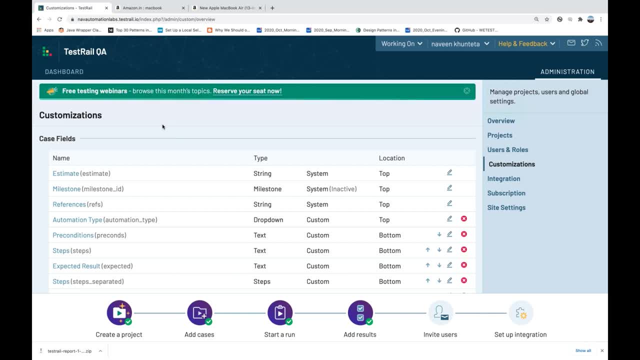 You will be working as a tester over there and you have to use the feature of designing part and the running part and the dashboard. that is important for you guys. But if you are working as an administrator and you have a responsibility to configure it- and it's very easily configured- you can configure and then a lot of good documentation is also available. 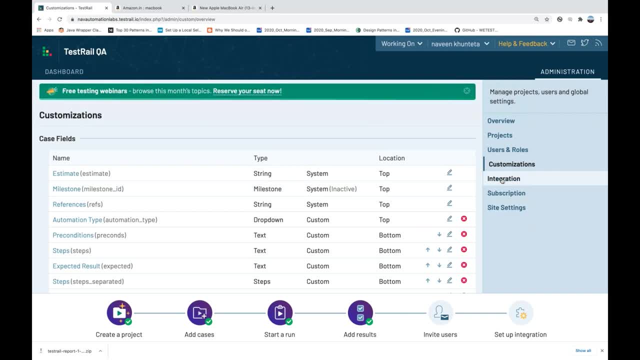 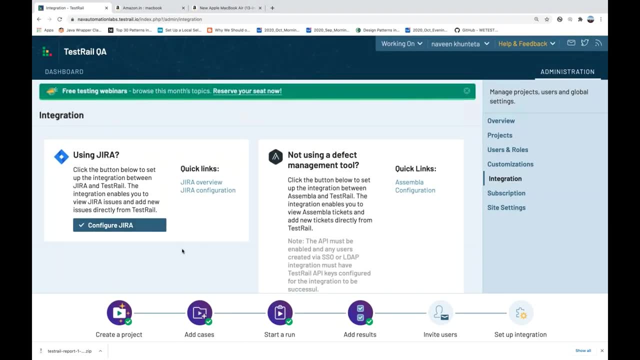 You can check your documentation, videos and everything. you can check that. then you go to integration. Yeah, that part I can take it later Maybe in some other video. you can configure Zeta accordingly and then you can connect with your Zeta. Also it's saying: click the button below to set up the integration between Zeta and test rail. that is possible. the integration enables. 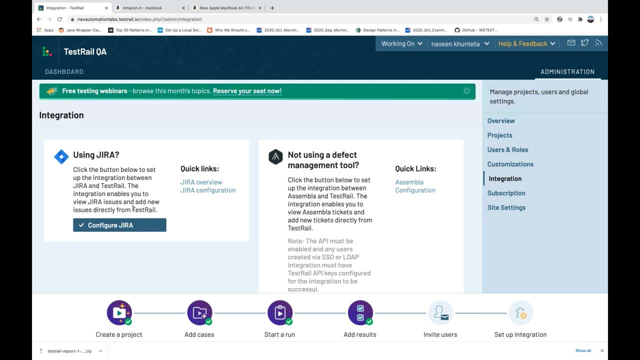 You to view Zeta issues and add new issues directly from directly from testing. Wow, that's a really good feature that the moment you raise a bug over here immediately If you raised in Zeta, we just need to click on configure Zeta. 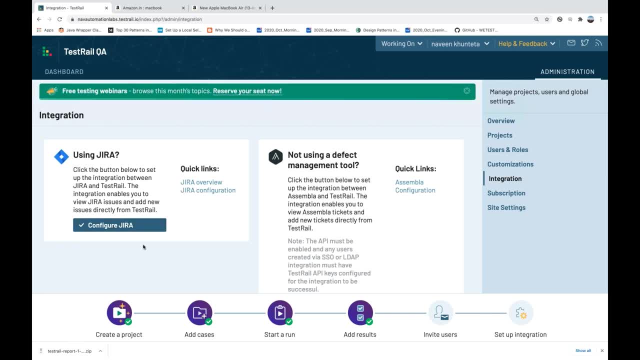 So let's see: for test management point of view, You are using test rate, but for defect management point of view and the user story and the sprint management point of view, you are using Zeta for that. So you can integrate between a test rail and the Zeta, but you should have a Zeta account in your company. 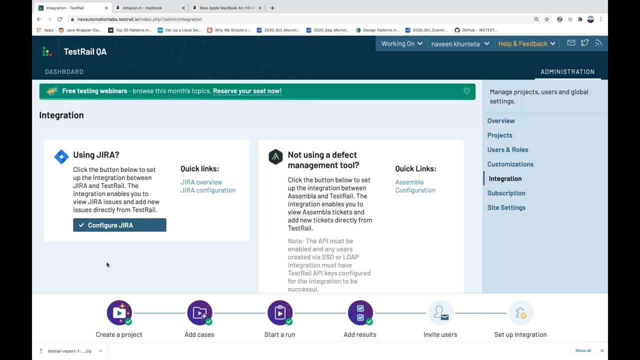 But sometime maybe In some companies they might not prefer that because you have to pay for Zeta and you have to pay for this test rate also. but it depends. Okay, come be to the company. If you have that, definitely you can do that. 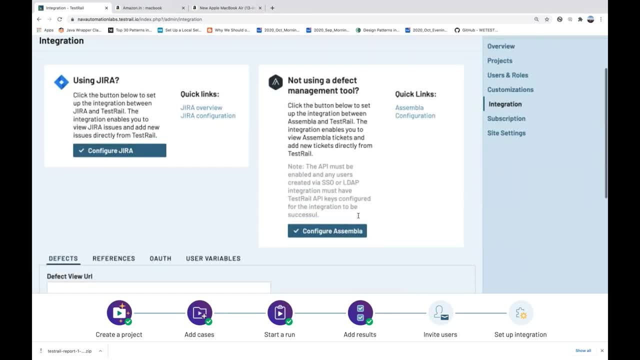 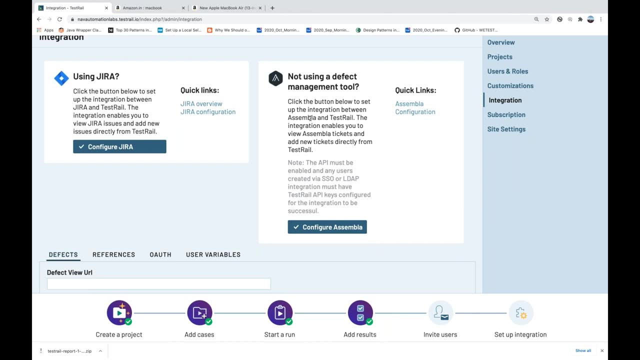 If you're not using any defect management tool, you can use your configure assembler. assembler is another tool. You can see that. click the button below to set up the integration between assembler and test return a test rail. The integration enables you to view assembler tickets and add new tickets. 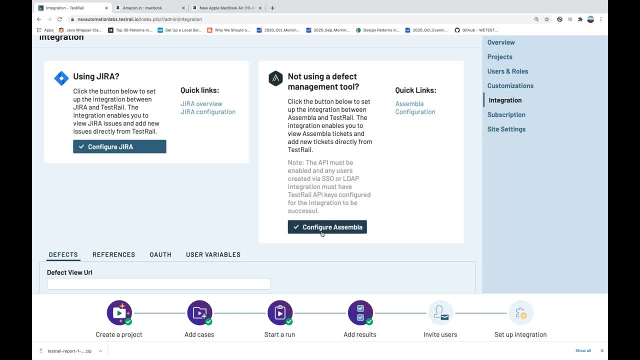 Directly from test rate. That's a nice feature. Okay, So this is a assembler defect management tool and you can view assembler defect over here in the test race Also. you can see that, Right, guys. So this is the configuration you can configure with the server on the cloud. 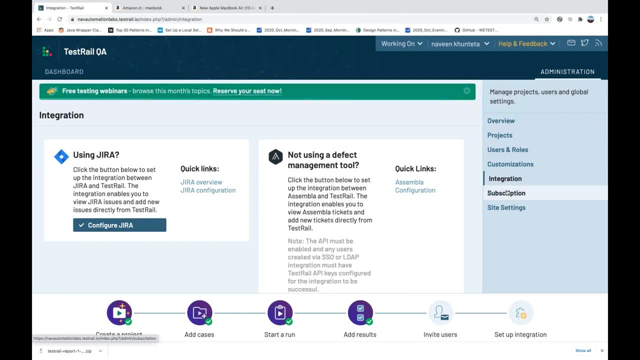 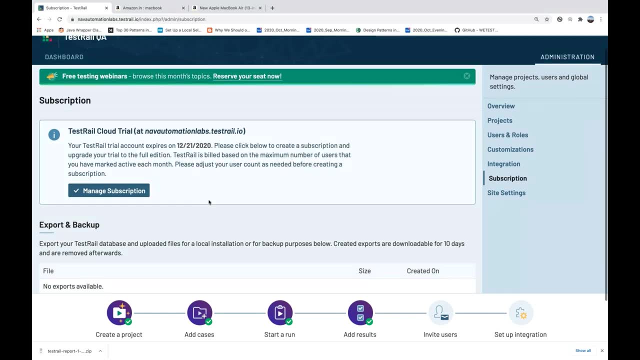 Also. you can do that. So these are the different. integrations are available. you go to the subscription and this is the trial subscription F. Okay, for this particular account You really want to extend. you have to pay for it and you have to manage your subscription. 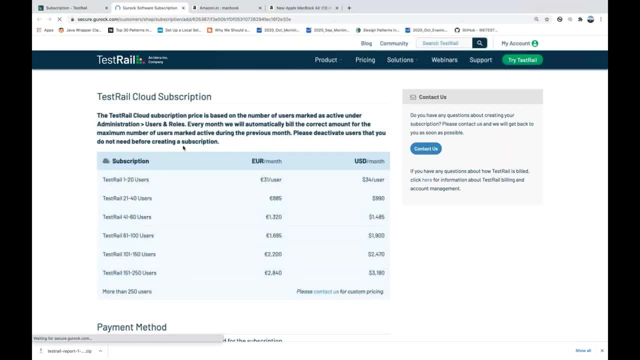 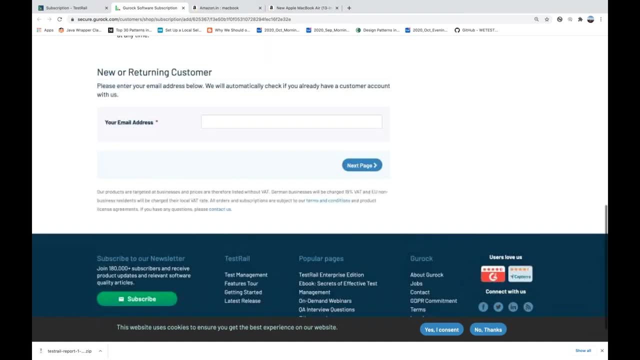 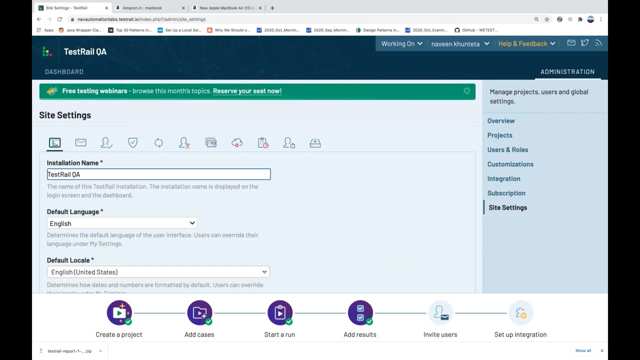 For whatever, according to their subscription plan and everything. you can see that these are the plans, Okay, per month and per year, and something like this You can read and then you can check it over there or you can directly contact with them like that. Then the last part of the site settings in the site settings, guys. 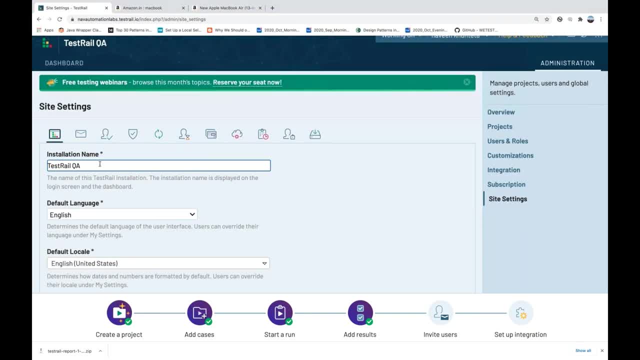 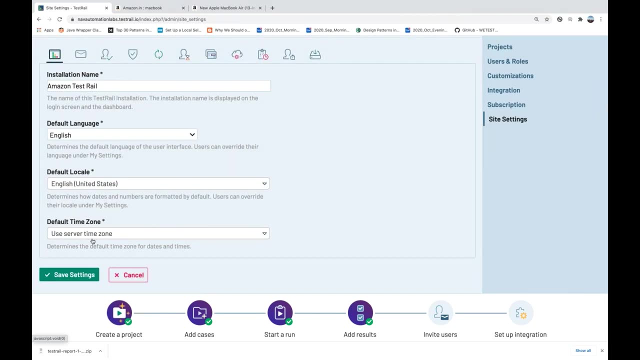 These are the different, whatever the installation name. So let's see What are the name is test rail QA. It's I'm working in Amazon. I simple say that this is my Amazon Test rail over here. which language? default language, default local and default time zone, user server time zone. 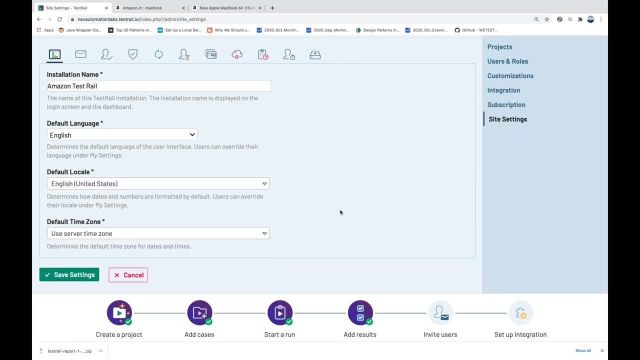 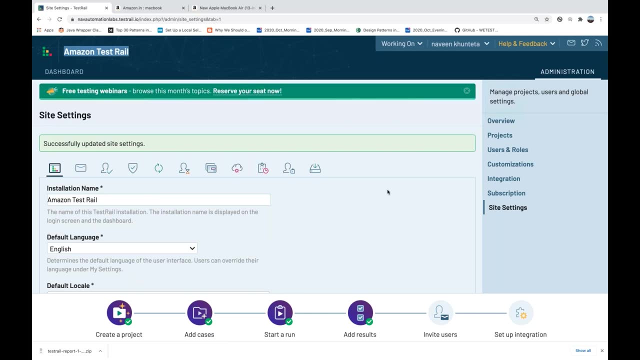 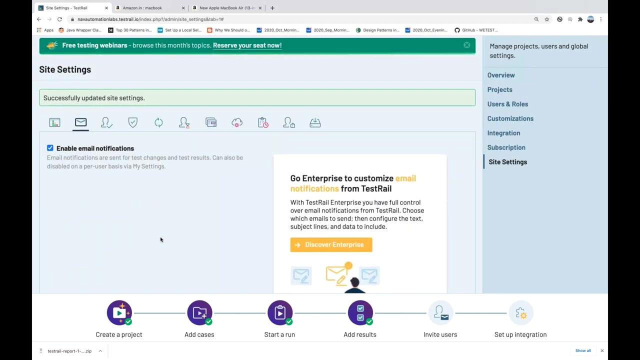 I would prefer not specific to the specific time zone and simple click on save the settings. The moment I say the settings, you will see that, Okay, it got changed. Amazon test rail over here like this: You can enable email notification, Yes, but every activity it will give you the email notification for any test changes or any test results got updated like that: 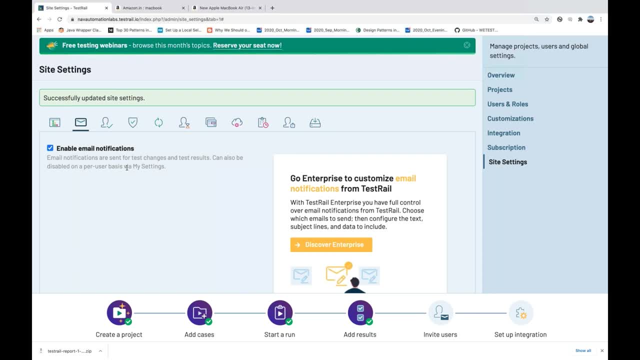 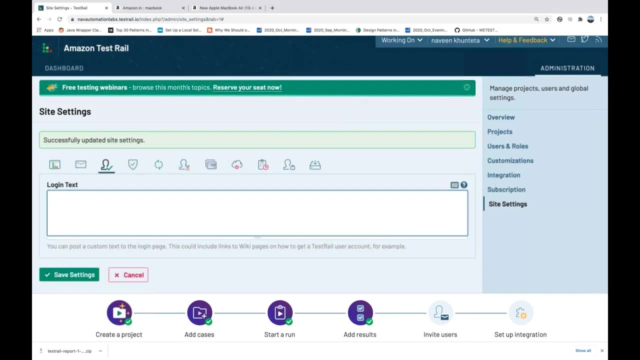 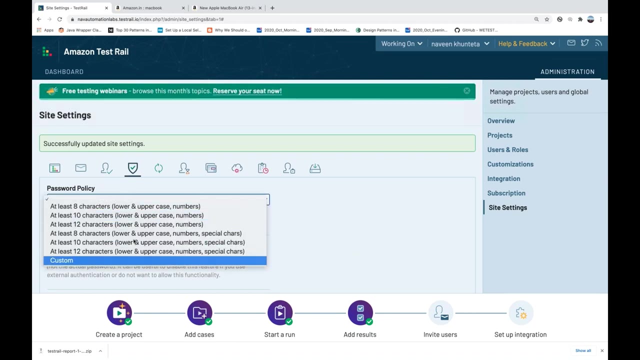 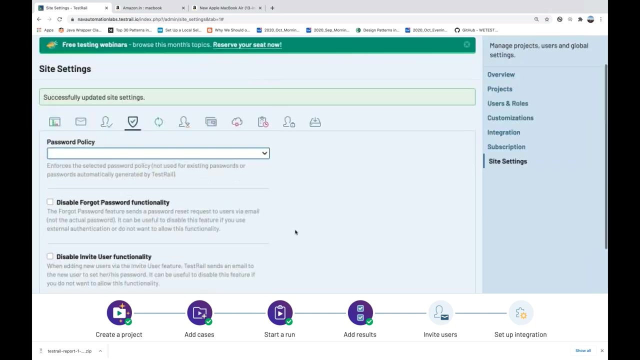 You can also disable on per user basis via my settings also, that you can do that. then the site settings for the login text also you can. whatever the custom text login page you want to define that also, you can do that. password policy You can define at least eight characters, 12 characters, all those things, and if you have any custom password policy you want to define that also you can do that. 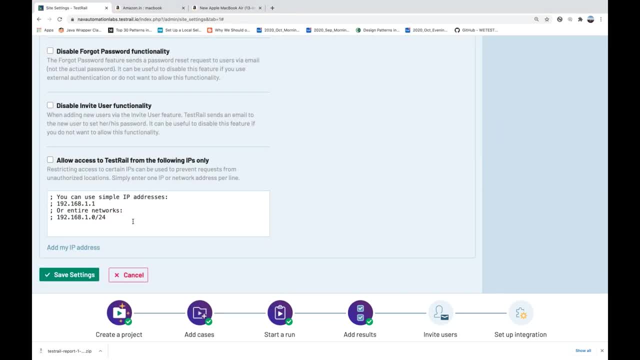 So that's a really good feature. allow access test rail from the following ips: So you can give the range of the IP addresses that within this particular range only people can access that or within your company network also, company network IP addresses range also. you can do that so that from outside of your company network people cannot access your test rail over here like that. 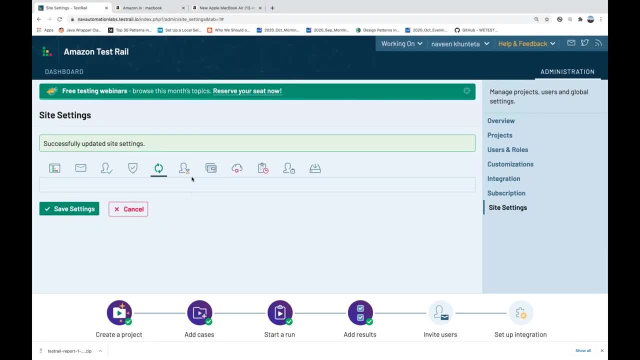 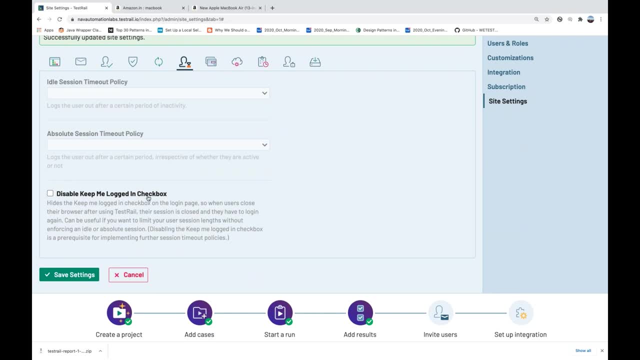 Okay, click on this. I think this is. I think it's blank over here and, yeah, this is also ideal session timeout policy, those things you can do that guys. keep me logged in checkbox all the time. That also, it will never be logged out. 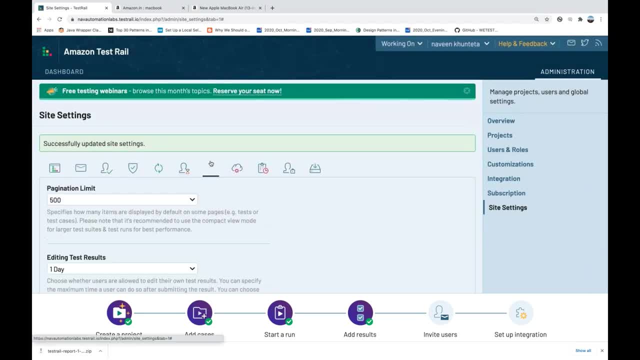 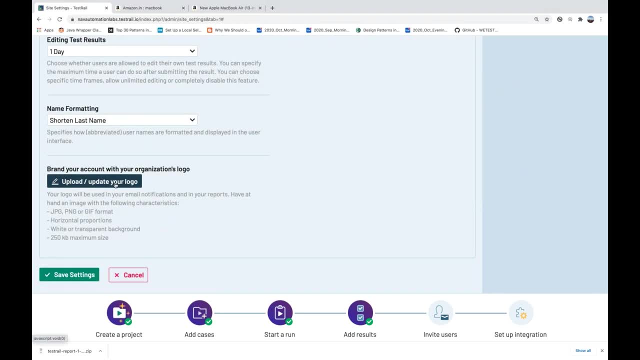 Okay, so this also you can have a look over here. This is a pagination limit: 500 generally. Okay, it's short and last name: nice thing, You can upload your logo also, whatever the logo that you have. So let's see, I have, let me add a logo. 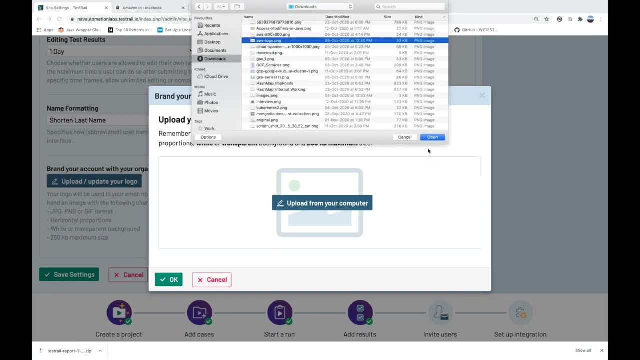 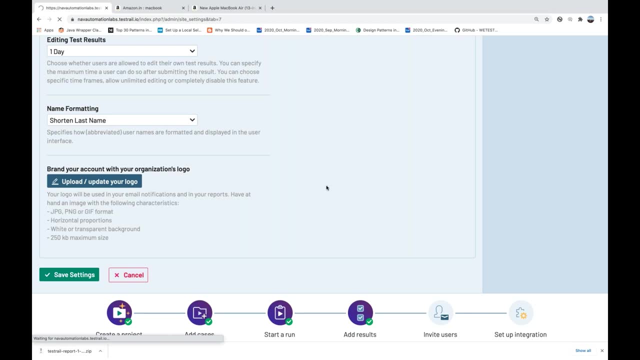 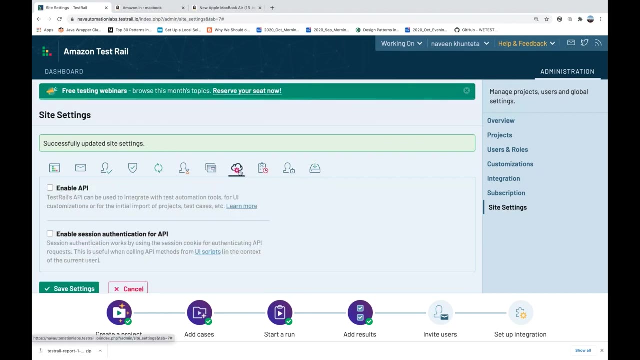 So do I have a? okay, So let's see, I have this particular AWS logo and simple click on open and then your logo will be added over there and simple save the settings. So logo should be visible, maybe on your dashboard or somewhere it will be. should be visible then. the next part is the site settings. 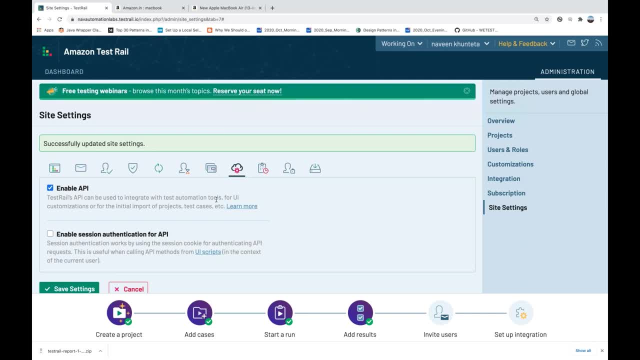 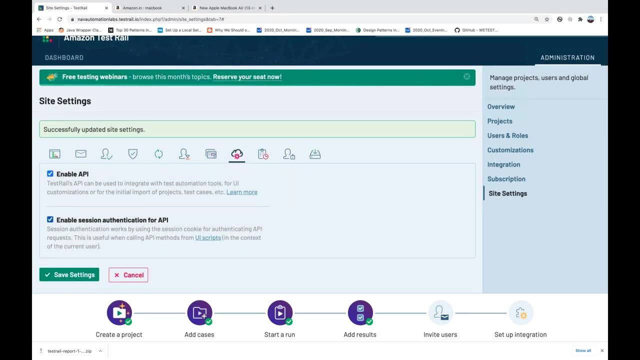 You have to enable, the API can be used to integrate with test automation tools. This is something very important and for UI customization. Maybe we can take this particular part later, guys, because when you enable the authentication and simple apis, why are the api? you just call the api from your test automation, from the test ng. let's see. 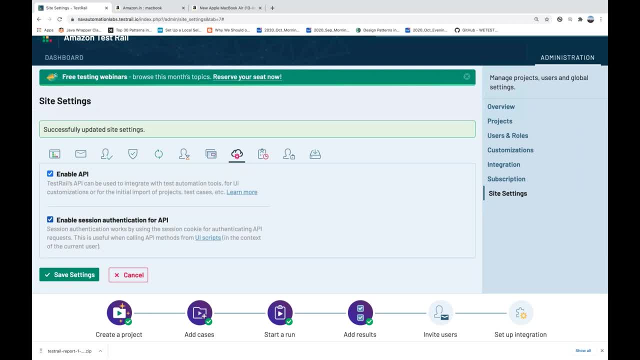 We're using selenium driver with test ng you, which is simple. This is a trigger for the failure test case in automatically. it will update your test case over here. You can map whatever the automation test cases with the manual test cases that you have written over here, like that. 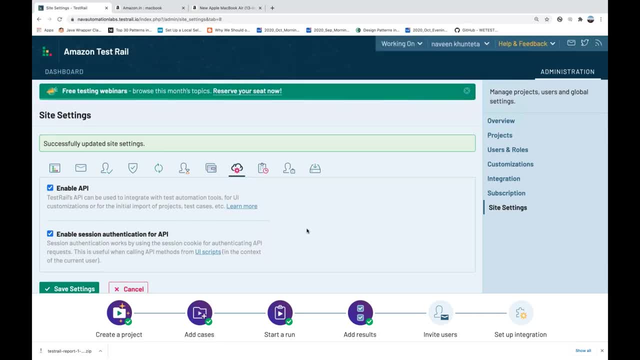 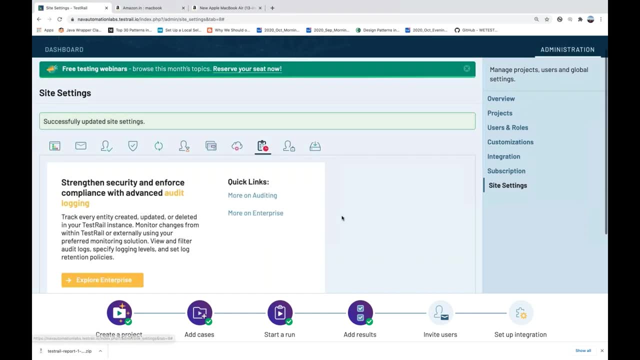 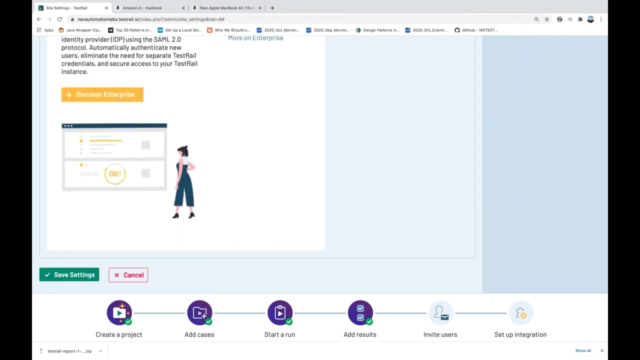 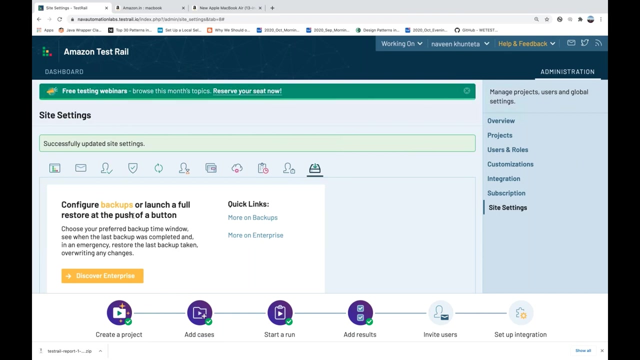 So let's save this particular setting. you can enable the API as well. So it got. I think it got saved on audio. Okay, it got saved and that is auditing part, auditing logging- that you can. this is a explore, the enterprise Version. maybe we can check it later. not that important. streamline user management with single sign-on also you can enable. that is again with the enterprise version. that also you can ignore that part as of now. and backup for launch, restore for at the push of a button. 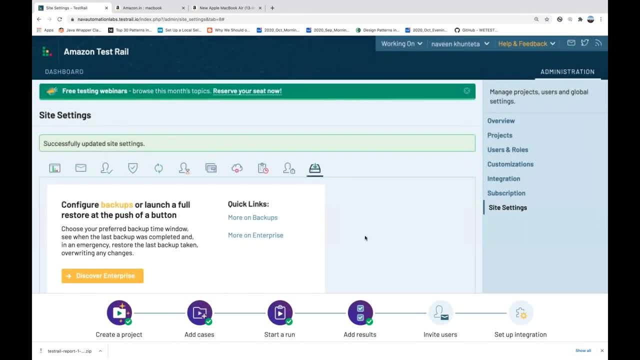 So you can restore and then you can take a backup for the entire data, Everything. Zeta also provide the same feature, because I have worked as a Zeta administrator sometimes in my previous company, So I know All these things like that. So I think it's not that important, guys, the admin section. but if you really want to know, you can a simple see that over there. 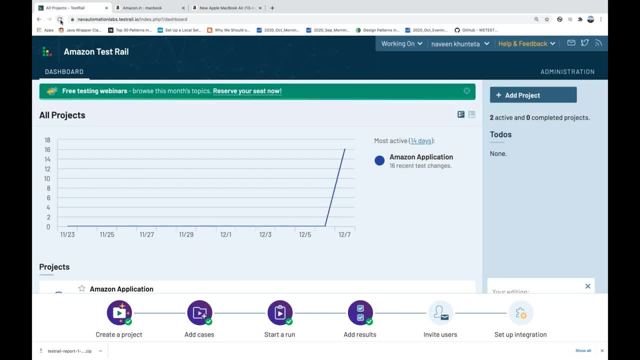 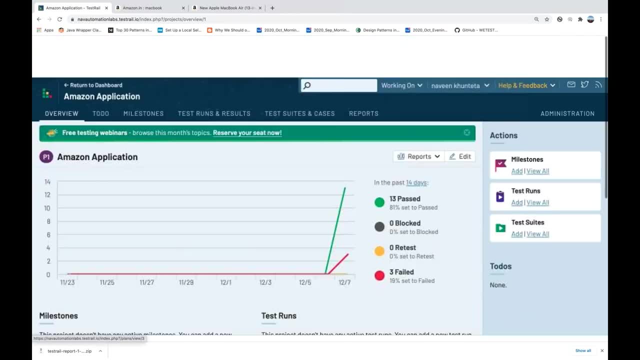 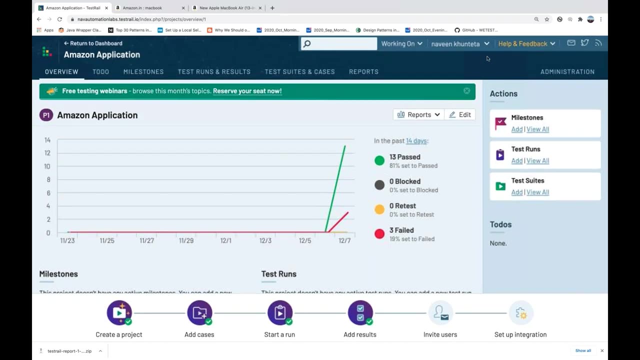 So let's go back to dashboard and let me refresh this page. Okay, I don't see where exactly the logo, Anyways, maybe, okay. So I think when we have to log out and log in again could be, maybe the logo will be visible over here somewhere, or maybe in the test, in the test account, in the free account. 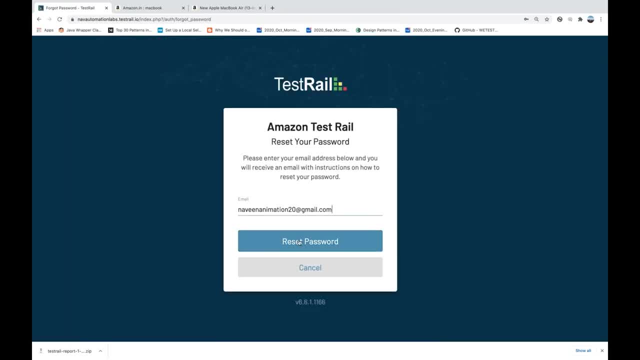 Maybe they have not that, so let me just log out way. This is my Username. click on reset password. Okay, this time I got successful. now let me enter my email ID And the password I'm going to enter and login again. 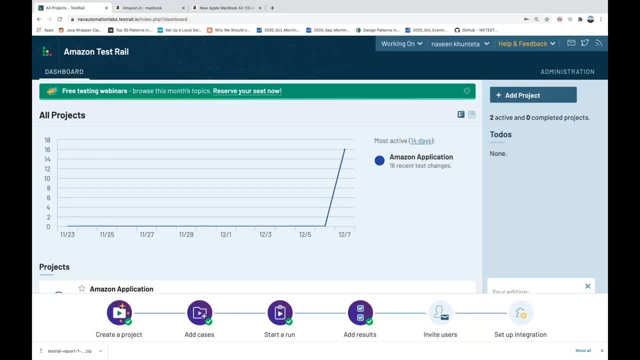 Done so good. In fact, I'll show you the email which I have got, which is my logo, actually with the Amazon logo that we have set up over there. Okay, so see, this is the see that this is the email That's just I got for the forgot password. 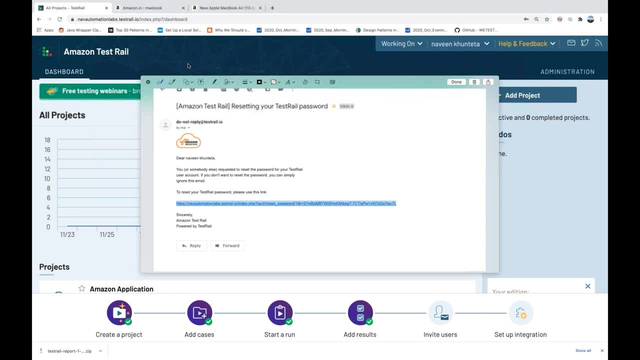 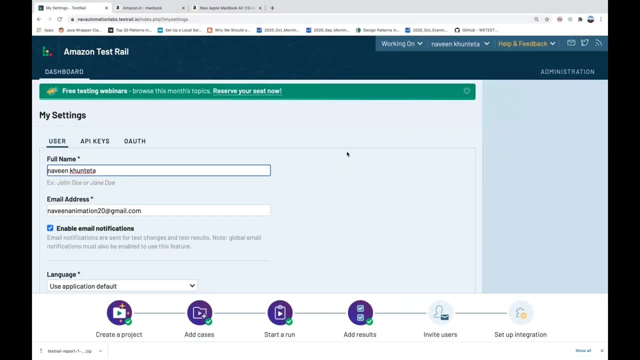 You can see the logo over here, Okay, but I don't see this thing here. It should be visible. Maybe I'll go to my settings, Okay, Anyway, that we can check it later. guys. that not that important, So thank you so much, guys.